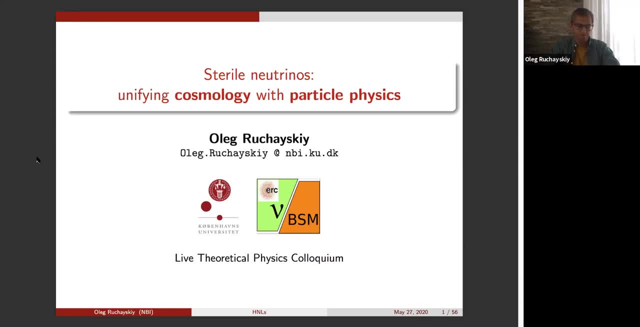 on which I've worked for many years, for more than a decade, And it goes under the name of Stellar Neutrinos And it has an ambition to be a unifying theory between particle physics and cosmology. So, to tell the story in somewhat narrative fashion, let me start from once upon a time. 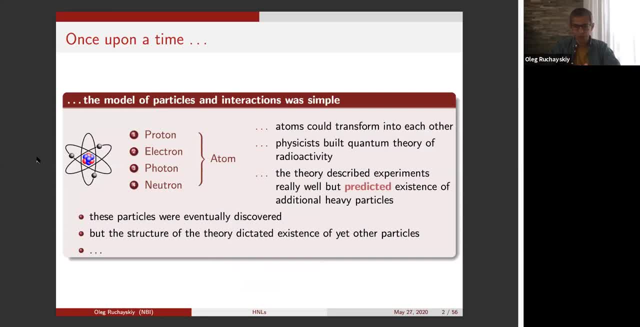 So there used to be a time when particle physics was very simple: There were three particles, one interaction. It was seemingly enough to describe atoms, And if it were not for the reactivity of the atoms, the story would be over at the beginning of the 20th century. 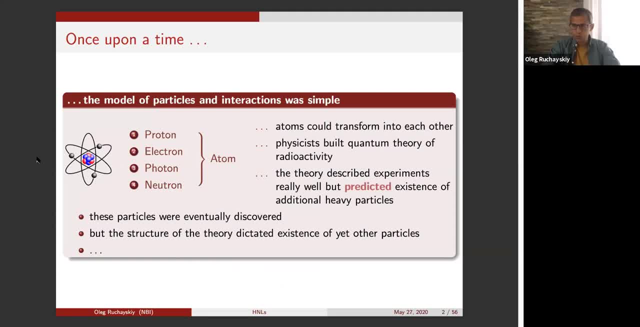 However, the attempts to understand what reactivity is led to the idea that new particles should exist. These particles were predicted, These particles were searched for, These particles were discovered And, fast forward half a century. people are trying to make sense for those particles which appear. 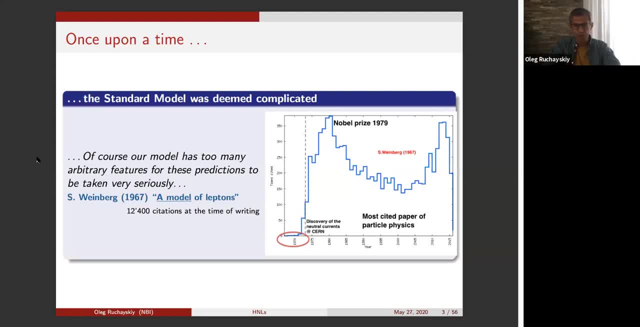 that are predicted, And in some moment. Steven Weinberg, writing the most cited paper of particle physics, writes in this paper: Of course, the model has too many arbitrary features for this prediction to be taken very seriously, So he puts forward an idea of how to unify this whole story. 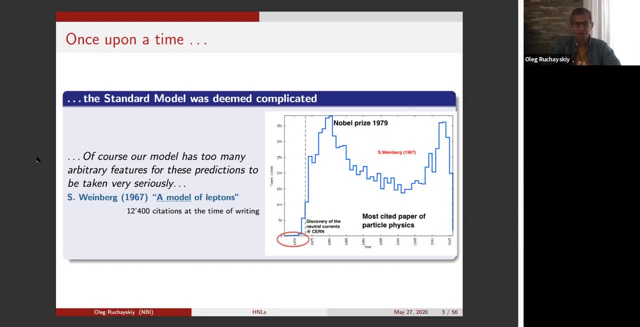 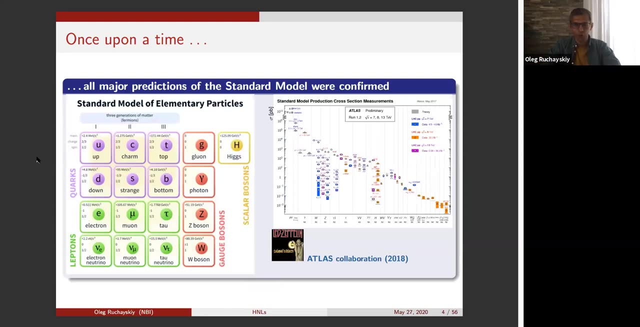 Yet he is puzzled by the fact of how complex and unexpected these things are. And so another half century forward and we are in a situation when this model has too many arbitrary parameters to be taken seriously, is called the Standard Model of Elementary Particles. 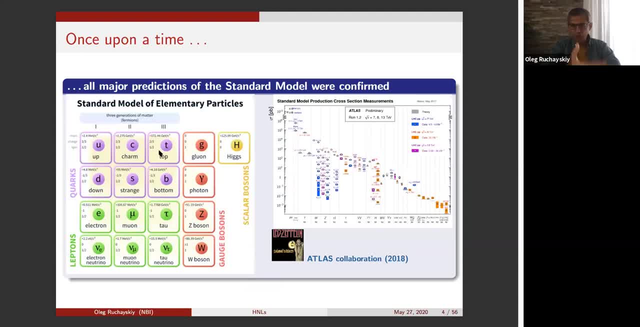 It contains 17 particles And, with LHC finishing two rounds, it produces a beautiful result which many of you have seen probably. It's a number of various predictions, various production of decay channels on the x-axis and cross-section of these events. 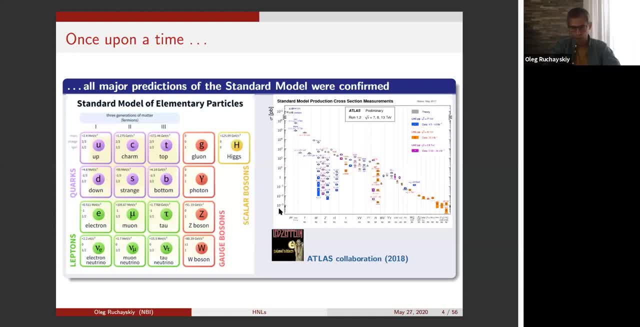 And there are kind of two striking features of this plot. That's why it's called Stairway to Heaven. First of all, between the smallest and largest numbers there are 14 orders of magnitude, So we can have predictions which are running. 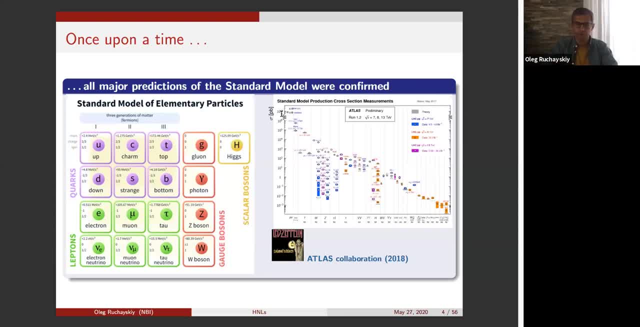 over such a vast decay. So the event which happens once at this end happens a hundred billion trillion times here. And another thing is that on this plot there are theoretical predictions that are in gray and experimental confirmations that are in color. And when you see this plot, 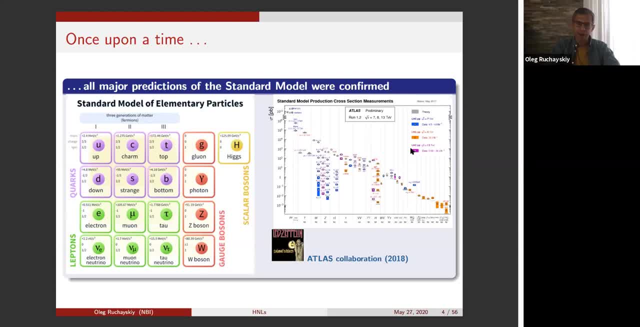 even if I zoom in the full screen, most of the time you don't see the difference, Which shows you how exact our predictions are as of today- And that's a very striking success of the Standard Model and today all the major predictions. 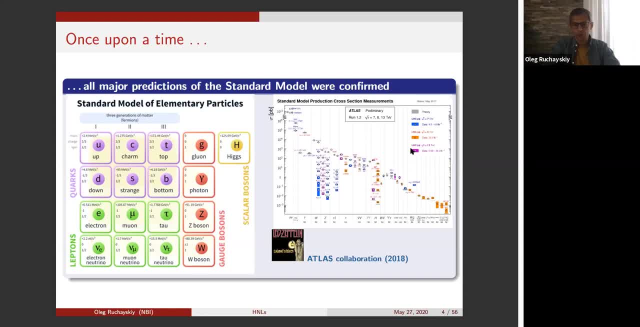 all the particles predicted for the Standard Model have been finally found, with Higgs being one of such particles, And you may say that we finally, in 2012, we finally closed the theory of beta decay, which started in 1920s and 1930s. 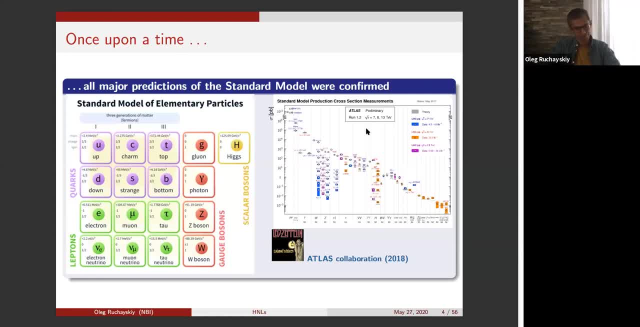 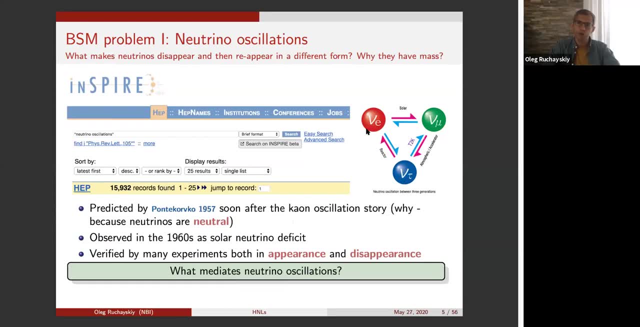 However, along these lines, we also find out that some of the phenomena which we observed in nature do not find their explanations within the Standard Model, And they are known as beyond the Standard Model or BSM phenomena. And let me say very briefly about them. 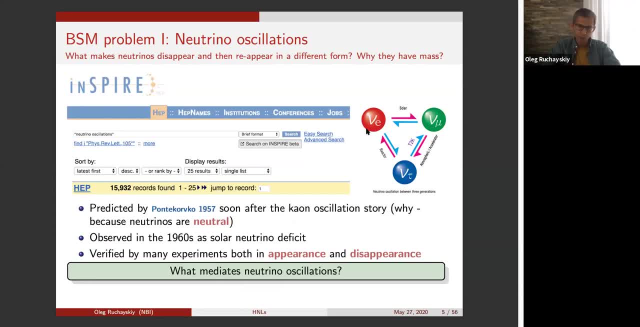 because I will be presenting for you an idea of how to address them. So the first idea is the story of neutrino masses and installations. Unlike other leptons, neutrinos change their flavors And unlike all other particles, they are massive, but we don't know what their mass is. 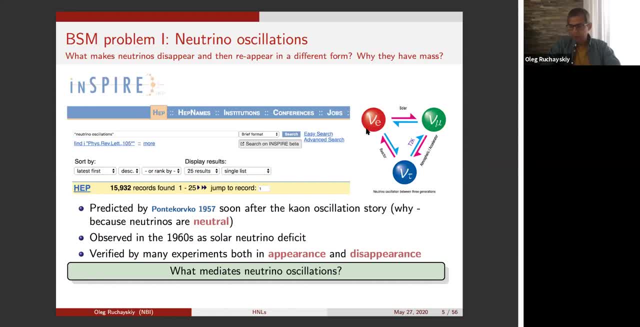 And if you try to think about this- and again I will speak in more details about this- you will see that neutrino installations and mediation of neutrino installations is most probably a fact that more particles, new particles, should exist, And we don't know what these particles are. 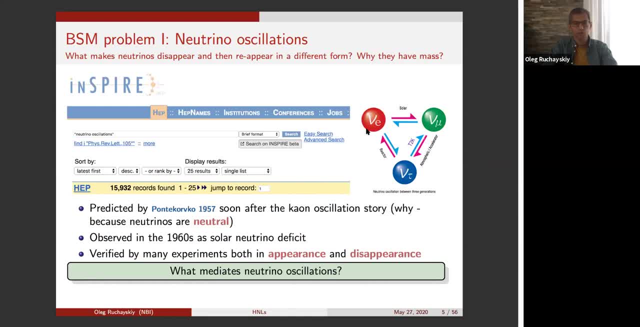 And there is a huge community of people working on this- thousands, of, tens of thousands of papers written on the subject And the Standard Model neutrinos are massless and don't oscillate. The BSM problem number two is not a particle physics problem. 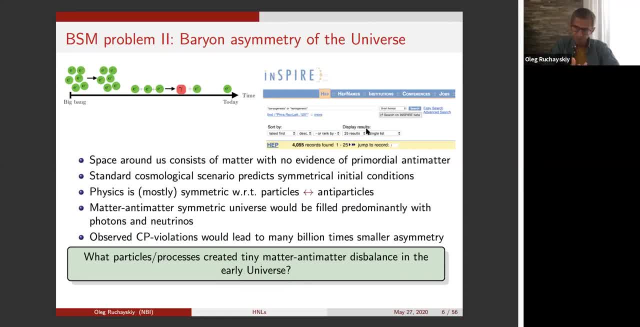 it's an interface of particle physics and cosmology. When people tried to apply laws of physics to the universe as a whole, they were extremely successful with this. The whole Big Bang series, the idea of expanding the universe, the predictions of cosmic microwave- background: 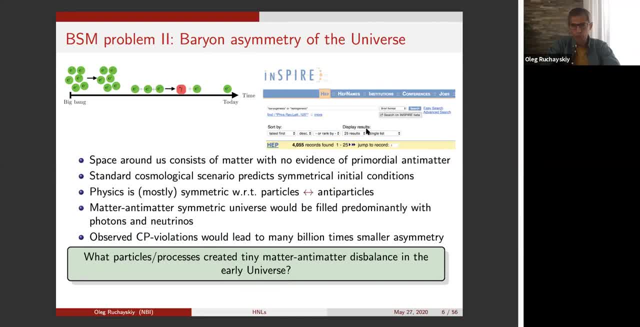 of primordial abundances came from this daring attempt to say, okay, the laws of nature are the same everywhere in the universe. And with this attempt- again very successful, with many predictions which were confirmed- people also noticed that the universe has matter. 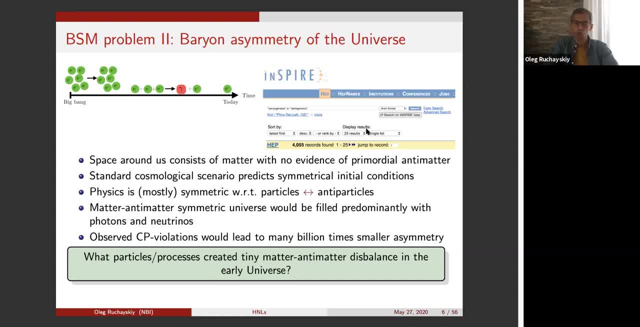 but has no primordial antimatter. All the antimatter we see in the cosmic rays is consistent with being secondary And the equation: from where did the I mean for the antimatter to be absent in the universe? this means that somewhere in the early times. 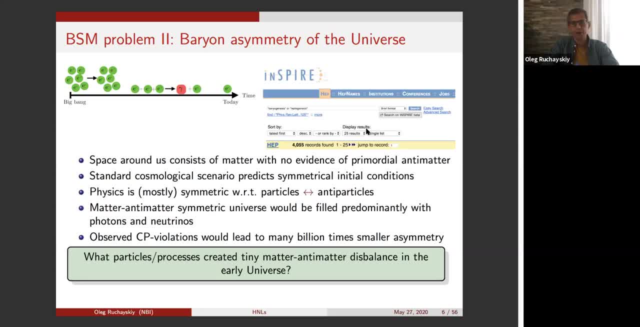 when the universe was hot in length. some of the particles and antiparticles should be unbalanced. You should have one billion more particles than antiparticles. And when everything annihilates, you are left with an excess And we are made of the success. 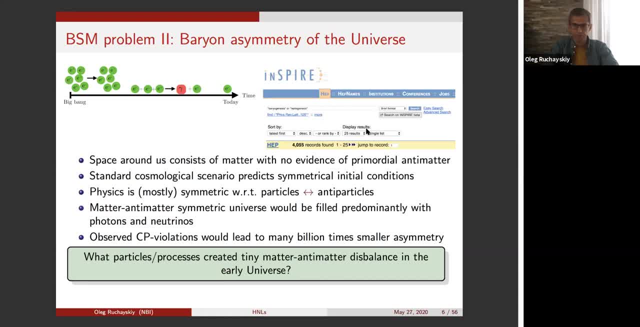 Stars are made of the success and more or less all matter is made of the success, And we know that physics, up to small CP violations, is matter-antimatter symmetric, And so this is something due to some particles, maybe due to some. 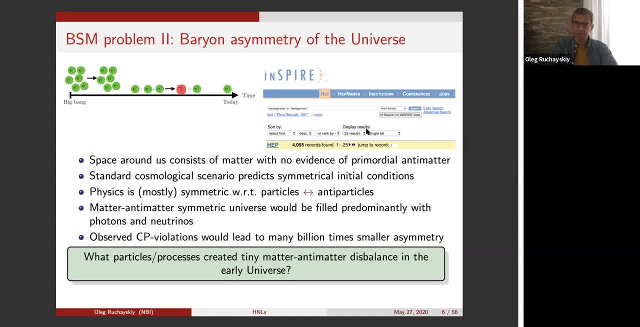 non-equilibrium processes which created this small asymmetry, And this something is not a part of the Standard Model. This can be discussed if you desire, But the short answer is: within a Standard Model, you would not be able to account for such a large. 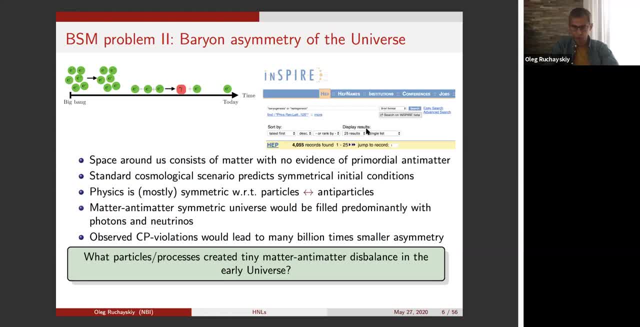 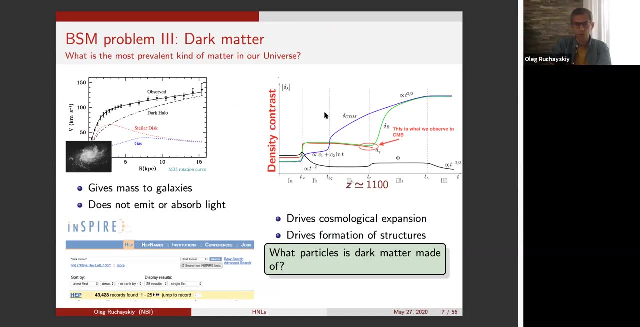 material asymmetry as we see today, And so new particles are needed to explain what causes this. The basic problem number three is a dark matter problem, The fact that you see, through various tracers, much more matter than you can observe. There is much more. 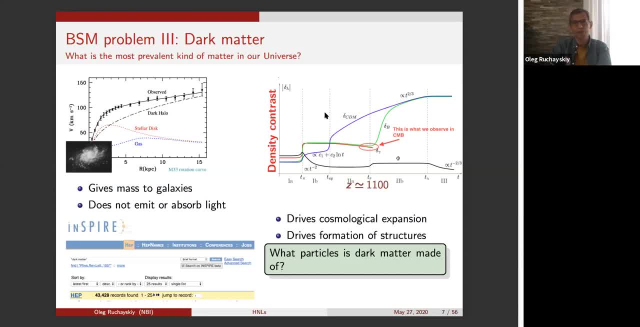 gravitating matter than you can observe from matter that emits light or other detectable radiation, And this is. there are many phenomena which are called dark matter. It's not an experiment, it's not an observation. There are phenomena which explain how that demonstrate for you that. 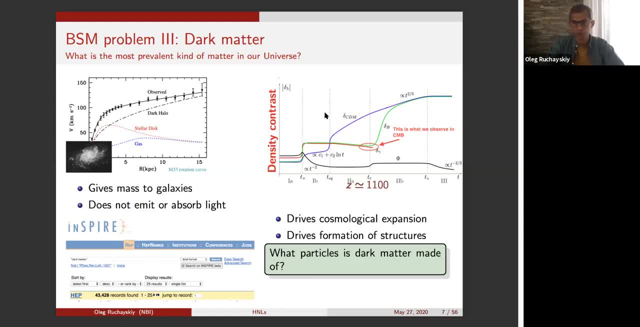 galaxies have more mass than we can account for, that clusters of galaxies have more mass. The whole cosmology sits on the fact that there is some substance in the universe which drives its expansion, yet it is not coupled to photons around the redshift of 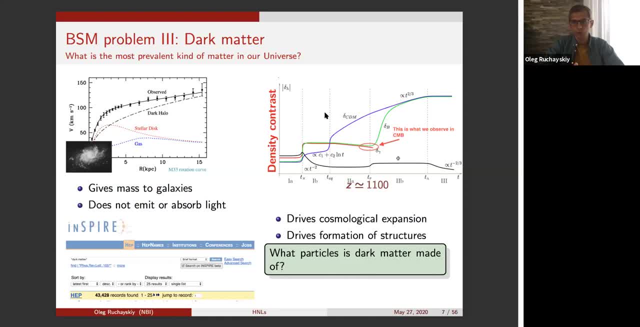 glass scattering. So all this together is known as dark matter, And most probably it's like the dominant hypothesis that this is a particle. And what is this particle? We don't know, And so there are many attempts like this snapshot from the recent INSPIRE search: 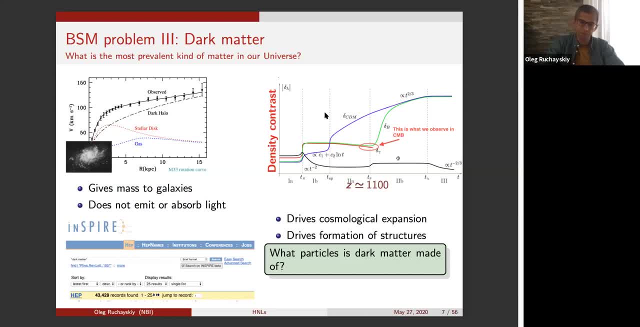 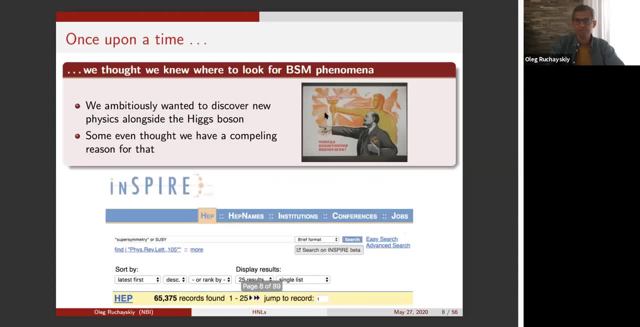 many papers which address this problem discuss various aspects of it. And again, there used to be times prior to the start of the LHC when people thought they knew what the answer was. There were several prominent frameworks which would say that, together with the Higgs, 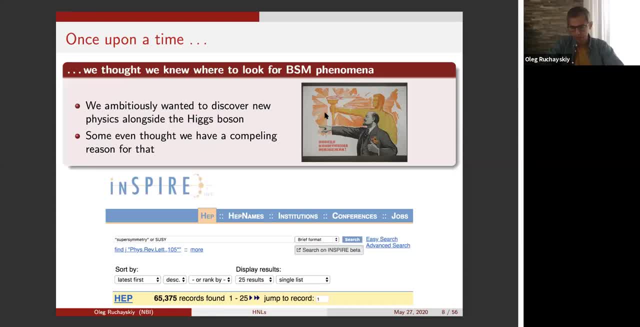 boson. at the electroweak scale we will see many particles And this framework was rich and prolific and all the phenomena which I discussed now could have been embedded into this framework. It's supersymmetry, some other electroweak scale. 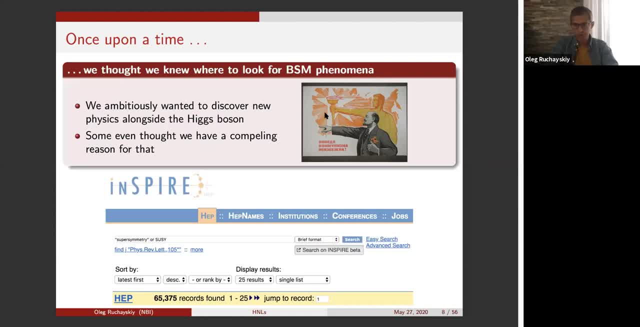 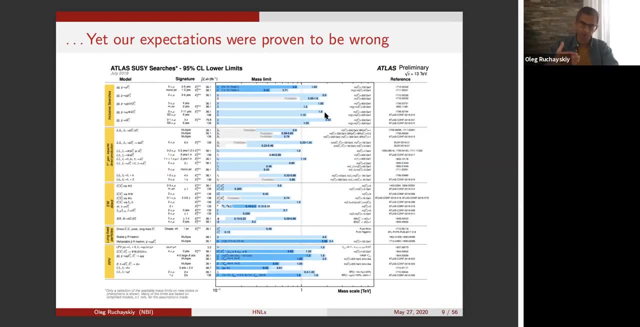 new physics and it didn't show up at the LHC. The state of the art today is that you see a lot of exclusions. various models, various channels are probed to TV scale and yet there are no evidence for any of this electroweak scale physics. 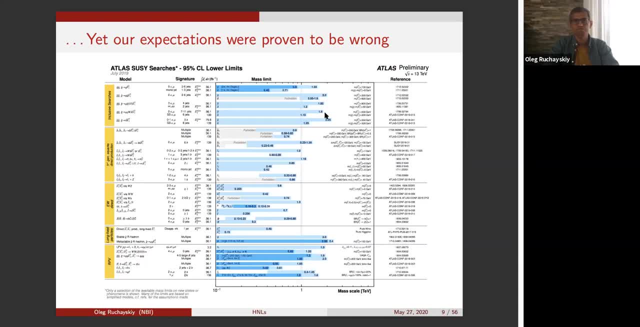 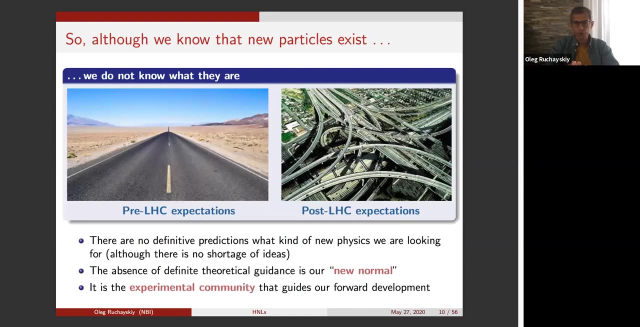 And so this framework is maybe not gone, but challenged, And people became very much open to new ideas. Paraphrasing one of the theorists from CERN: prior to the LHC, the community felt they knew what the road is to new physics. 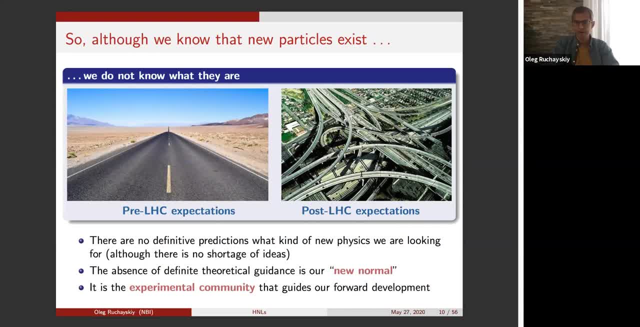 And today we are somewhere. here. There is a land of ideas, land of opportunities, if you wish, and they are all of the same footing. There is no prior, there is no bias, apart from your personal interest. So it's a very interesting time in physics. 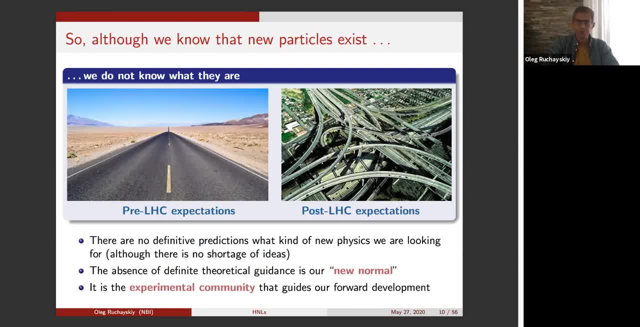 when everything is allowed and when it's not a theory which drives the development of the field, but rather the experiment. We all wait for what new experiments will show to us, And that's an interesting time, challenging time and for me being a phenomenologist. 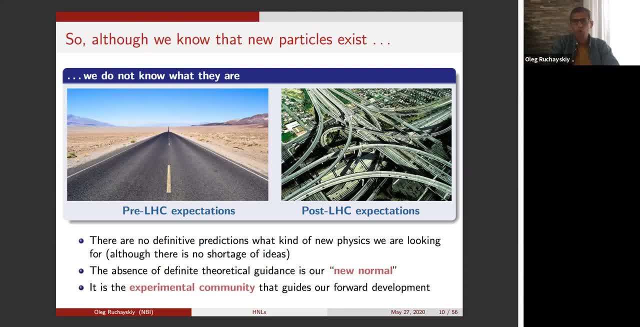 a theorist, it's a time when I choose a model based on my taste, preference, intuition, and I work on it because trying to see whether it survives the observations which we have in the future. And so this is a model which 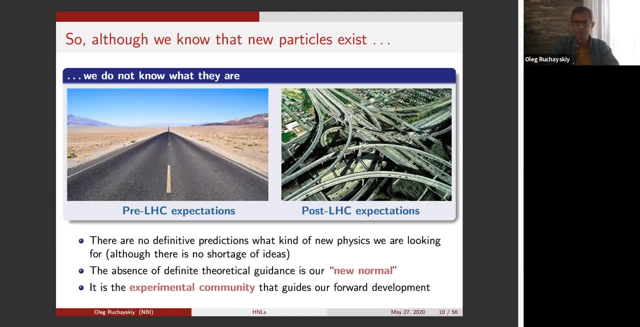 I want to talk to you about. So, in this state of affairs, the question is: which road do I take? Again, it's a personal take. I don't want to make an impression that this is the model or that I don't believe that. 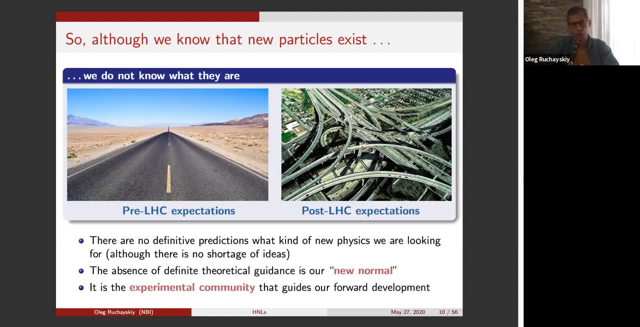 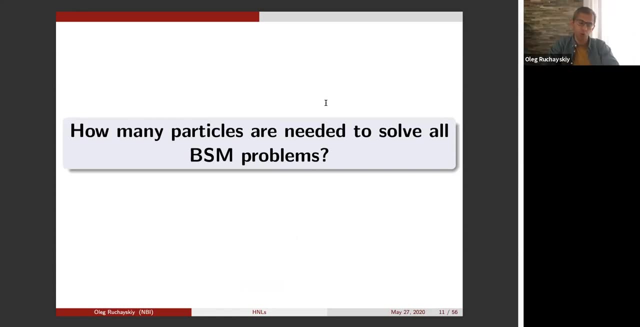 anything else is possible, but again, at some moment you have to decide what you are working on. That's my choice and I hope I will convince you that you are. So let me, given that we have at least three Bionsen-Rothmose problems, 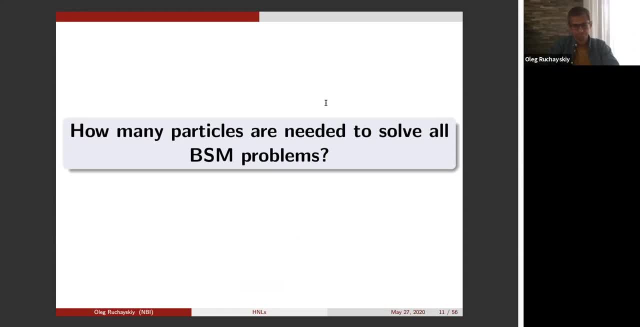 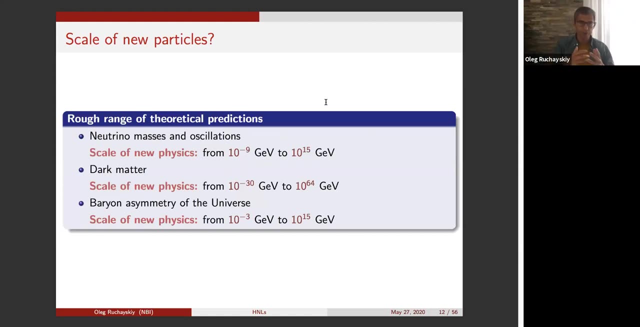 what would be the minimum number of particles that you need to identify to resolve these problems? Well, let's start from the question here. In the landscape of theoretical ideas, do we have any indication as to where to go, which scale to choose? 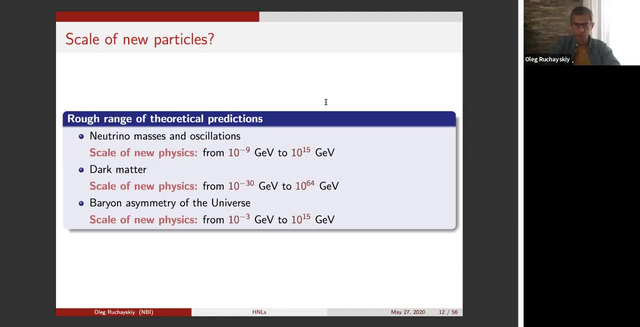 The answer is no. The scales are enormous, from tiny electron-volts or even sub-electron-volts in case of dark matter scales to n, to the 15 GeV, to the scales which are well beyond the reach of current. 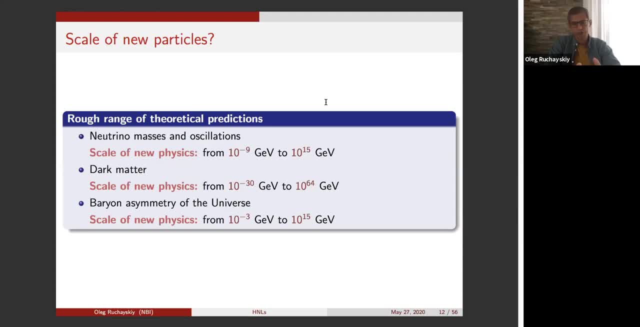 or any foreseeable experiments. So you cannot say let's explore this because this is a preferred place or we don't know. And this vast range of scales, field of scales, it's very well indicated by the story of neutrino oscillations. 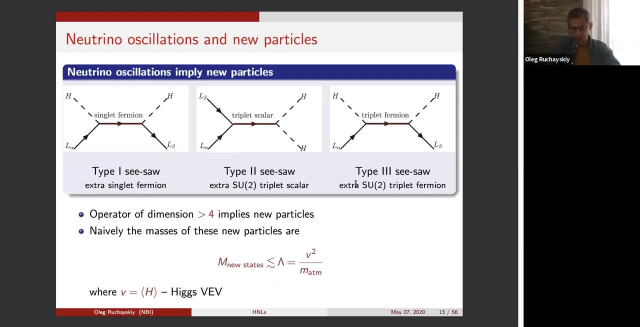 So the fact that neutrino oscillate? what's neutrino? We know that the weak and electromagnetic forces are united into the electroweak symmetry and, in the unbroken phase, the electron and neutrino are two components of the same doublet. 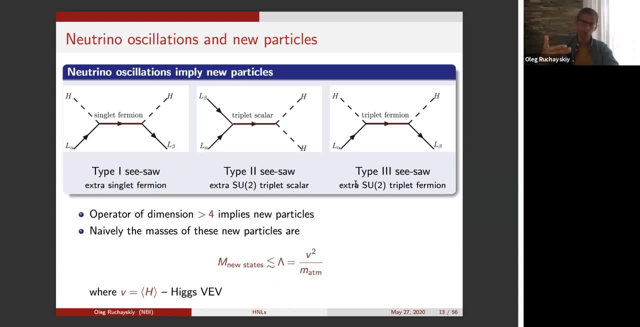 and so you can rotate one into another. And it is a Higgs which, when it breaks the electroweak symmetry to weak and electric, it actually tells you which of the two components of the doublet is electron and which one is neutrino. 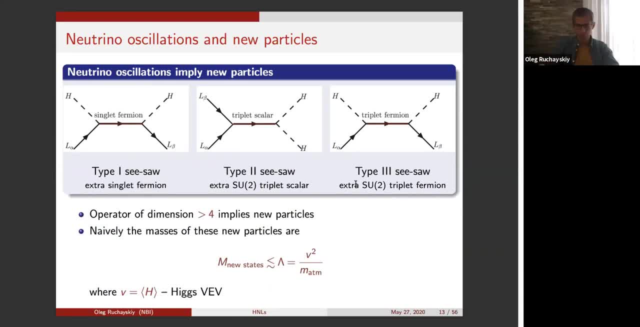 And so the interaction between neutrino masses and neutrino oscillations are actually an interaction between four particles, two lepton doublets and two Higgs bosons, And there are many ways to resolve this kind. this is a high dimension, dimension 5 operator. 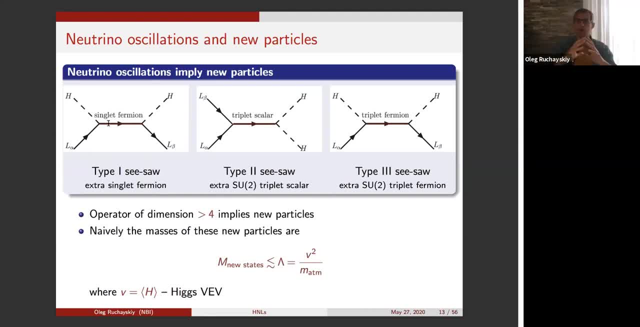 and there are many ways to resolve this dimension 5 operator: by introducing an extra particle which mediates it. It can be fermion, it can be scalar, it can be uncharged scalar, it can be charged scalar. and if you just look at the scale of this, 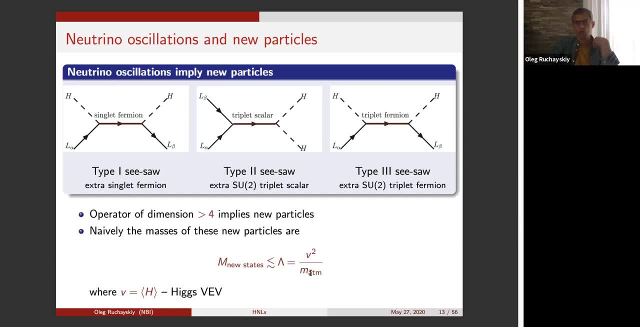 which is just mass of square root of atmospheric neutrino. mass difference divided by the Higgs wave, you will see a scale which is of 10 to the 15 GeV And therefore the first idea of a resolution of neutrino oscillation puzzle. 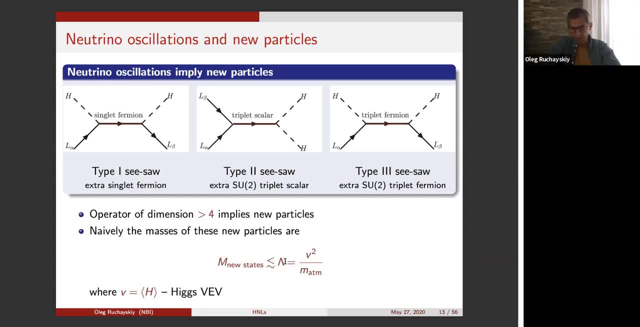 was with a very heavy extra neutrino, But then people understood that actually there is no. this is a scale, but it's not a mass of the particle. There is no one-to-one correspondence. It's a very much extent not so. 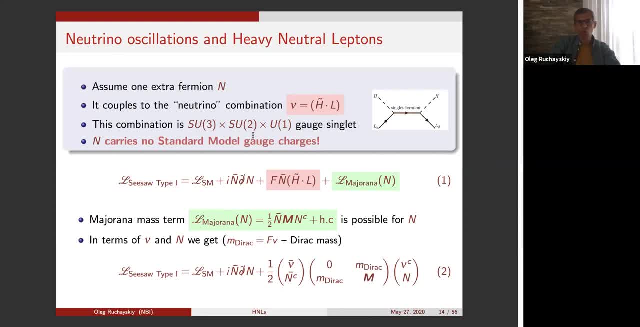 If you look at this in more details, here's your dimension 5 operator, resolved with a singlet fermion. The fact that it is singlet means non-charged with respect to the strong, weak or electromagnetic field, is dictated to you by the charges. 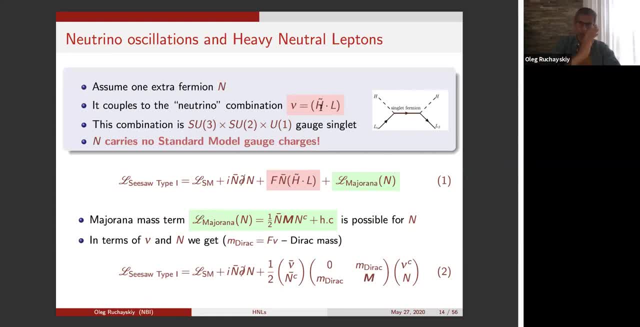 of the lab doublet and of the Higgs, which chooses for you what is neutrino. as I said, And given that it is singlet, you can not only couple it to the Higgs and to the left-handed neutrinos through usual Dirac interaction. 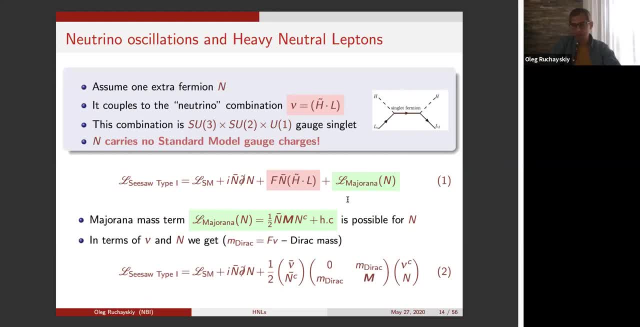 but you can also write for it: the Majorana master. The idea of Vittorio Majorana, which introduced, inserted this to give mass to actual neutrinos, came back to us half century later, because then people understood that this is a truly neutral particle. 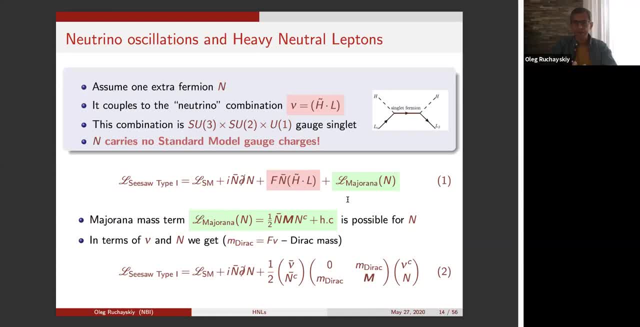 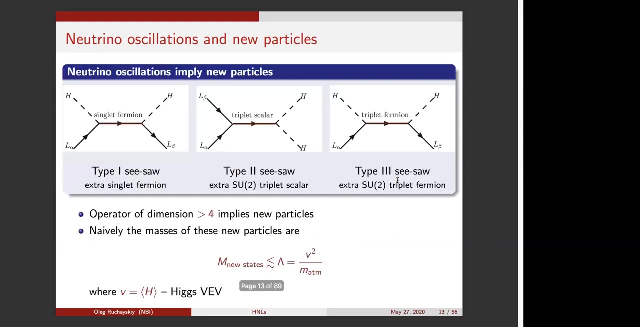 and only true neutral particle can have Majorana mass, because this Majorana mass violates any continuous symmetry. And so you have. Yes, Somebody has a question? Yes, go ahead, Thank you. So can I ask: where can I see the triplet fermion in type III C cell? 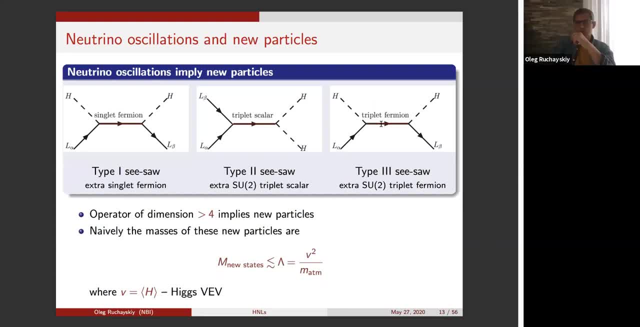 I don't see any triplet fermion there. The triplet fermion is here. So what you have? you have a triplet. this is the SU triplet. So you have an SU triplet and two SU doubles. You can think about the SU triplet. 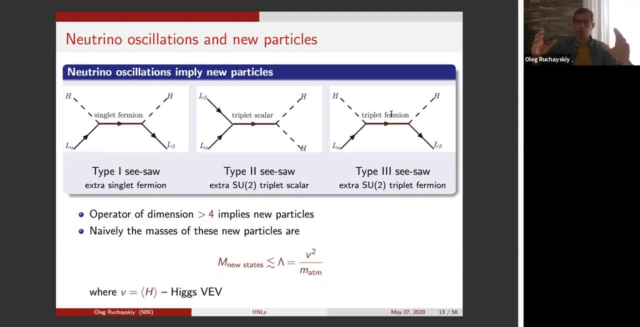 as the joint matrix, and so you have two two-dimensional vectors and one matrix which couples them. Okay, Sorry, can I? can you explain the difference between the triplet scalar in type II C cell? So the triplet is inside the propagator? Yes, they're always inside. 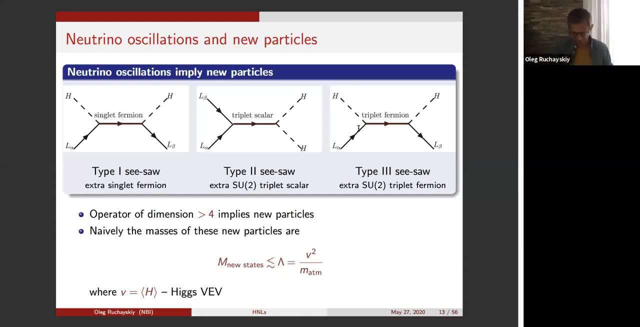 the propagator, but their mass is different, Their statistics is different and if you try to, if you would try to write, to write the mass term, you need to ensure that you build a scalar and you need to ensure that you build scalar in terms of the Lorentz. 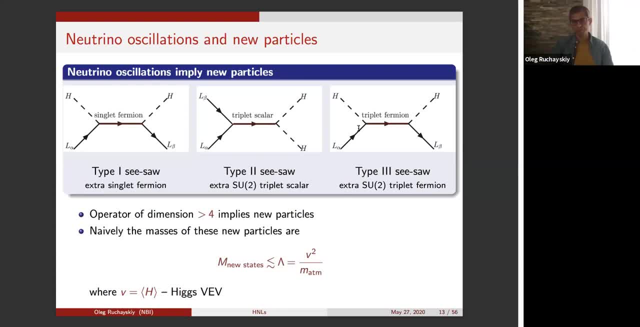 transformation and scalar. in terms of the SU transformation, Okay, I see, And so you have triplet for the SU, and then you need two Fermions, one scalar, And so these and these are two different choices, I see, Or you can combine SU triplet. 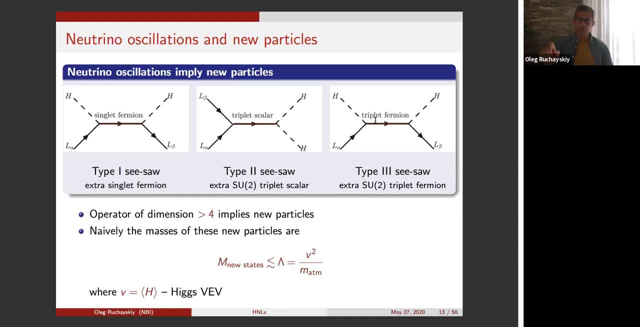 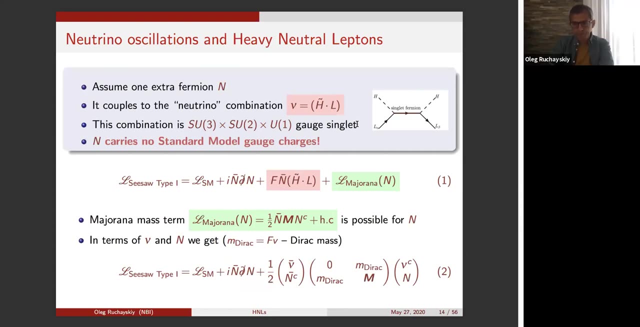 Again, you can think about this as a Pauli matrices times three, Fermions, scalars, Pauli in the Isospin, in the SU space. Okay, Okay, Okay, thank you. Okay so, but coming back to the CISO type one, 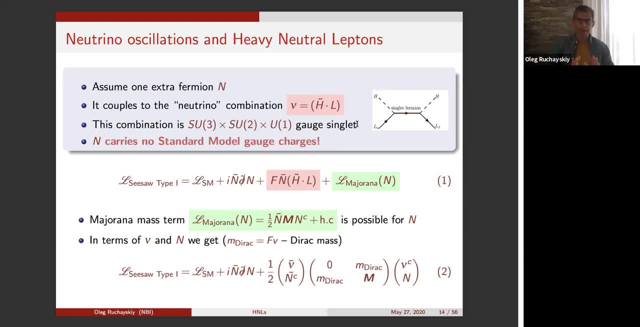 where this Fermion is single, which seems to be again, it's not. as you see, there are many choices in which one brings its own observers and its own ways to probe it and its own predictions. So even in this naively simplest, 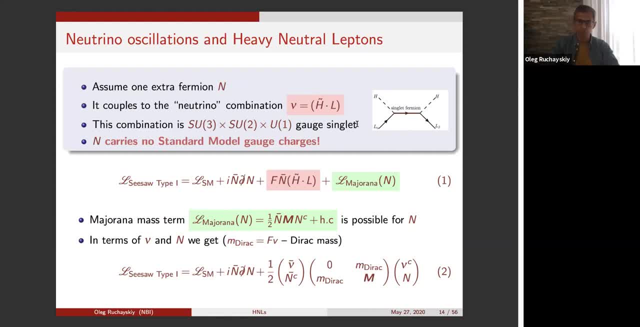 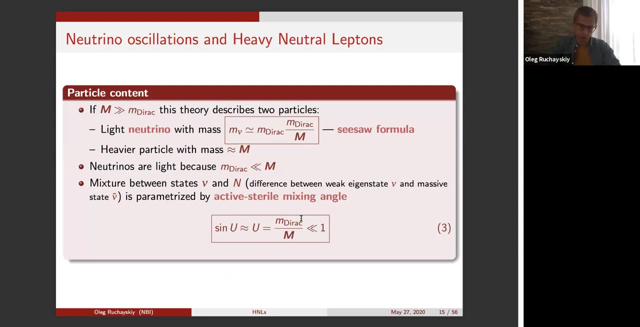 model. you will see, the is very rich. So what happens here? You have a particle which is charged, which carries no charge- Dirac mass and Majoran mass- And there is a philosophical question of what you call a particle. And is particle something? 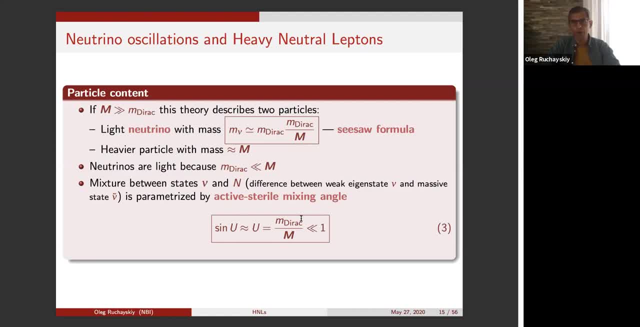 that propagates in a definite way, Or is particle something that interacts in a definite way? And very often for photons, electrodes, etc. you don't have to worry about this question because they coincide: The one who propagates and the one who interacts. 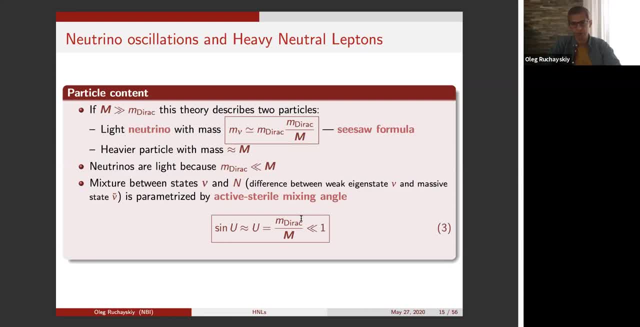 Here this is not the case. There is a charge state which I just described. It has zero charges, but it doesn't propagate. This state by itself does not obey the Klein-Gordon equation or Dirac equation, of which the Klein-Gordon is a consequence. 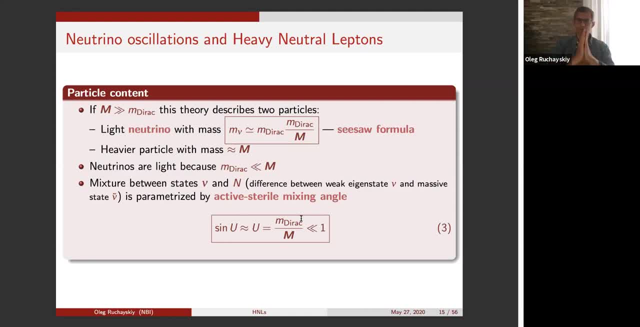 But you can diagonalize it, defining definite propagation states, mass eigenstates, In which case you will see that your theory contains actually two particles Light but not massless fermion, which is not its charge eigenstate, and therefore there are oscillations. 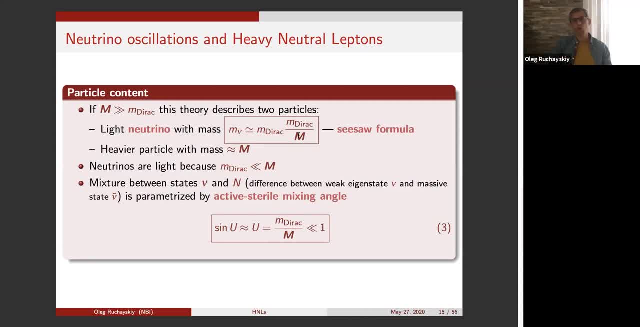 And also heavy. if your mass of your right-handed component of your singlet fermion is much bigger than the Dirac mass Which carries some charges, I will show you. And because of this formula, mass of neutrinos is Dirac mass times the ratio. 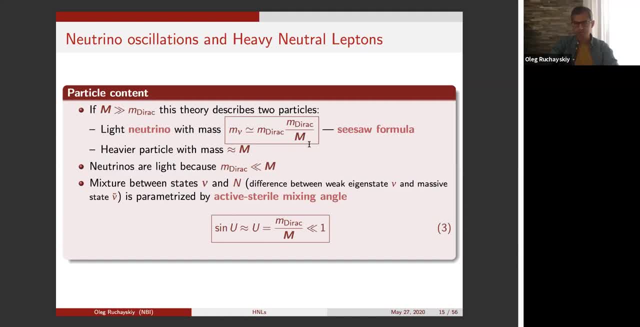 you see that you can change both Dirac and Majorana mass and getting the same neutrino mass. And this mass may be of electroweak scale, in which case the denominator will be 10 to the 15 GeV, Whereas this mass can be. 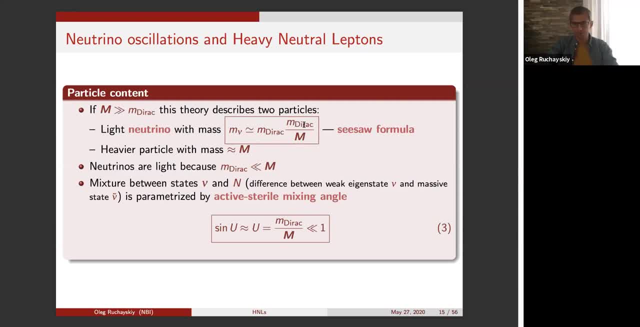 of some sub-electron world, in which case this will be tiny And there can be anything in between. So that's why I say that neutrino masses do not predict a scale and can be from electron worlds to 10 to the 15 GeV. 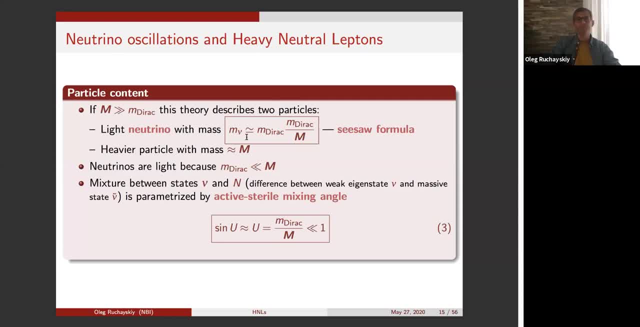 But what's important is that there are two particles here and there is Majorana mass of neutrinos- There's always phenomenology, neutrinos, etc. And there's also another particle, And if I define the dimensionless number which is called mixing angle, 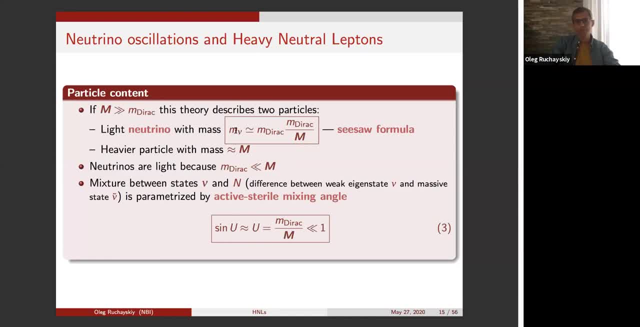 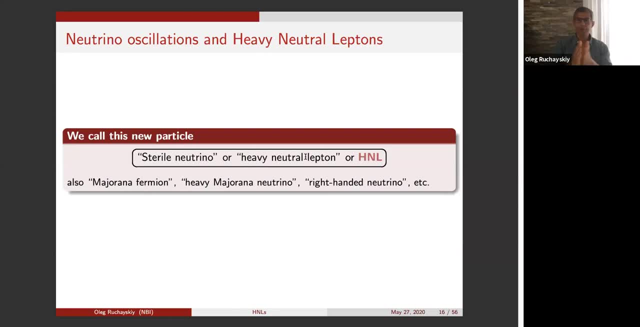 which is Dirac over Majorana mass or, if you wish, which is mass of the neutrino over this Dirac mass, then this propagating state is usually called sterile neutrino or heavy neutral lepton, HNL, or Majorana fermion. 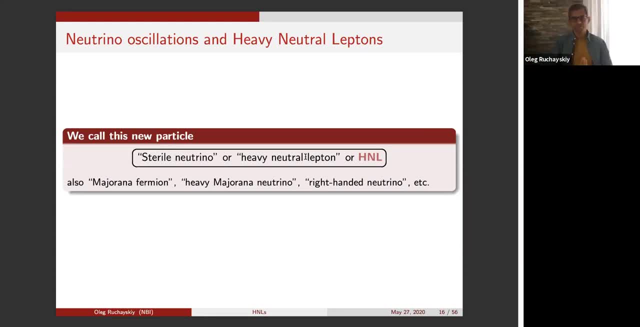 or heavy Majorana, fermion or right-handed neutrino. There are many names and, depending on which branch of particle physics you are sitting, different names are considered more standard. But what's important about it? it's a heavy neutral lepton. 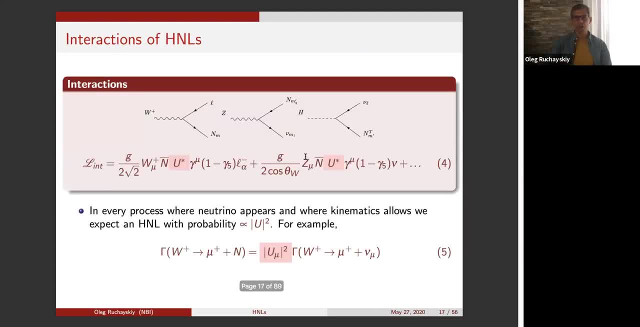 it's a heavy cousin of a neutrino. it behaves like a neutrino, it interacts. if I speak about mass eigenstate, again there is a charge. eigenstate which is sterile doesn't interact, but it mixes with neutrino. 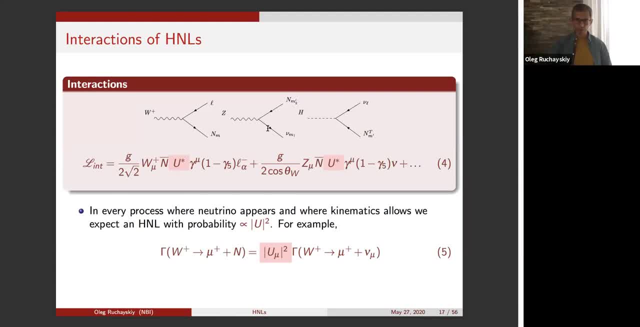 or there is mass eigenstate, which doesn't mix with anything, but it interacts with W, with Z, with Higgs, and it interacts in a way similar to the way neutrinos interact, but with a weak coupling constant suppressed by some small, dimensionless number. 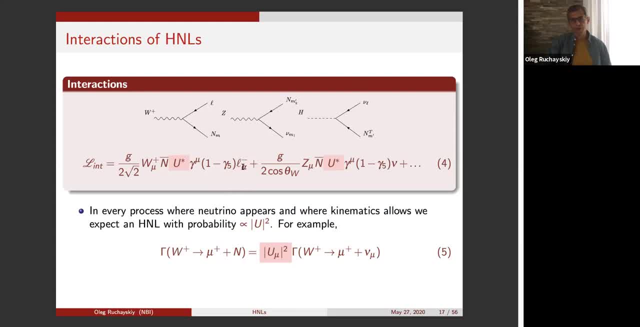 which is actually flavor dependent. I forgot to put flavor in this here, but it's electron, mu and tau, so there are three mixes here. So it's the type I Sasson the introduction of a singlet right-handed fermion into the Lagrangian. 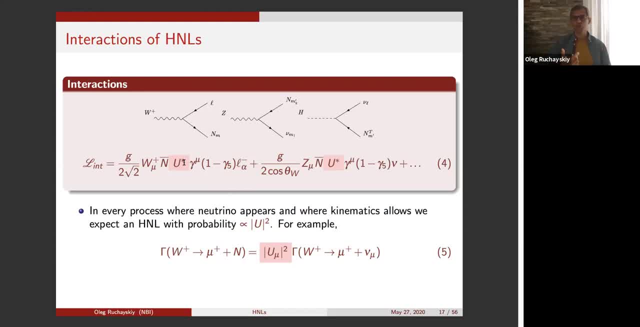 leads phenomenologically to the appearance of new particles whose mass is a free parameter in your theory and whose interaction strength is free parameter in your theory, because it's weak-like but suppressed. so sometimes we call it feebly interacting particles or super-weakly interacting particles. 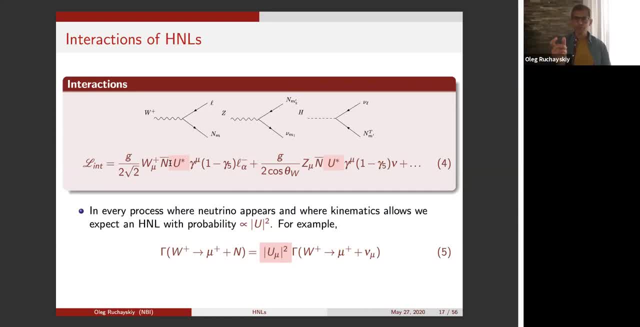 And this is phenomenology- is in a sense very simple. It participates in all the interactions, in all the reactions in which usual neutrino would participate if kinematics allowed, and it's their interaction is suppressed by this number, by the mixing angle. 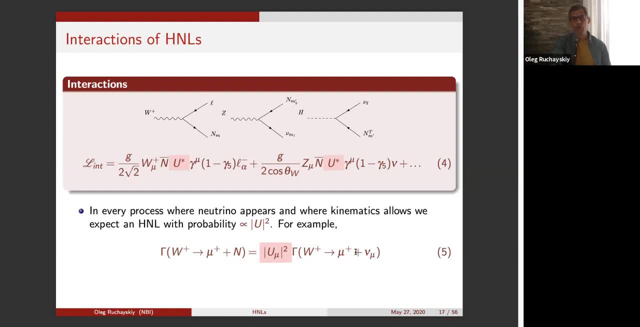 So, for example, W decays to muon neutrino, or it can decay to the muon and sterile neutrino to the H now, and the decay which to the heavy is suppressed by square of the mixing angle, provided that the 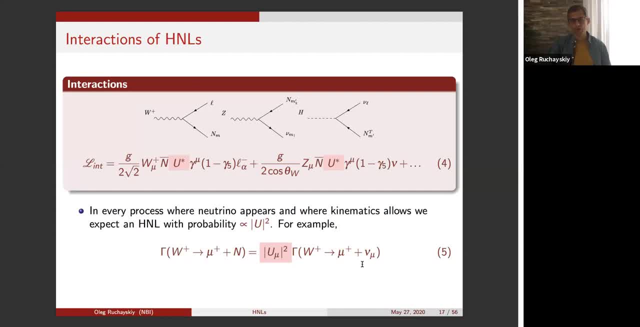 mass of H now is much smaller than the mass of the W, otherwise there are corrections due to threshold. So and that's kind of the simplest model of explaining neutrino mass installations And, as I will show you right now, it already brings a very rich 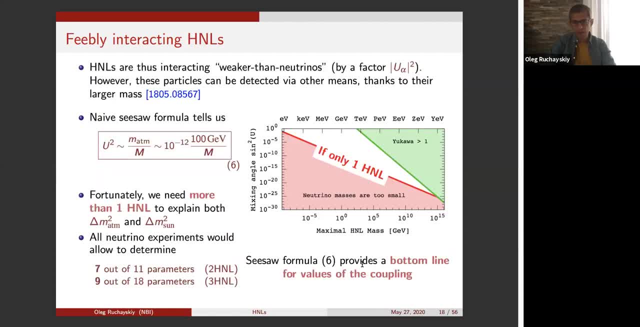 phenomenology, Namely like it's useful to have a feeling for what the level of the mixing is, the mixing angle, how tiny it is, And it's one trillionth, for if your H now has a mass of 100 GV and it scales as one. 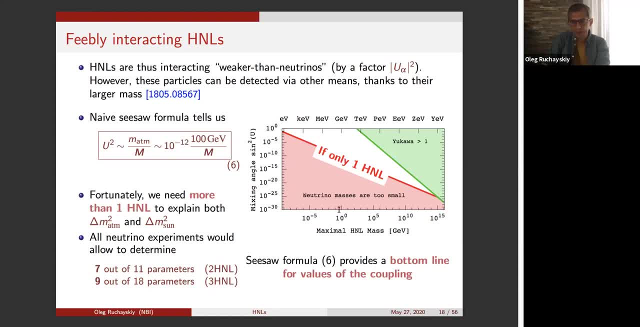 over mass. And if you look at this space of neutrino masses versus mixing angles, then it can be from electron volts to 15 GV. and if there would be only one H now in your theory, you would have this line along which the 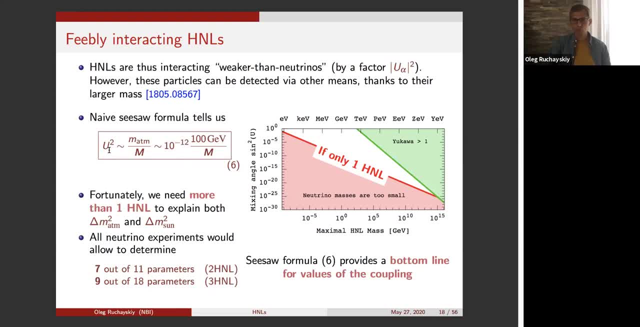 mixing angle follows mass, So you could assume the mass and predict the coupling constant. However, the story is not that simple, because neutrino physics observed two mass splittings, called atmospheric and solar. They are different, but they are both non-zero. 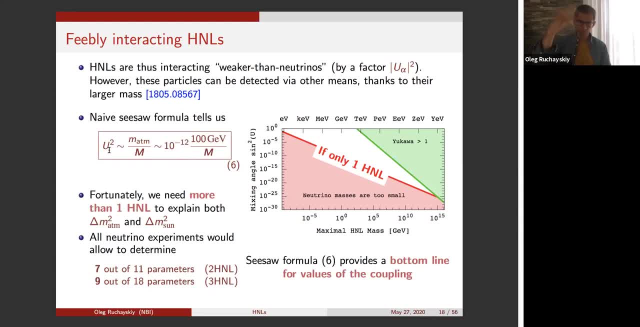 which means that you would need at least two HNLs coupled in the same way. but now you have a matrix of Eucala couplings and a matrix of Majorana masses And you need at least two to explain two mass differences. 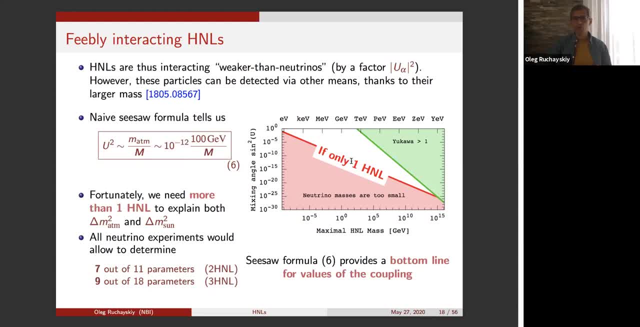 And this fact allows you to open for you this whole wide wedge, this whole wide parameter space. So, from here to up to there, anything is allowed If you have two of them, because there are more parameters in two HNL models. 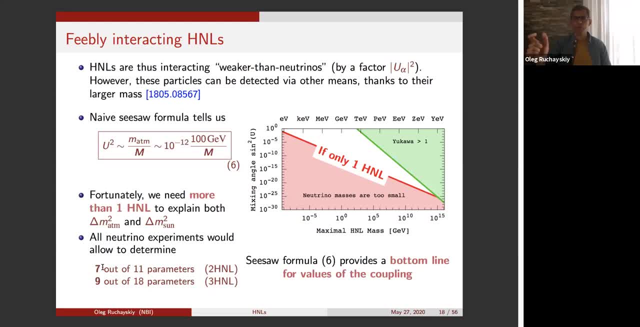 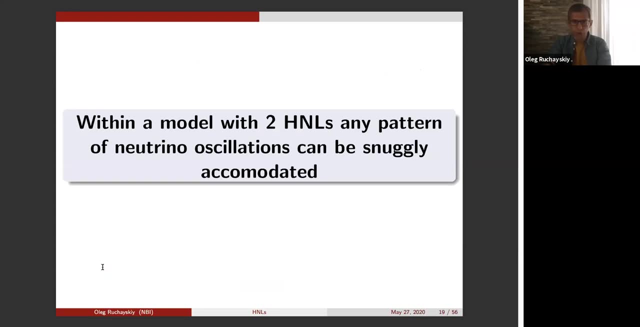 There are 11 parameters and only seven can be restricted from neutrino data, So you have enough freedom to move your interaction strengths up and down. Okay, So two HNLs can snugly accommodate the neutrino oscillations for any. 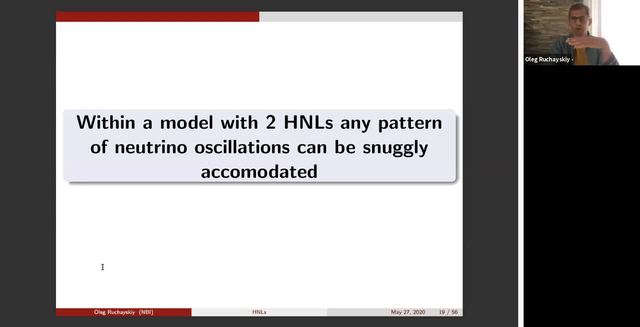 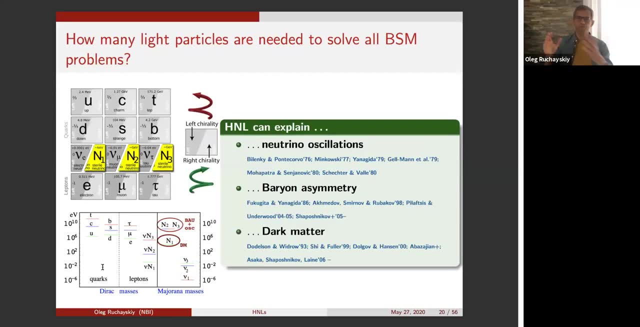 neutrino data, including Cp phase, which is not measured for any neutrino mass order. However, the interesting this idea goes back to late 70s. In 80s people understood that actually the same particles can be responsible for generation of the baron. 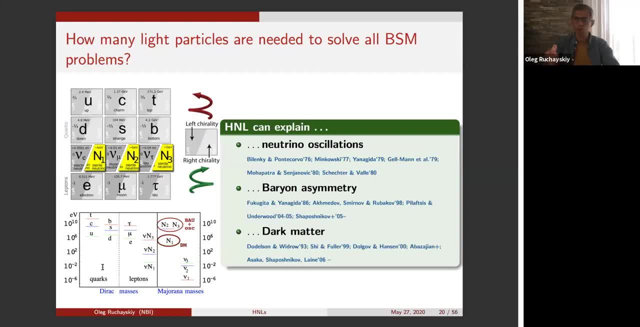 of the universe. In 90s they understood that they can be responsible for generation of the baron of the universe with a mass much smaller than 10 to the 15 GeV At the order of GeV or TeV. there are different models. 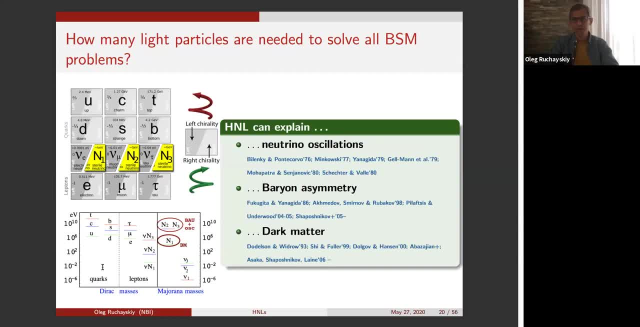 In, also 90s, they understood that light having neutral lattice are responsible for- maybe responsible for- dark matter. I will speak more about this. And 15 years ago, in 2005,, Takiya Saka and Misha Shapochnikov understood that. 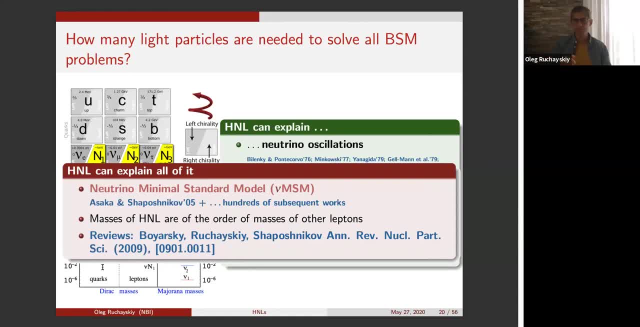 actually, you can combine all of this into one model, And this model will require for you three neutral lattice, Which is nice because you have three left-handed neutrinos and you can add to your model three right-handed neutrinos. By the way, this is not required. 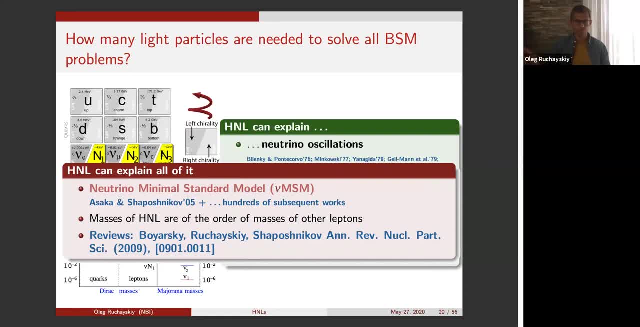 You can add one, two, three, five or seventeen neutrinos to the model and still have all the neutrino phenomenology. Of course there are a lot of free parameters, So the number of right-handed neutrinos don't have to be the same as number of left-handed neutrinos. 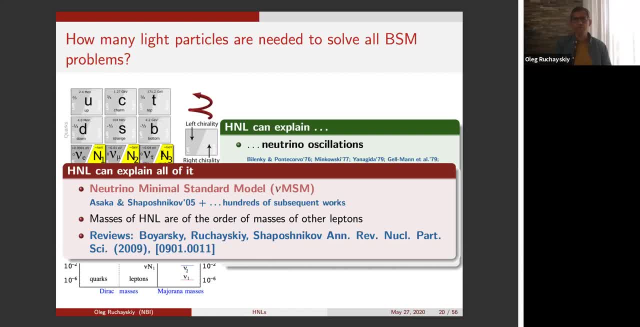 However, if it is surprisingly, you can fit into the same model. choose a parameter in such a way that you can get neutrino mass and oscillation binary asymmetry of the neutrinos and dark matter. This model is called NeuMSM- Neutrino Minimal Standard Model. 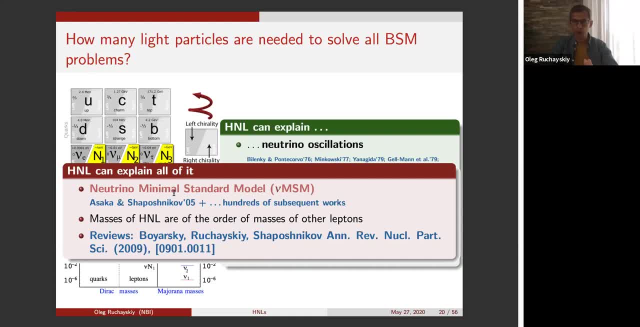 And it is this model which I'm going to talk about later. It's one of the choices of parameters for the type one to solve the singular right-handed neutrino, And that's a very interesting choice of parameters. And already here we still have a lot of freedom. 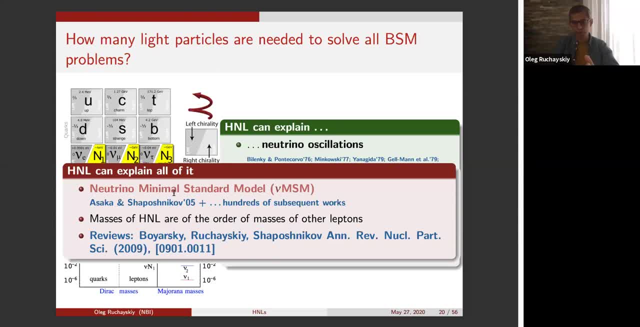 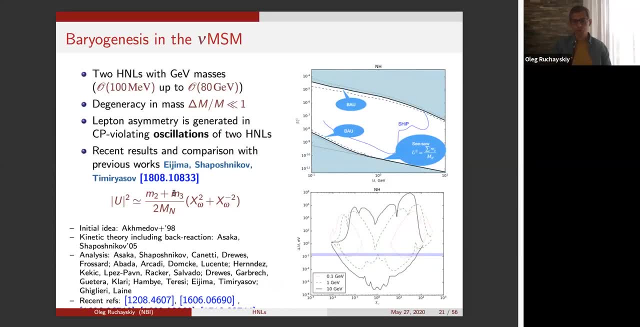 surprisingly, as it is in such a negative constraint model. So let me speak about this a little bit. To produce binary asymmetry of the neutrinos, you should have also two heavy neutral leptons. They can be the same heavy neutral leptons. 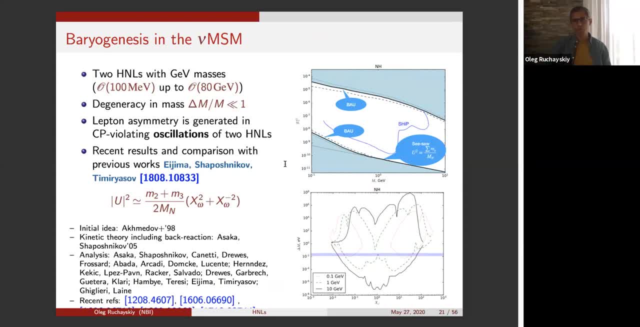 which generate for you neutrino mass and oscillations. So this is their mass and this is their interaction strength, And they should be degenerate in mass, since their mass difference should be much smaller than their mass. How much smaller depends. There is a wide space of parameters. 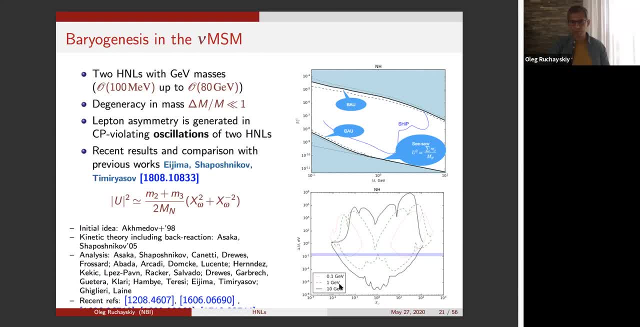 This is delta m for various masses And you see that there are about 10 orders of magnitude. This is the region where you can generate successful binary asymmetry of the neutrinos And this is the area of researching. This is a long list of names. and long list of references. You can look at this paper. It discusses all the previous works, So you can look there and see the comparison. But what you do? essentially you have two HNLs. They almost degenerate in mass. 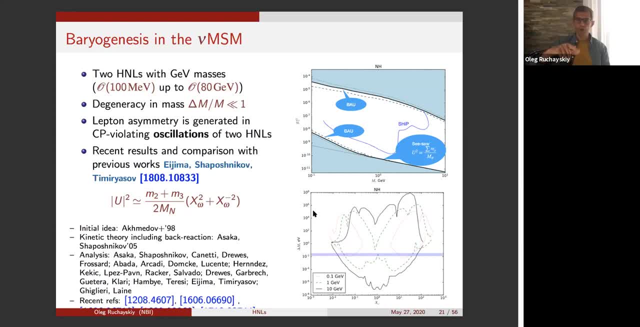 When they oscillate in the early universe, they do it in the CP-violating manner, And in this way they produce leptinous symmetry which then gets transformed into the binary asymmetry. This is the range well accessible to all accelerators. 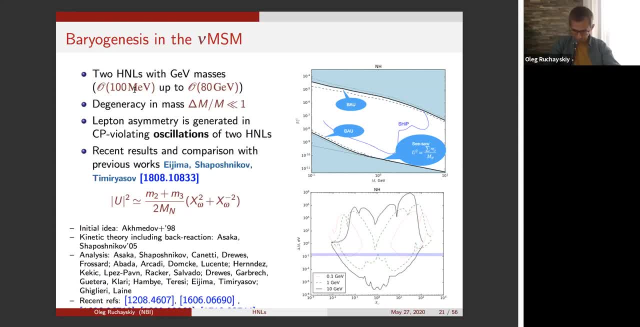 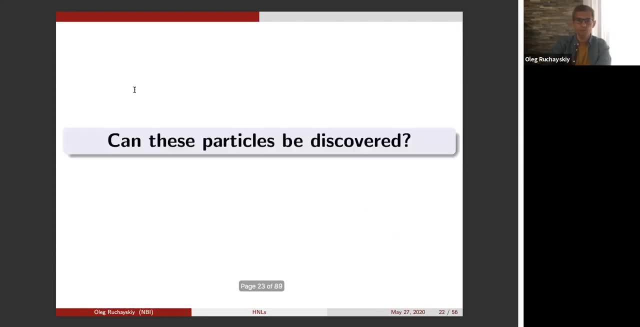 but their interaction strength is very feeble. The question is: can we search for such particles? And let me now discuss where this particle can be searched, and then move to the question of dark matter. So can this particle, this two HNLs with GV-scale masses? 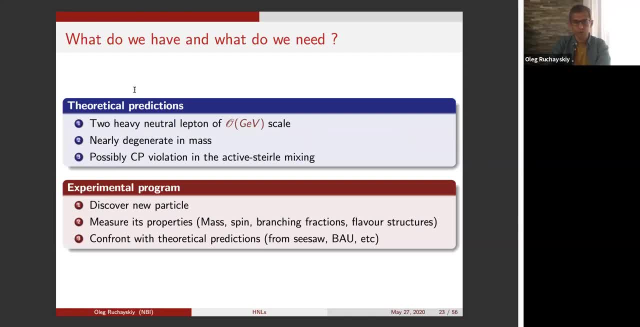 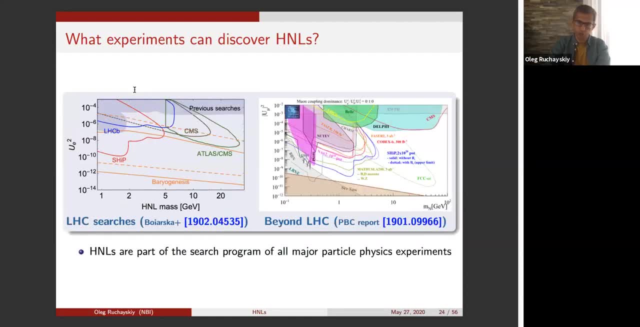 be discovered. So two particles nearly degenerate in mass. How can we do it? Short answer: Yes, they can. They can be discovered in the future rounds of the Large Hadron Collider or at many so-called intensive frontier experiments. And what I show you here? 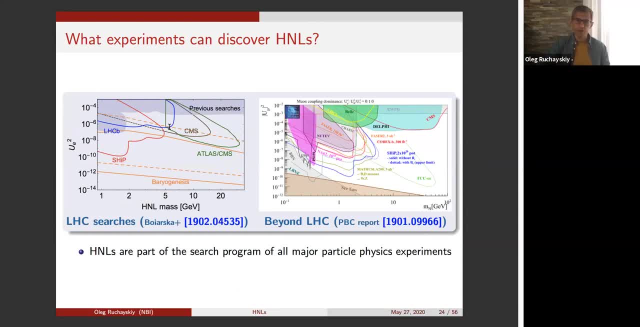 I don't show you any specific details. What I want you to see- all the open contours- are future experiments. These ones are related to the Large Hadron Collider. These ones are related to future non-LHC searches. And the interesting thing here is: 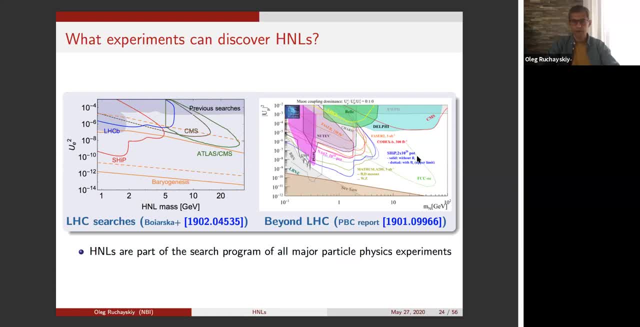 that these are all experiments which are possible. okay, It's not a 10-15 GV collider, It's a future circle collider, a larger version of FLAP, which is challenging but doable. probably You can explore a significant part. 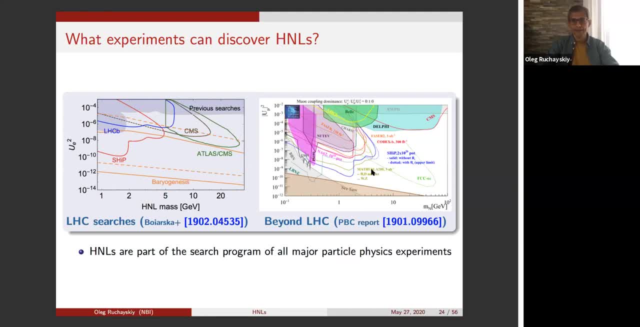 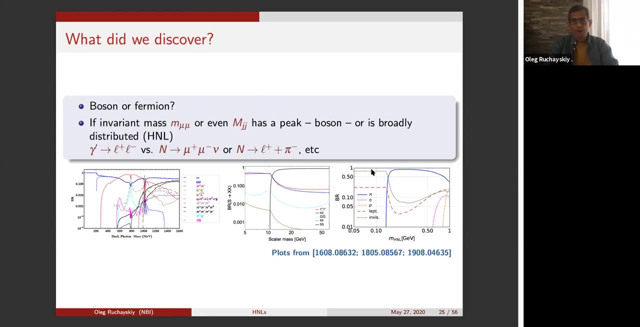 of the parameter space of the heavy neutral lapland model And because of that and because of the interest to this model, HNLs are today the part of the search program for all major particle physics experiments, which is a very interesting and very interesting. 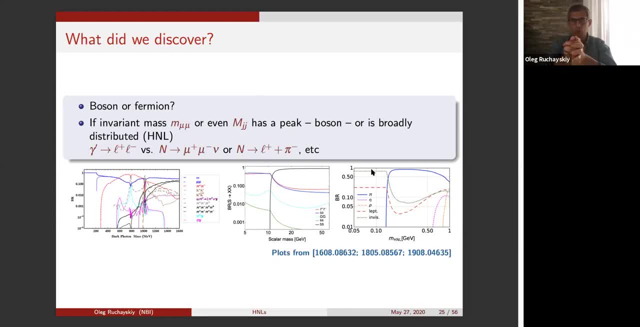 land. When you discover a particle, there is no name tag attached to it. However, if you look at the particle and if you discover sufficiently many events by looking at the various branching ratios of the way it decays to leptons or to leptons plus mesons, 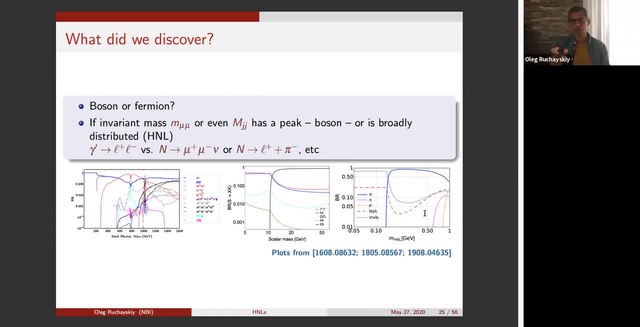 by looking at the ratio of the branching fractions, you can determine whether you discovered a scalar or a fermion. You can restore its mass or see that certain channels have broad distribution. So you can figure out. okay, I discovered a particle. this is a fermion. 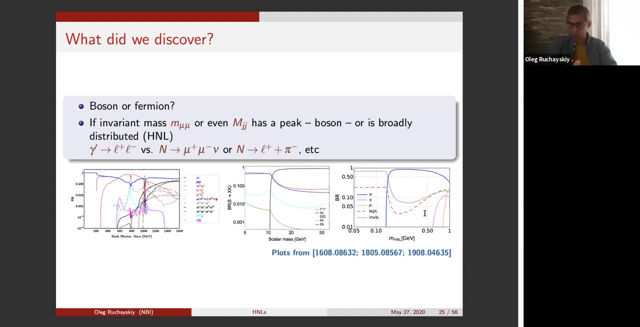 its decay patterns are consistent with heavy neutral lapland And its mass. if I am lucky enough to measure decay of HNL to meson plus pion, a very nice particle from an experimental point of view can be determined with sufficiently good precision. 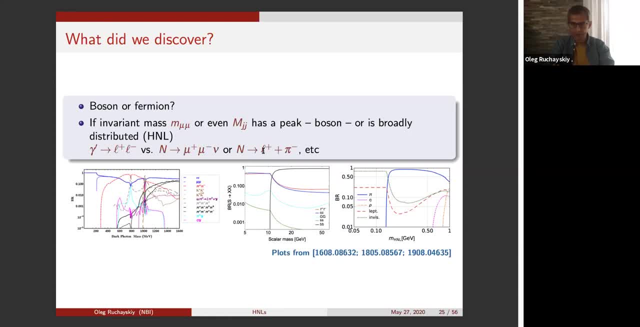 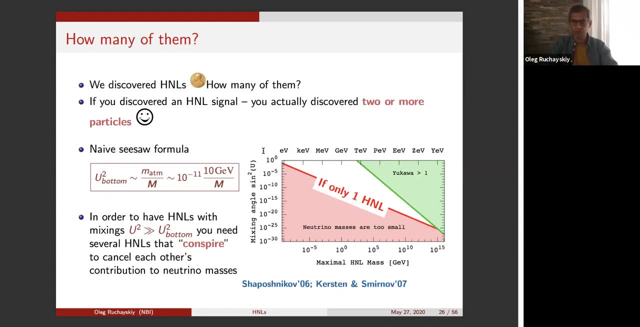 Okay, What's next? Actually, the interesting thing is that if tomorrow, LHC discovers such particle, this will mean that they discovered two such particles, not one. Why? Because, as I told you, if you would have only one, HNL. 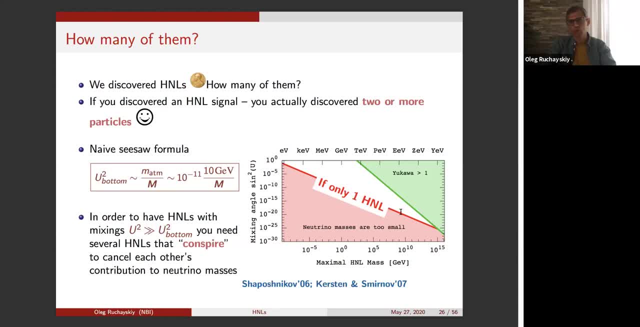 its mixing, the function of its mass, would be sitting on this lower boundary, which means that for the 10 GV HNL you would be probing. you would need to probe mixing at the level 10 to the minus 11.. Typical bounds today: 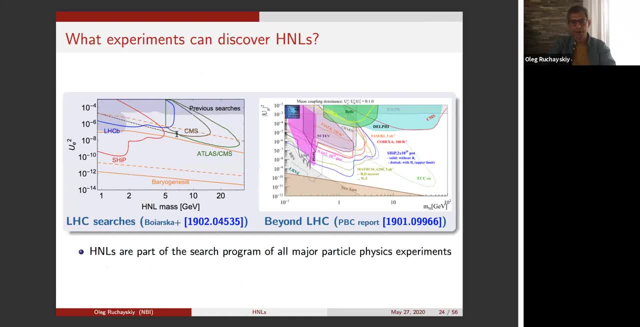 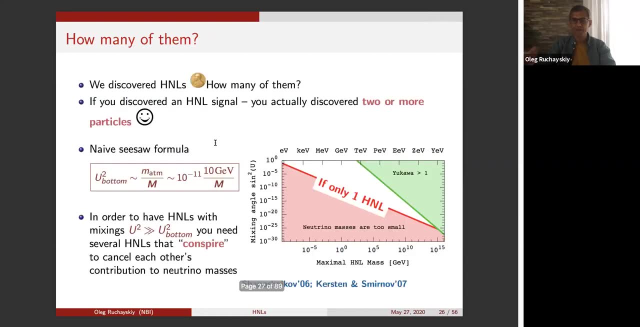 are at the level 10 to the minus 5.. And LHC may go to 10 to the minus 8,, 10 to the minus 9.. To sit so much above the CISO line, the bottom line, you need to have two HNLs. 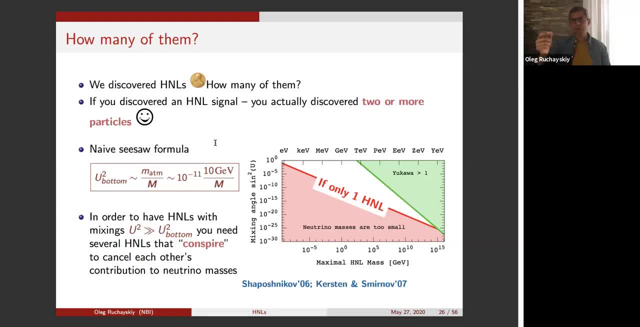 who should be almost degenerate in mass. Then big enough. mixing does not lead to big neutrino masses Because otherwise, if you just scale this thing up, mass of neutrino scales up And this starts to be incompatible with neutrino data. 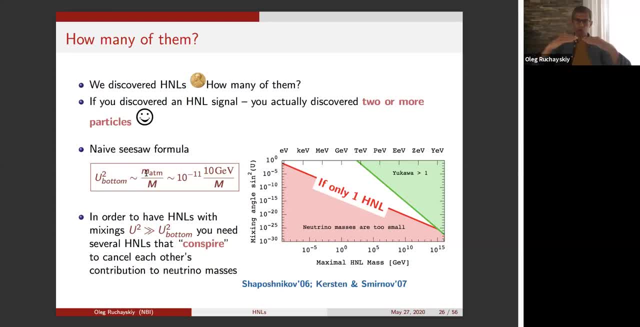 However, there are several particles that are sufficiently close in mass. They cancel each other's contribution to the neutrino masses, but they don't cancel their contribution to the decay events at the LHC. And so, essentially, if you discover HNL at LHC tomorrow, 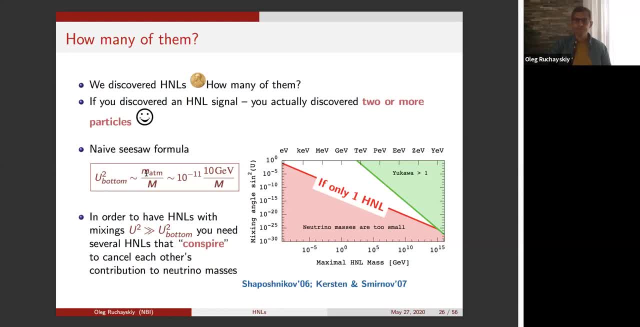 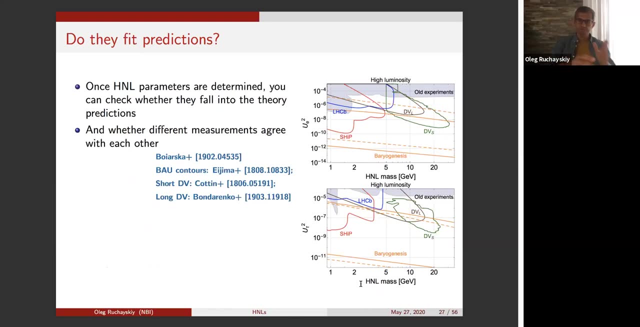 you discover two for the price of one, Which is nice. And, yes, there's a whole discussion about this cancellation by Mischapschitz and by Kaschitz and Smirnov. Now, once you determine the HNLs, you can study them in various channels. 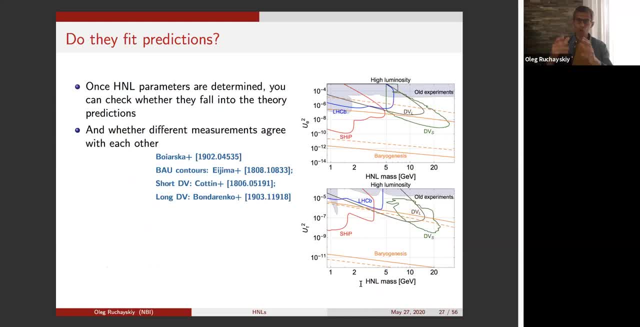 There are many complementary experiments. You can do the studies and you can actually measure not only masses, not only total lifetime, but also various branching fractions. So you can determine with certain precision even the flavor mixing angles. Then you ask yourself: are these really the Majorana particles? 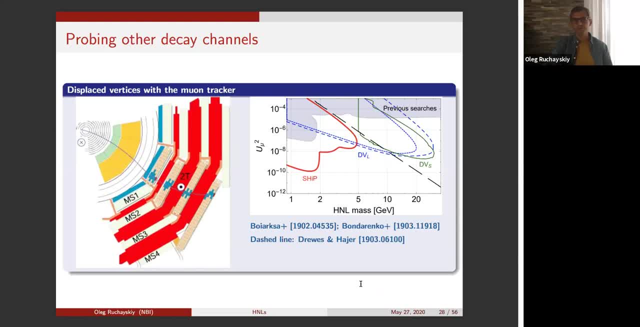 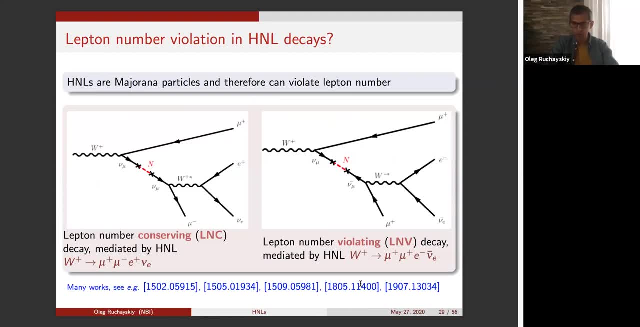 or not. What does it mean to be a Majorana particle? Well, to be a Majorana particle means to violate lepton number. Formerly heavy, neutral lepton is lepton, so it carries lepton number. However, as I said, 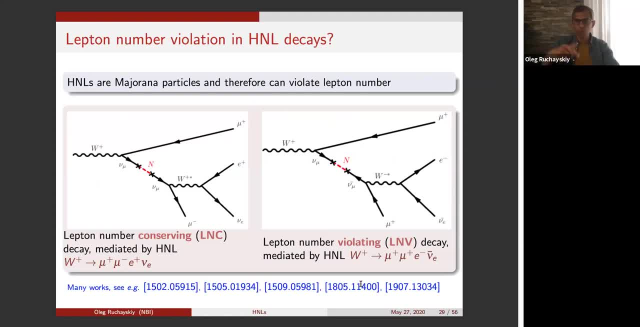 the Majorana mass prohibits any global symmetry, And lepton number is a global continuous U1 symmetry, And so if my HNLs exist, then they can be produced in lepton number-concerning events, Like in this one: W decays to muon to HNL. 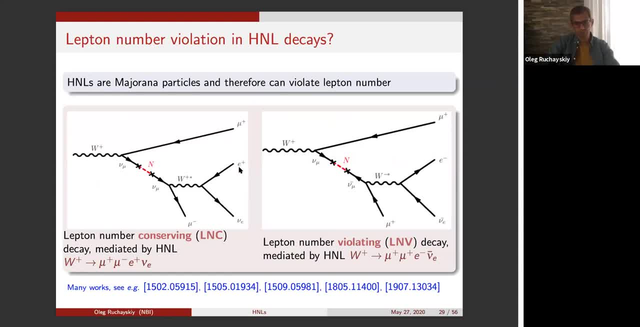 HNL decays to another muon, but of a different sign, And then positron and electron neutrino, So lepton number is conserved here. Okay, If you look at this decay channel, the situation is different, because both of your muons are mu pluses. 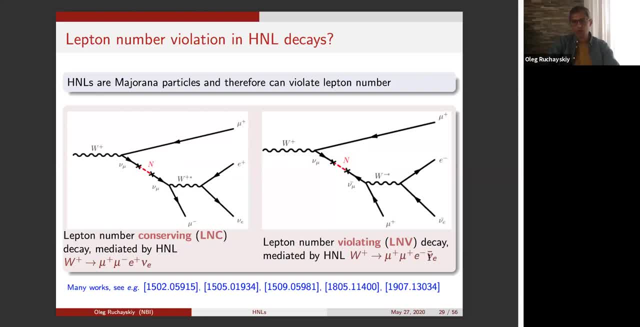 And then the electron is E- and the neutrino is electron anti-neutrino. But this is because this particle, what does it mean to be a Majorana particle? It means that you can decay to something and also to the charge conjugated something. 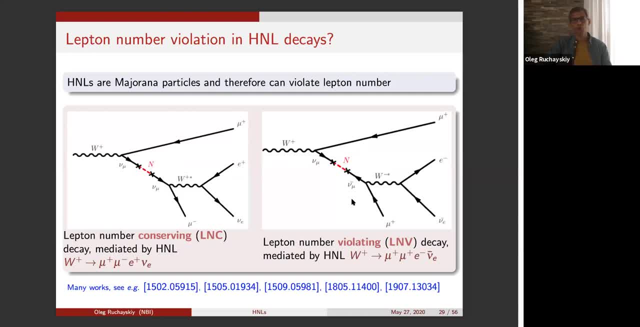 So here HNL decays to W plus, mu minus, And here the same HNL decays to W minus of shell, W minus and mu plus. That's what Majorana is. It's kind of two different holistic states, to be precise. 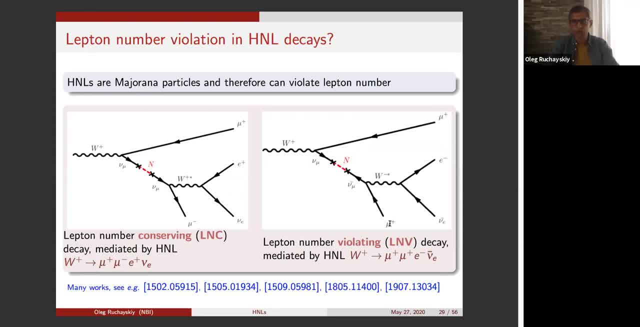 And there are many words which discuss how to study this at the LHC, Because lepton number violating processes are not part of the standard model otherwise, And their backgrounds are greatly suppressed And so you have much cleaner signatures. Unfortunately, the same story which cancels. 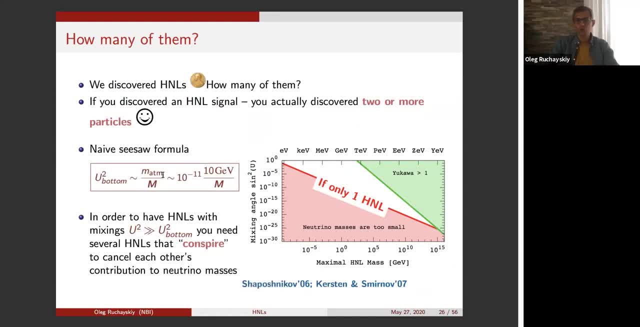 the contribution of several HNLs to neutrino masses also cancels lepton number violation, If you think. because neutrino mass is Majorana neutrino mass, the contribution to it and contribution to lepton number violating process is of the same footing, as discussed again. 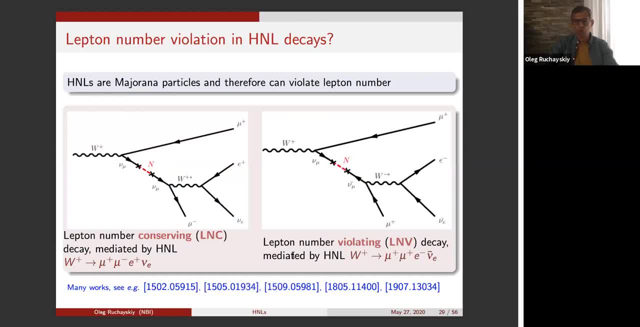 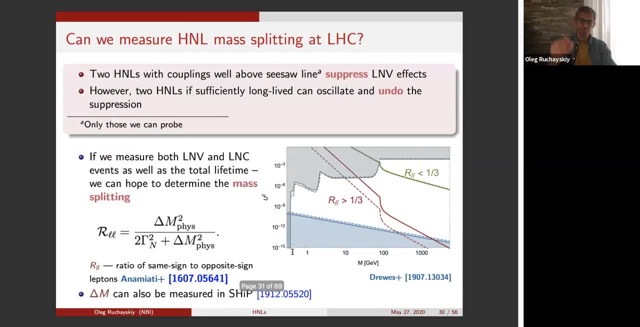 by the same people. So on the one hand, this doesn't seem to be a very promising interaction. However, if you think about this more, it turns out that because your two HNLs may not be of the same mass, but can be- 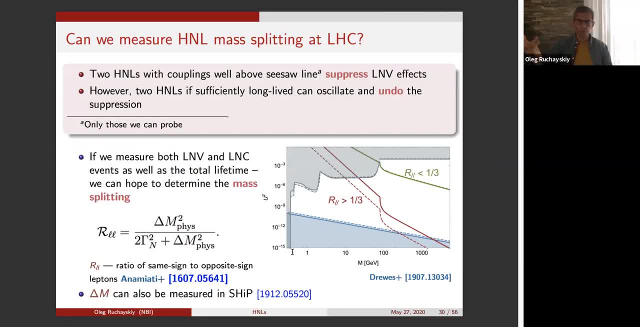 almost degenerate. So their masses may be very close- one per million, one per billion, but not exact. And in this case, not only they are produced, they can oscillate and fly. They are long-lived particles And this opens for you certain ranges of. 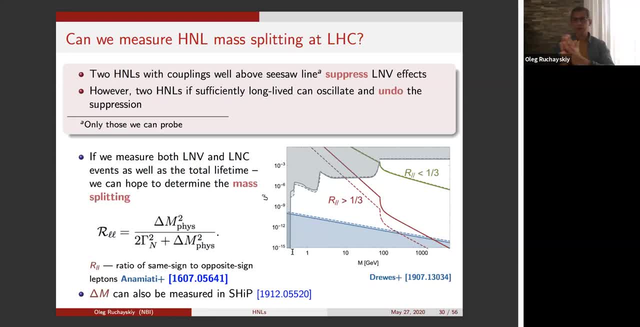 parameter space where you can see both lepton number violating and lepton number conserving properties And, more morally, if you measure enough of them, you can actually see the ratio proportional to the mass difference times, the lifetime and decay widths of the lifetime, as discussed, for example, in this paper. 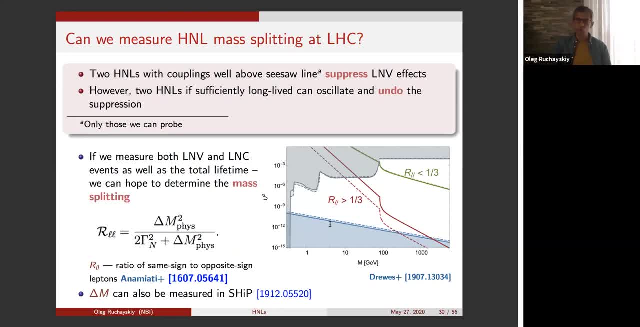 And which opens for you a nice possibility to search at the LHC, not only for Majorana or HNLs, but also to measure the range of parameter space, at least their mass splitting. So you're getting one more prediction out of those which you want to measure. 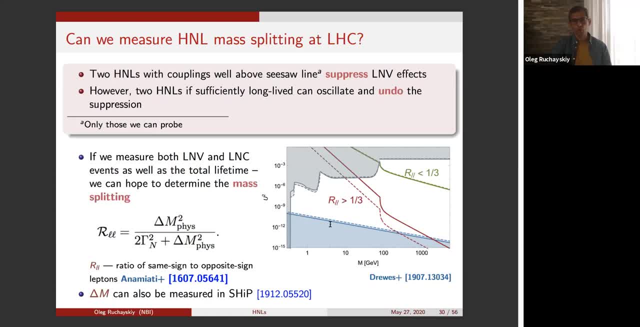 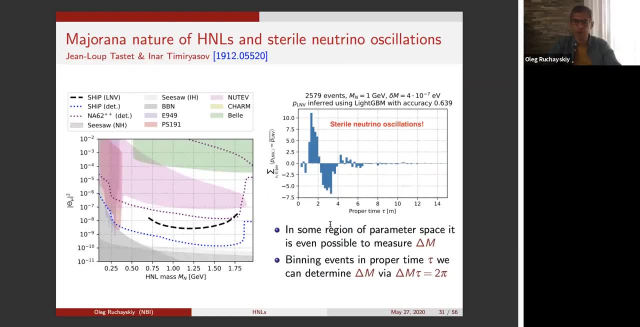 And, what's more interesting, you can do it not only at the LHC, but also at other experiments, like the experiment called SHIP, one of the hypothetical intensity frontier experiments, where particles are produced at the target by 70 meters and then decay. 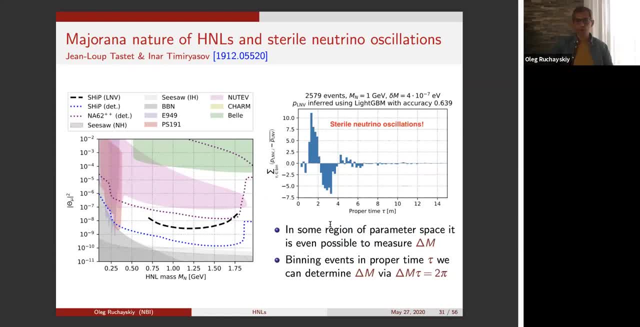 in a long decay vessel And there you can literally see neutrino oscillations. If you have enough events somewhere here- and that's the parameter space where a SHIP would be able to probe, It goes to 10, to the minus 10 also. 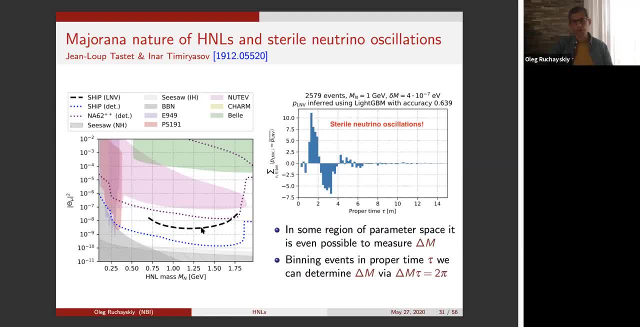 almost for small masses. And if you want all this magnitude, above you have hundreds of events, You can bin them in their proper time and you could literally see traces of oscillations of such particles. And from the period of these oscillations you will measure the mass splitting. 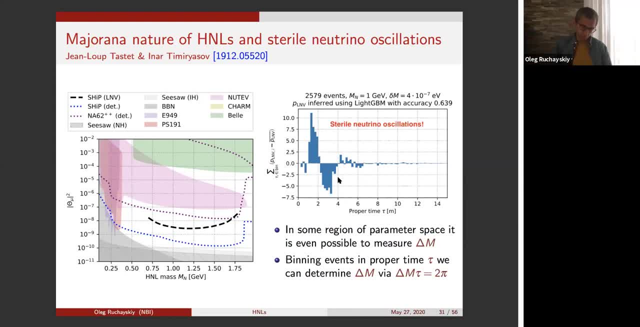 So in the, in certain worlds, you will be able, within five years from now, when SHIP will be operational, you will be able to measure both HNLs and their mass splitting their oscillations. There are no good ideas of how to measure CP violations. 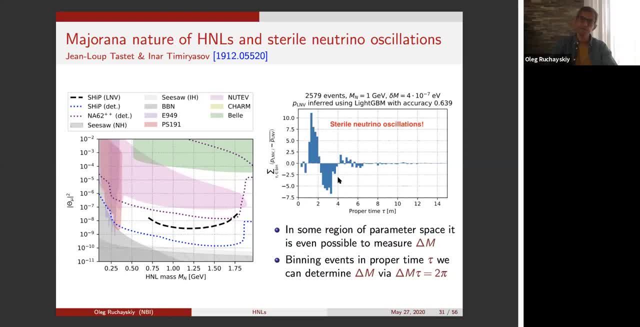 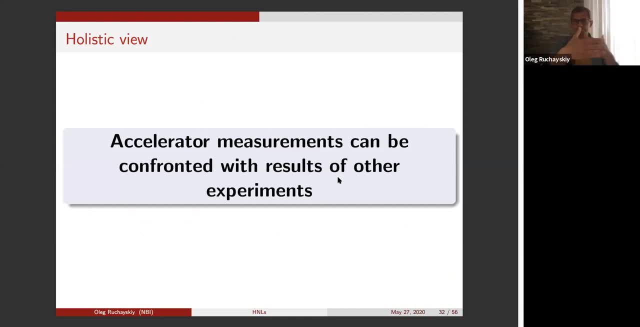 in the HNL sector. That's left for the future. So, in short, accelerator measurements complemented to each other, LHC, non-LHC experiments, and all together they can determine the heavy neutral leptons responsible for bariogenesis and for neutrino oscillations. 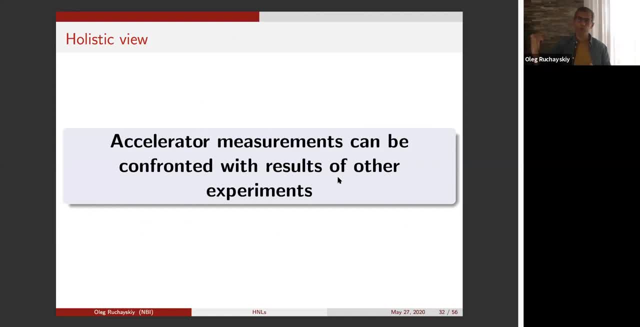 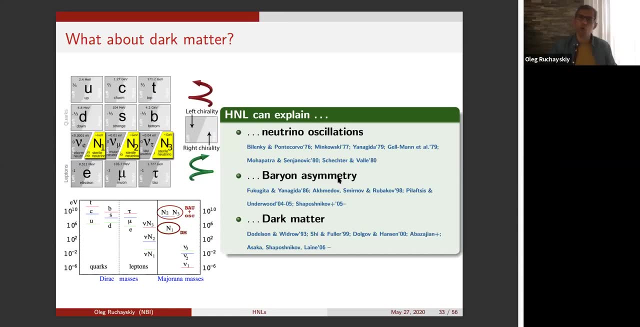 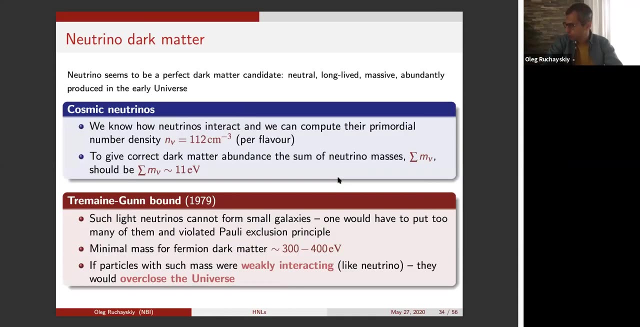 And measure many of their properties, to be confronted by theoretical predictions. However, let's now go to the question of HNL and dark matter. The idea of HNLs and dark matter, as I said, was developed in parallel to the ideas of HNLs and neutrino oscillations. 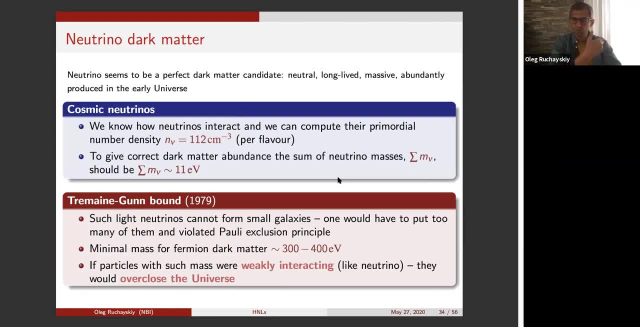 And more or less the line of reasoning is the following: People used to think that dark matter is neutrino, Because neutrino is neutral, stable, maybe have some small mass and is copiously produced in the early universe In every cosmology course. 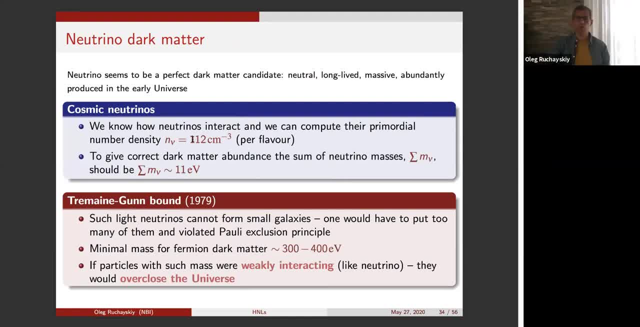 you do the computation that per flavor of neutrinos you get 112 particles per cubic centimeter. However, if you ask yourself what mass should my neutrinos have to explain all the dark matter abundance, you will see that the mass should be 11 electron volts. 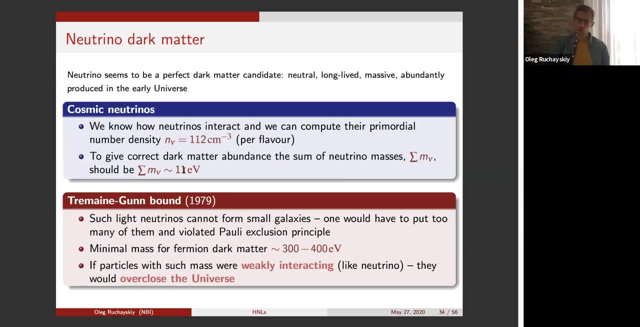 Which is incompatible with what we know about neutrino masses today. Today's neutrino masses are below 0.2 electron volts- the sum of them, And that the electron neutrino is below 2 electron volts from direct measurements. And not only: it's inconsistent. 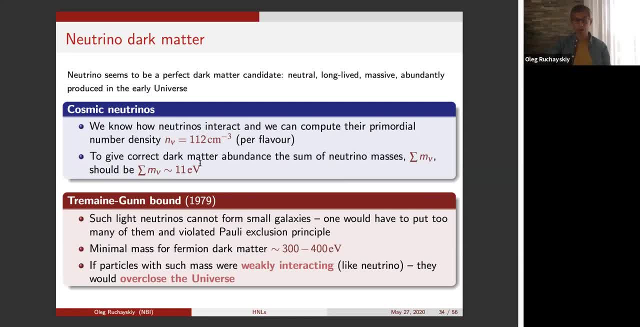 with the measurements of neutrino masses. it's also inconsistent with the fact that neutrinos should be not only cosmological dark matter- dark matter which gives you the metric density of the universe- but also astrophysical dark matter, Something which gives the mass to the galaxies. 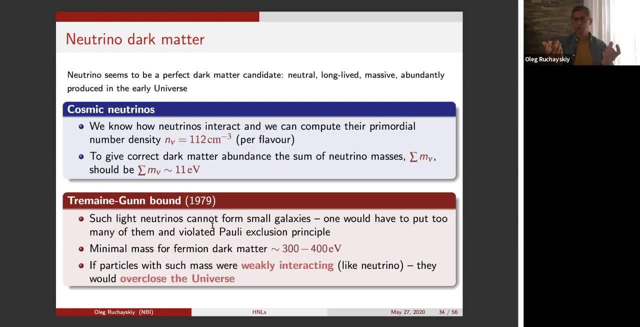 Because neutrinos are fermions. you have to have sufficiently many positions in the phase space to put them into the small galaxies. And the smaller is the mass of the particle, the bigger is the number to realize the same mass of galaxies. And as it turns out, 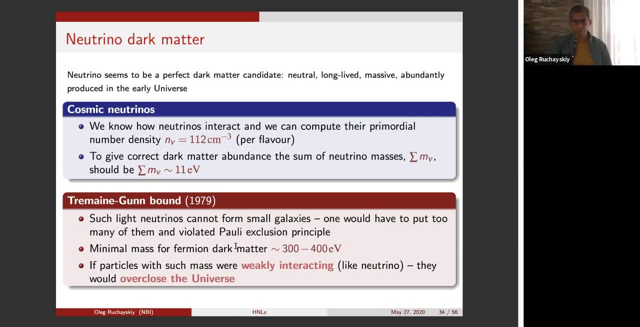 as was discovered by these people in 1979, for any fermionic dark matter, your mass should be several hundred electron volts or more, in order to not violate the power of exclusion principle when realizing small mass of galaxies, And this bound is the lower bound. 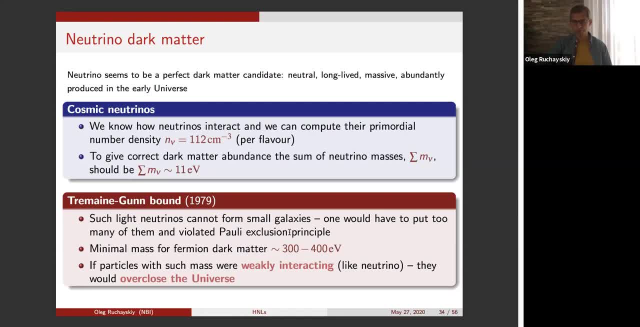 and this is the upper bound, for example, by a factor of 30 or so. So from late 70s, early 80s, people knew that neutrino dark matter is not really a dark matter candidate. So the only standard model, particle. 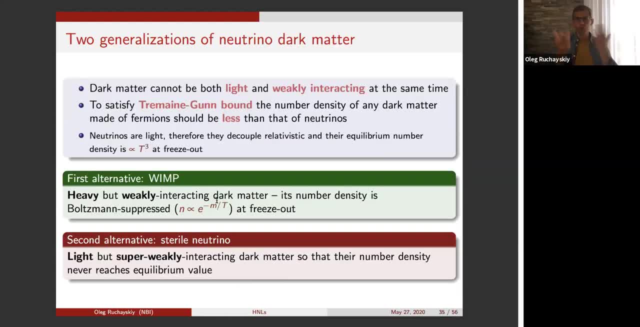 is not a dark matter. And if you think about this and if you move along these lines, you can say, okay, what went wrong? And you understand that for the Tremenghan mass of a few hundred MeV, your abundance number of particles was too large. 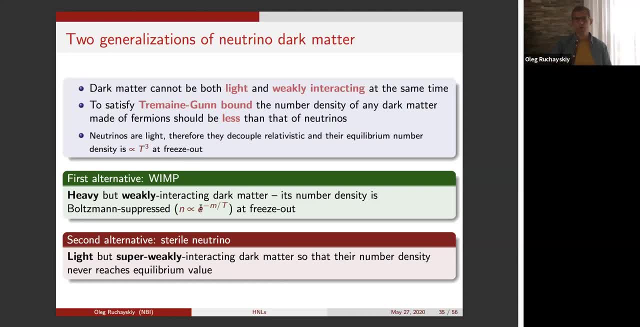 So you can reduce the number of particles. One is making the particle heavy, then the decoupling relativistic, and their number density is not t cubed but it's also suppressed. That's what's called weakly interacting massive particle, or WIMP. 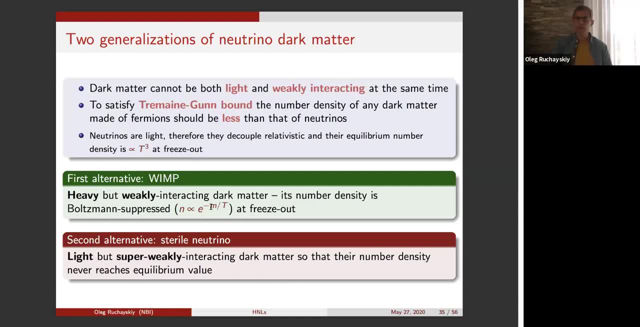 The first WIMP of Lee and Weinberg or Zeledovich and company was actually exactly cosmologically heavy neutrino. At the time there were no bound sources. Your second alternative is to make neutrino super weakly interacting. It's called sterile neutrino. 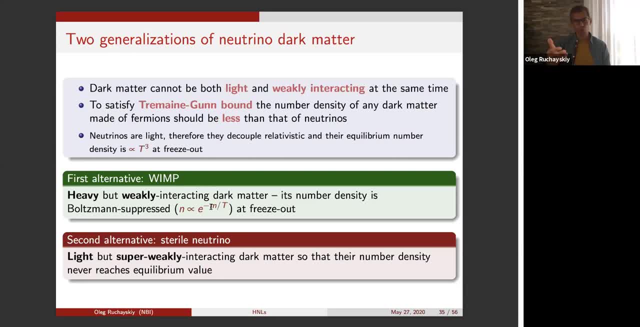 In this way they interact insufficiently strong, never interested in equilibrium, and so their abundance is sub-equilibrium And your energy density abundance is mass times number density abundance. So if you shrink the number density abundance, you can allow for larger mass. 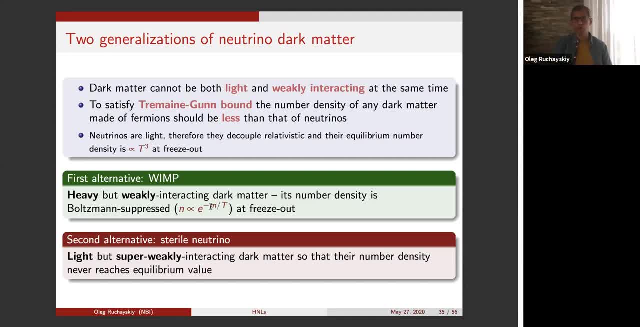 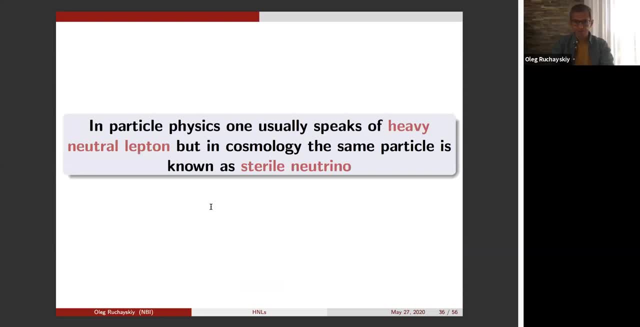 And that's what sterile, neutrino dark matter is. It's realized by Duderson and Wintrow in 1993 and then by other people later on. And again here I should say that in particle physics these particles are called heavy neutral leptons. 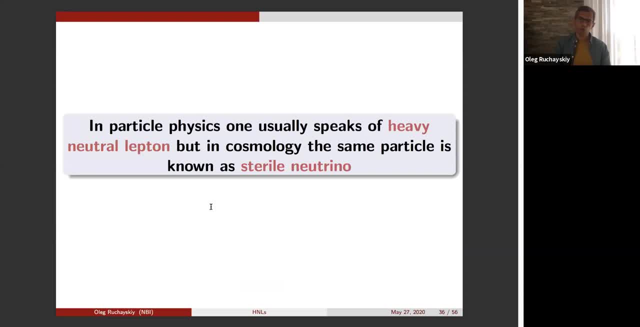 and in cosmology the same particles are usually called sterile neutrinos Historically, And there is also electron-volt sterile neutrino, which has nothing to do with the story because it's not a dark matter and it's not a part of the biogenesis. 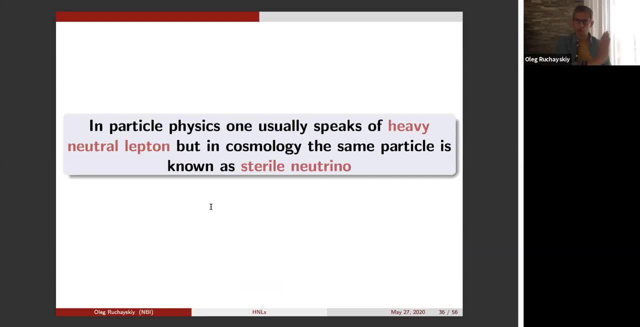 so it's a completely different story. Electron-volt sterile neutrino is our force neutrino which can explain the lesson. It's not in this picture, But here. I will sometimes use the word sterile neutrino, simply because, for dark matter, that's the name. 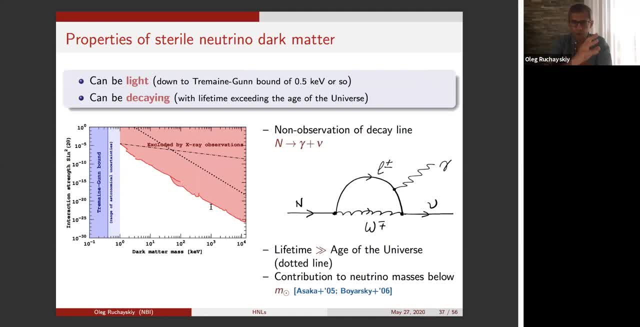 Okay, If my sterile neutrino is dark matter, then its mass can be light, but no lighter than several hundred triple volts. Half kiwi order, half kiwi. It can be light. It doesn't have to be, but it can be light. 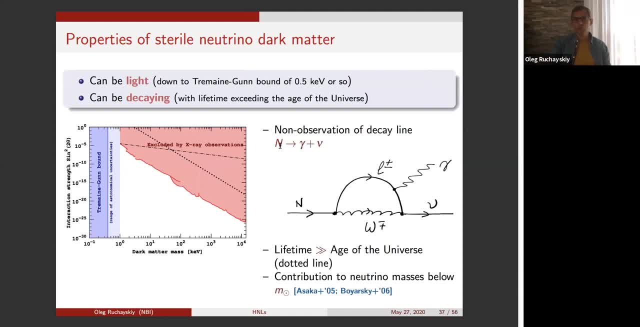 Its lifetime. it can actually decay. It can decay to three neutrinos, or it can decay to a neutrino and a photon through liquidated process And, surprisingly enough, the requirement that this particle is heavier than the lifetime of the universe is not enough. 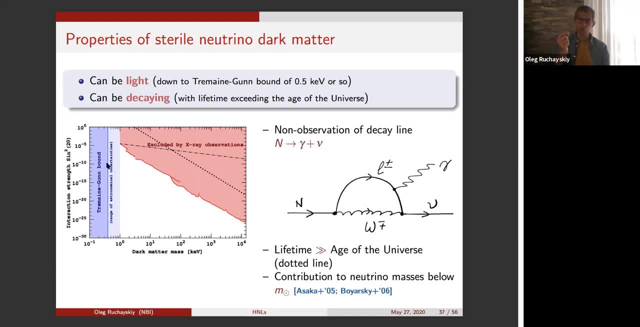 The fact that you have so many dark matter particles that, even if they produce decay once per lifetime of the universe, you still have a very strong flux of X-rays that would come from any galaxy, Like if they would have a age of the universe- lifetime. then the Andromeda galaxy would be. 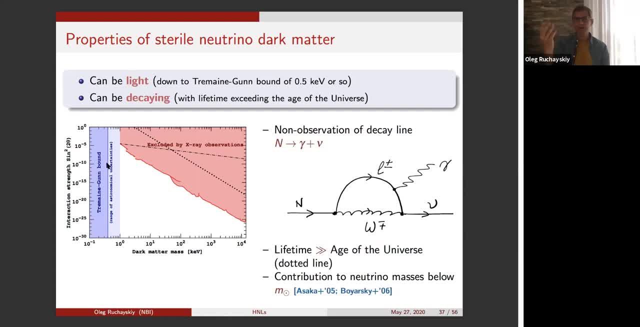 shining at one X-ray frequency with more brighter than the whole X-ray emission of Andromeda galaxy from astrophysics. And so, because of non-observation of this decay line, you can put a strong bound on the interaction strength of sterile neutrino. 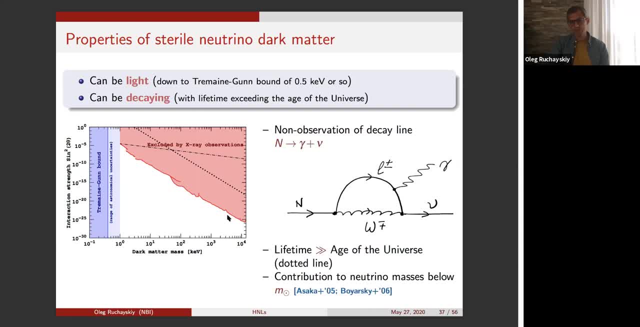 the same mixing angle as a function of mass. This is a large region. This is cut by this power exclusion principle arguments and this is cut from non-observation of X-ray emission And this is the lifetime And that's contribution of the dark matter. 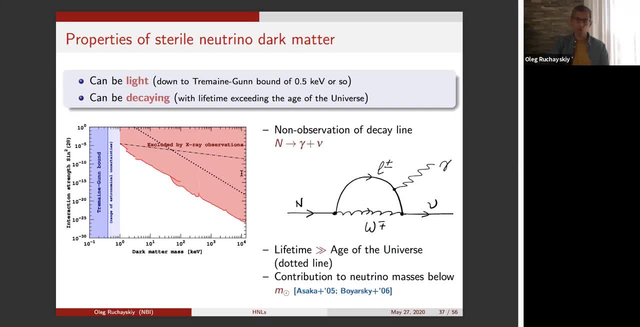 neutrino. Neutrino is such a mass coupling constant to the neutrino oscillation, So along this line it contributes to the level of solar smaller neutrino mass differences. So everything below here gives you negligible contribution to neutrino mass. Now 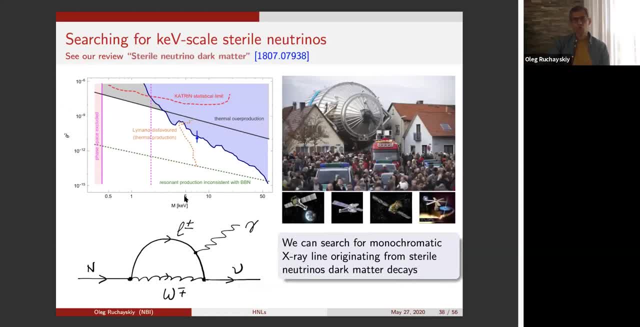 it should be said that if you want to search for key V-scale sterile neutrinos and even experiments like Katrin, is not compatible with X-ray bounds because essentially Katrin operates with tiny amount of tritium and galaxy like Milky Way has 10 to the 70 dark matter particles. 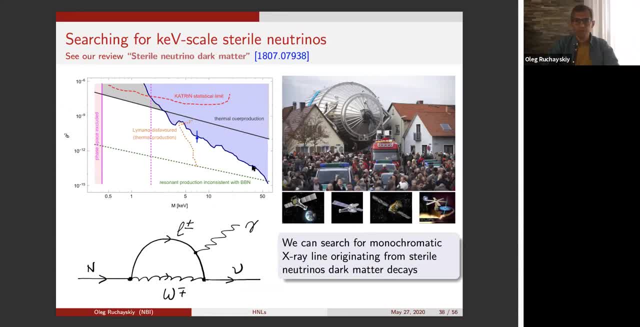 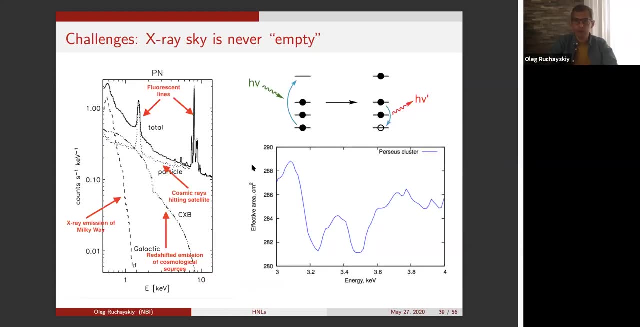 of this mass. So your X-ray line searches become the dominant source of information about dark matter, sterile neutrinos. This search has been conducted by many groups over many years, since beginnings of 2000.. And surprising as it is for people who are not in the field. 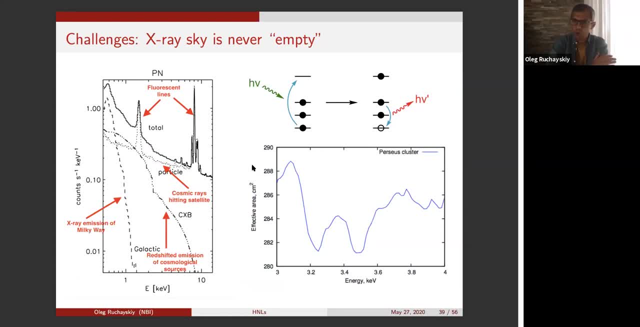 X-ray sky is very non-quiet sky And there are many X-ray telescopes. all of them are satellite based because X-rays don't penetrate the atmosphere And if you look at what X-ray telescope measures, it mostly measures parasitic signal. This is the spectrum of 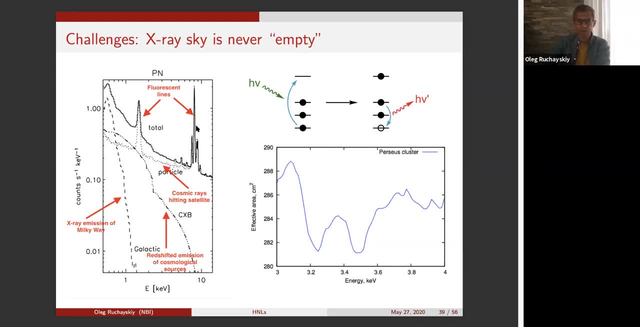 typical X-ray neutrinos, And every line here is not an astrophysical line, it's a fluorescent line. A photon comes, heats your detector, it excites an electron just in the material. then it gets remitted back and it's K-alpha of all the metals. 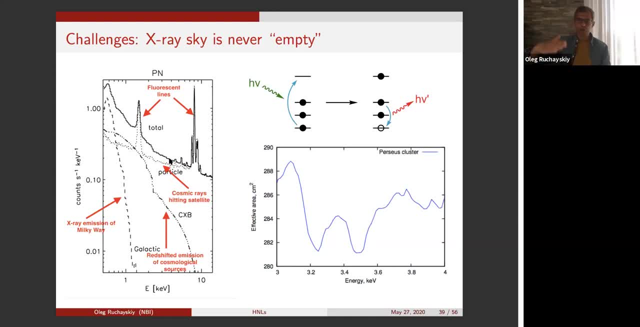 of which the satellite is made, And then there are other induced particles in the ground because of soft protons which heat the detector by passing the mirrors, because of all sorts of stuff. So it's very complicated to search for a narrow line on top of the astrophysical. 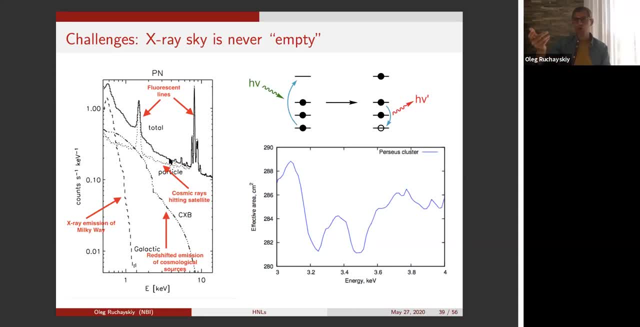 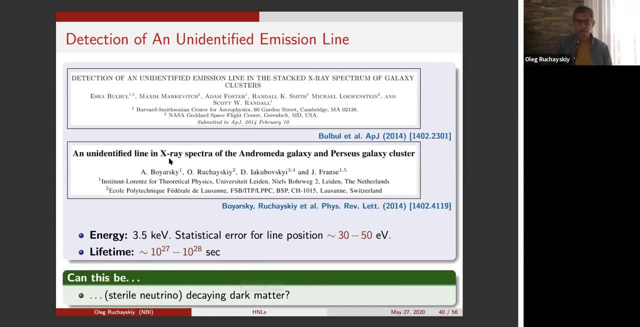 emission. On top of this, most of your gamma-dominated objects are also X-ray active. So, as I said, many people were doing this work for many years and, given some recent developments, I should speak a little bit about the work which we did in 2014. 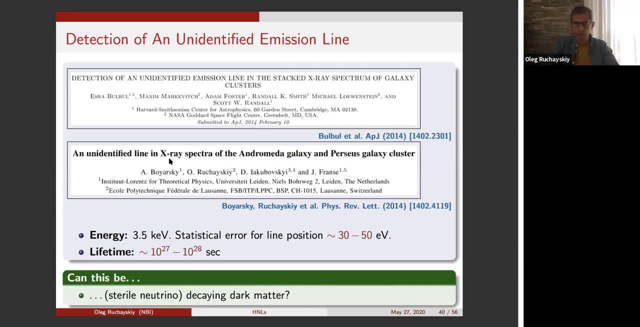 when two groups with an interval of one week reported that they see a line of energy about 3.5 kV which they cannot identify with any non-astronomical lines and they think it's not systematics And this line comes from a. 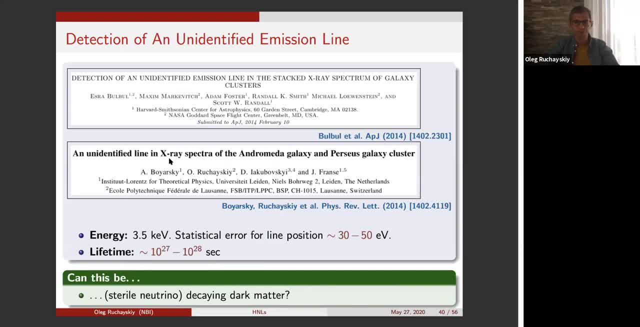 spectrum of gamma-dominated objects, galaxies and clusters of galaxies, And these are two independent worlds and two independent sets of data And the question, of course, people became very excited because the question was: is this decaying dark matter finally discovered, and if so, then can this be probably sterile neutrino dark matter? 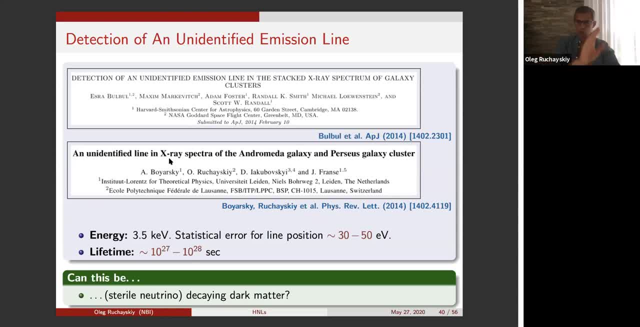 One doesn't imply the other. It may be non-dark matter signal, it may be dark matter signal, but no sterile neutrino dark matter, and it can be sterile neutrino dark matter. So what I speak about from now on, it's not really about sterile neutrino dark matter. 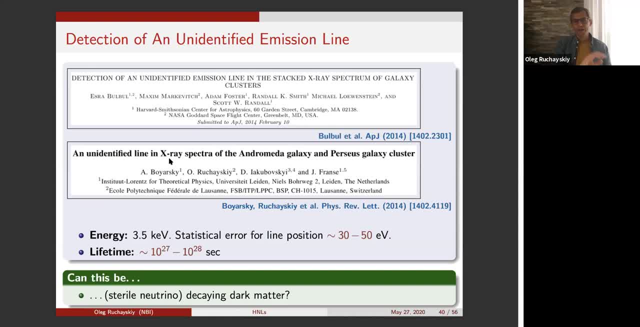 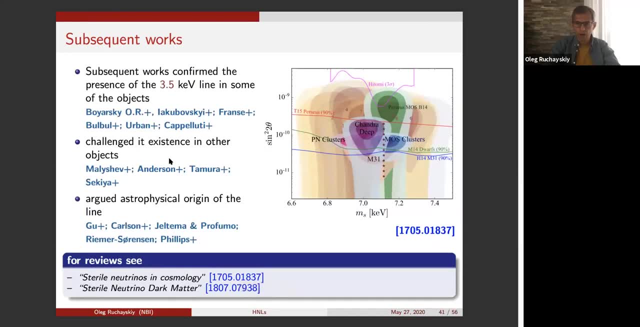 it's about this decaying 3.5 kV line, which can be interpreted as any of your favorite models- A lot of interest this subject has generated. Many subsequent works have discovered this same signal in other types of gamma-dominated objects. Other groups did not find anything. 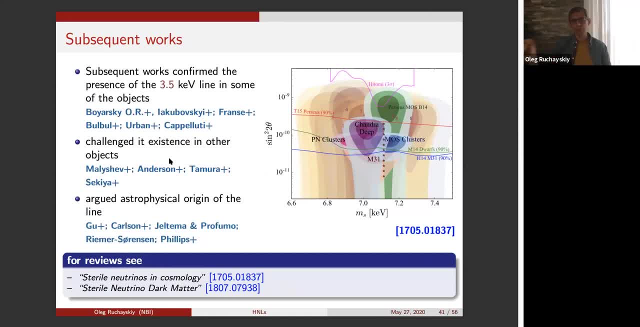 challenged what they saw. Some people explained this is systematics, some people said this is astrophysics. There are several reviews which I would recommend for you to read And this is a plot made by which more or less tells you the story. So there are a lot of detections. 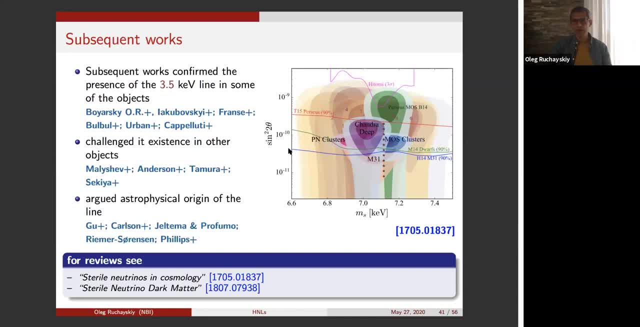 these are the shaded 1, 2 and 3 sigma regions and there are various non-detections which put certain bounds. So everything above any line is excluded And it looks messy and you see that things are roughly consistent after, and of course you shouldn't take all this 1, 2, 3. 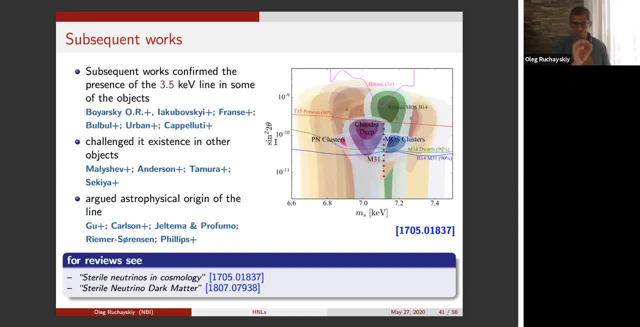 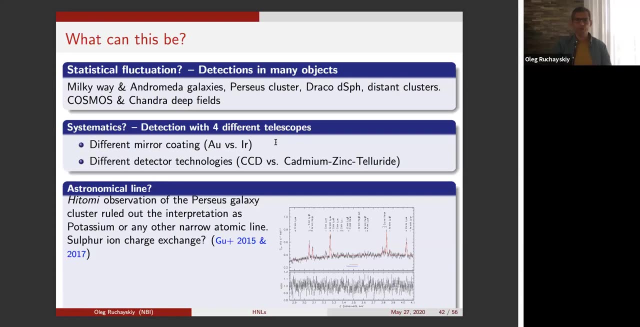 sigma bounds, like at face value, and there are uncertainties. This is not a controlled experiment of particle physics yet As we are today. this thing has been detected in many objects with significance from 3 sigma to 4 to 5 sigma. we all know that 5 sigma is. 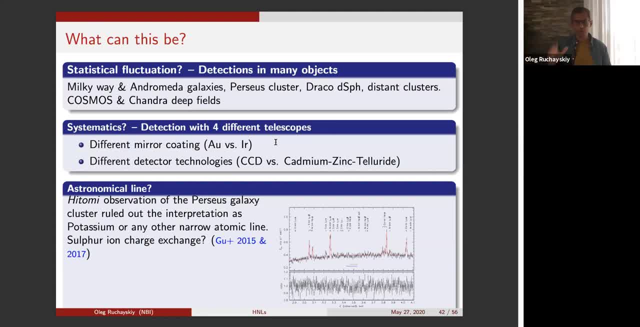 discoveries, but not in astrophysics. There are examples of 5 sigma detection in astrophysics, which is actually spurious, because systematics is very hard to control. Speaking of systematics, something which is related to the structure of the detector, It has been observed. 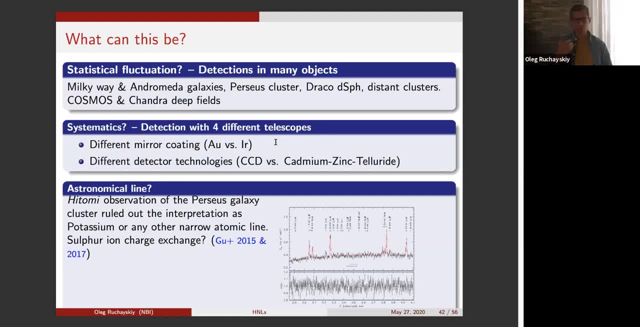 with 4 different telescopes made of different materials in terms of mirrors, different materials in terms of detectors. It's not clear what systematics goes through all of these telescopes. People discuss this may be some astrophysical lines. Kyiv region is very astrophysically. 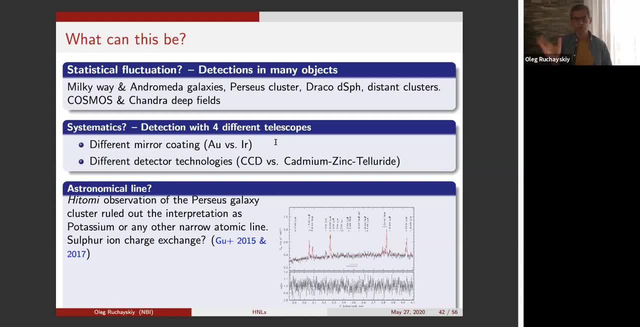 active, and so pick any frequency within 100 electron volts, you will see some astrophysical transition. However, one of the observations made by a satellite called Hitomi, which was the only really high resolution satellite which have a fluid or only existed for two weeks- 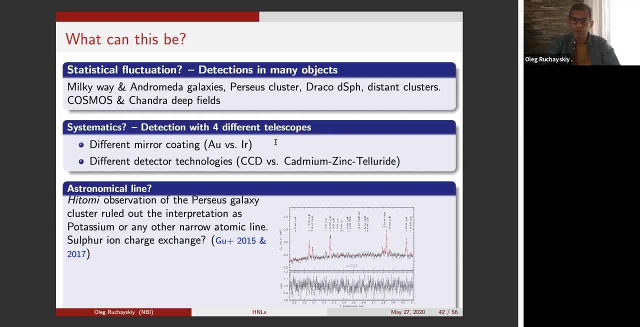 and it was malfunctioned and stopped working. It looked at the place where the emission was very strong and they didn't see any astrophysical lines there, And for this kind of spectrometer astrophysical line is narrow and the metal line is broad. 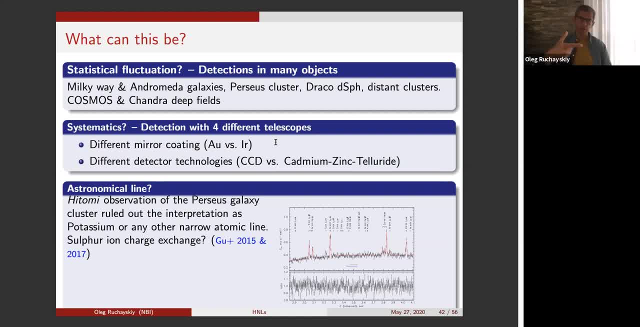 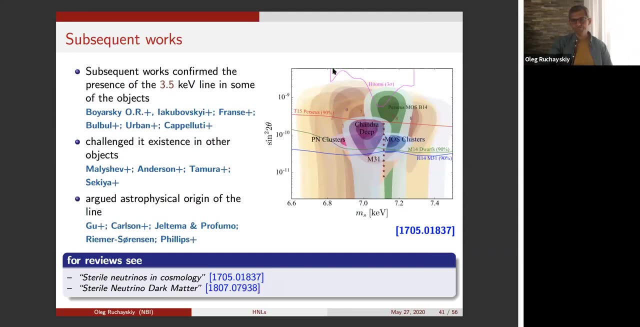 And of course it takes much more observational time to detect the broader line because it's more beans and so number of extra photons per bean is smaller. So if you look for example here, Hitomi did not determine a small dent in dark matter. interpretation of 3.5 Kyiv line, but without 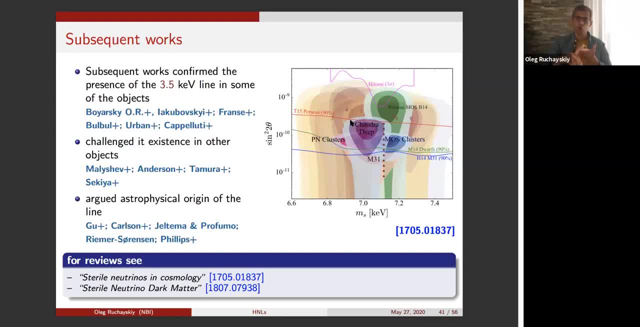 astrophysical origin. So it's neither statistical fluctuation nor systematics that we know of. It's more astrophysics It may be a combination of those. For each non-observation you will give some of the explanations. then you can combine. 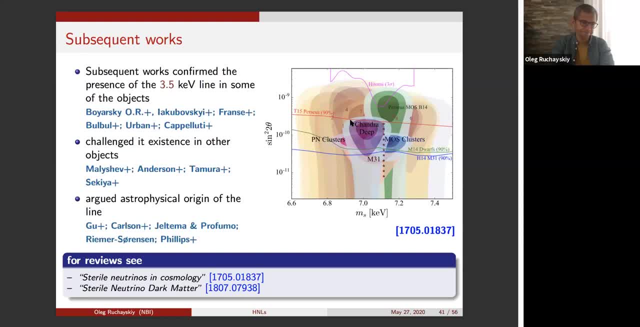 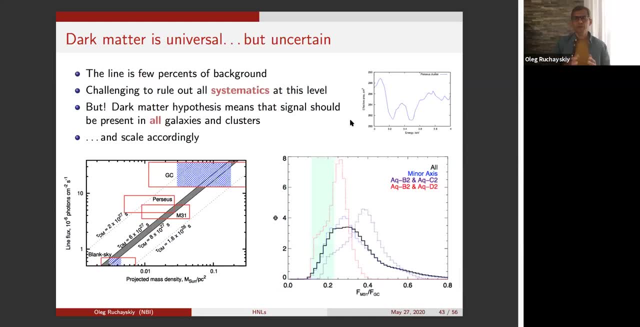 things, But if you won't explain everything from one, then there is no convincing explanation what it is. Now. it's very difficult to rule out systematics when you work in uncontrolled environments like space. However, I understand that dark matter is universal. It's present in every galaxy. It's present in every 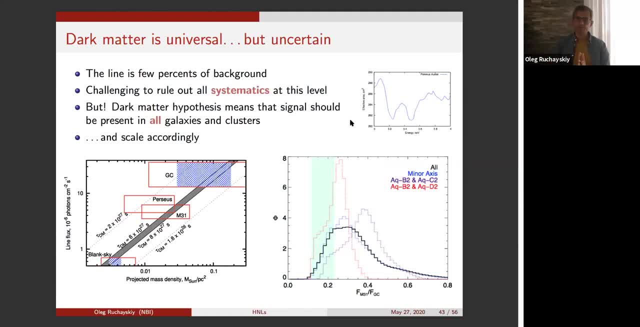 cluster. There are uncertainties, but essentially, if you see big enough sample of dark matter dominated objects- each of them exhibits a line is within needed uncertainties- then then you have a reason to believe that you are discovering dark matter, And this is what you see here. 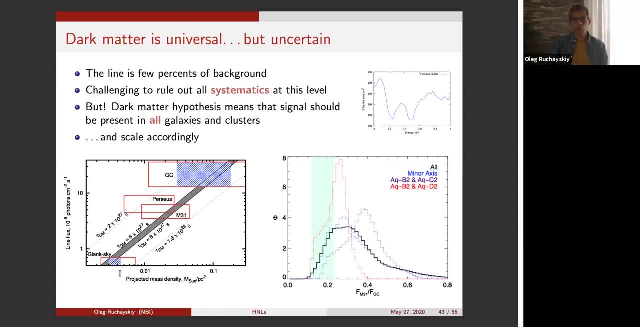 You. this axis is uncertainty in dark matter, the projected dark matter mass along the line of sight. This axis is predicted flux in the line which you see. This is a line of the constant lifetime And you see that everything you detect roughly sits along the 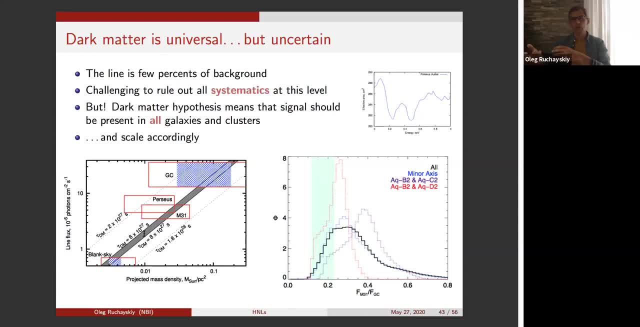 needed line And you can go to simulations and you ask yourself, okay, given that I observe that signal in Andromeda and that signal in the Milky Way, but different regions of those, How probable it is that they both come from dark matter, decay. 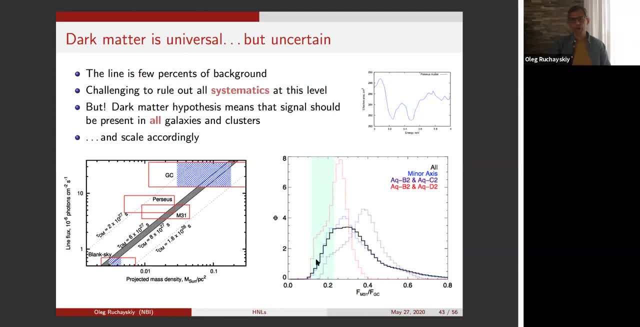 This is distribution of the ratio of the fluxes and this is where you are actually seeing clearly consistent with dark matter predictions, And you can play this game for a long time. I mean, it's very hard to prove things in this way, but it's a consistency check which you can. 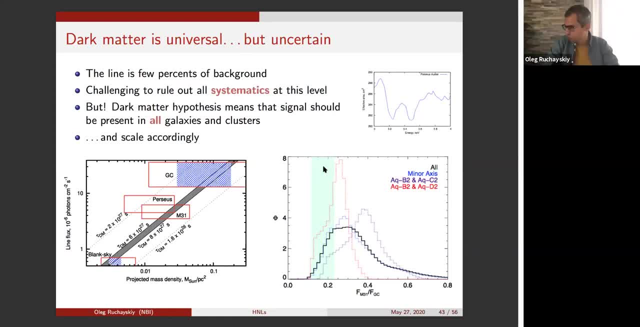 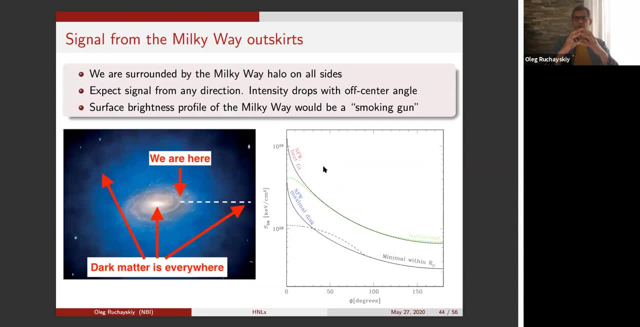 constantly run And a very important consistency check. and why I speak about this now is that in the Milky Way we are sitting 8 kiloparsec away from the galactic center and dark matter galore is around us. halo is around us with 100. 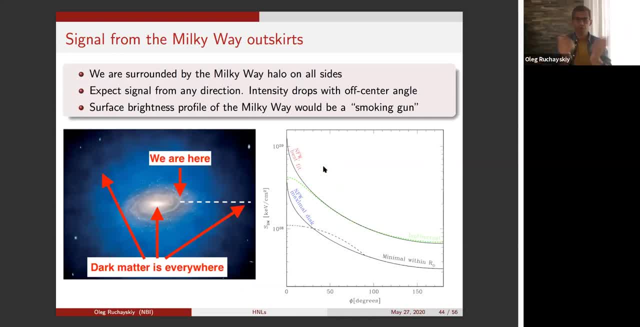 kiloparsecs radius, hundreds of kiloparsecs radius. So when you sit inside the dark matter halo, no matter where you look, here, here or here, you pick some dark matter signal, even if otherwise the sky is empty and there are. 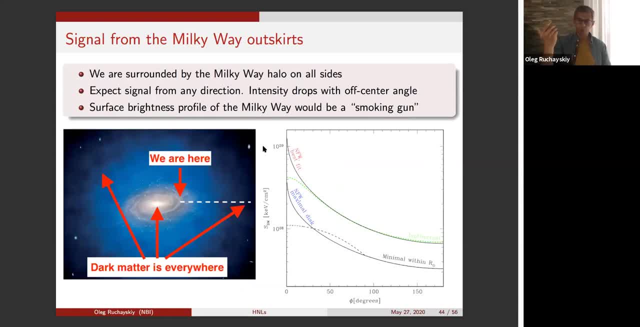 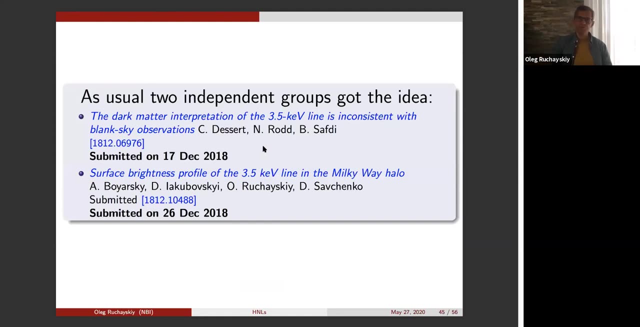 no galaxies in the line of sight. So, in principle, what you would like to do, you'd like to build a surface brightness profile of the line across the Milky Way sky and then compare it with prediction of dark matter distribution And, as usual, two groups have an idea. 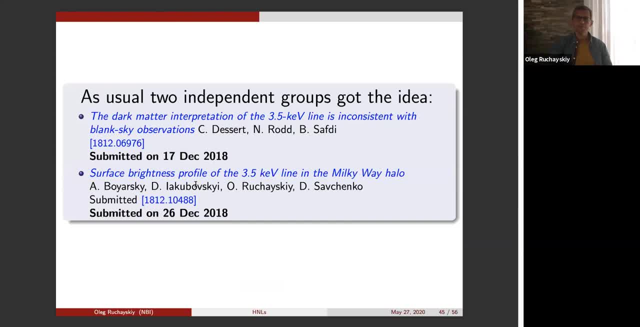 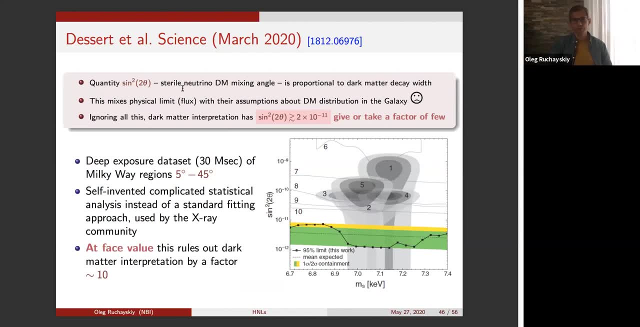 And then two papers appear within 10 days And some of you probably saw the press releases in March of this year when the first group got their papers, So they did publish inside. so it took a year and a half, which means never give up. 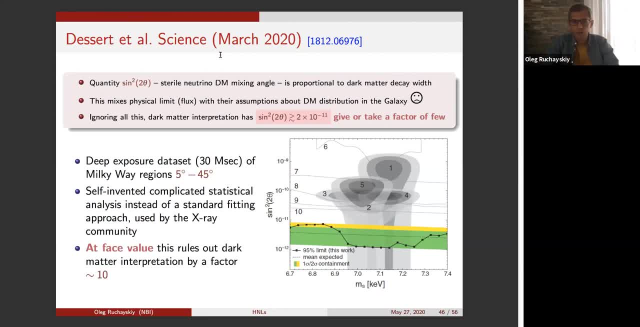 And they did a very solid work. They demonstrated that you take enormously big data sets- 30 megaseconds, it's huge. They split it into the regions. They implemented their own complicated statistical analysis, ignoring usual X-ray community standard fitting approach, because they have their reasons to believe. 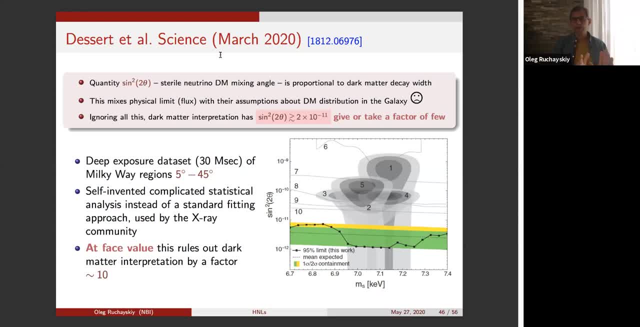 that there are some systematics there. And at face value, they say they ruled out the smallest dark matter signal predicted by other observations, by a factor of about 10. Which is a strong exclusion. At the same time, sitting on a very similar data, doing different statistical analysis, 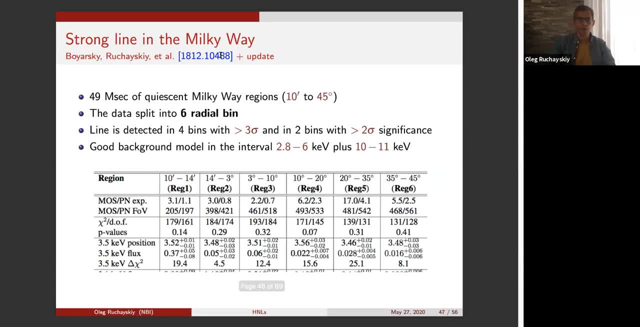 essentially standard in this community. We take comparable data set, We split into the six radial beams, from center going outwards, And we detect the line at the same frequency in every beam, For beams with three sigma significance to be one more than some two plus sigma significance. 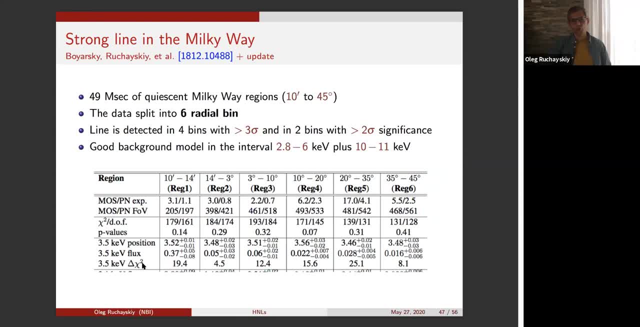 That's your detection. square root of this is your detection significance, roughly speaking. Okay, So this is a line And they don't. And the question is: is our line compatible with the Exclusion? First of all, what does it mean? this is a line If we take. 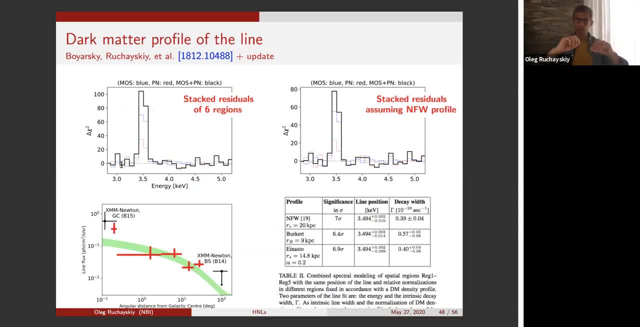 our six regions. with this line present and then put its flux to zero, We ask yourself: okay, how big is the residual? This is the residual in terms of the standard deviations. You see about 100 standard deviations. So the square root of 100 is about 10. 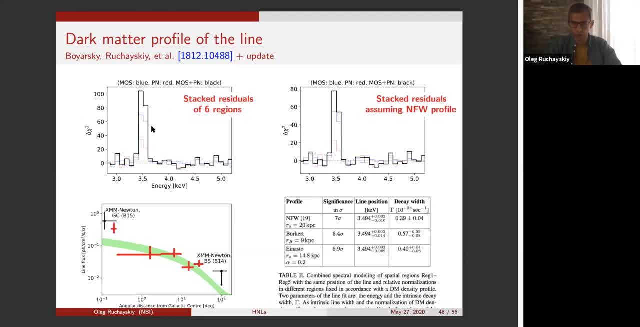 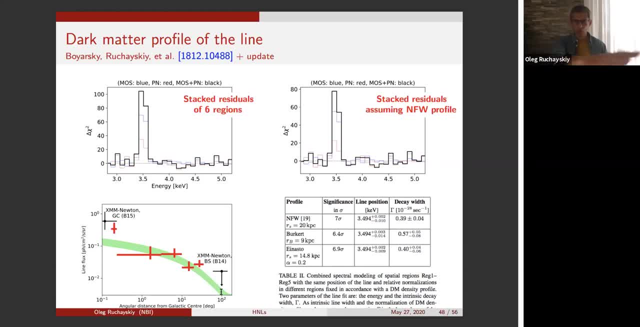 This is your predicted documenter density profile. This is one. It's not a fit or fight, just an illustrative example. But by taking the real document density profile and connecting all the six regions according to the document density profile, do you see the line? 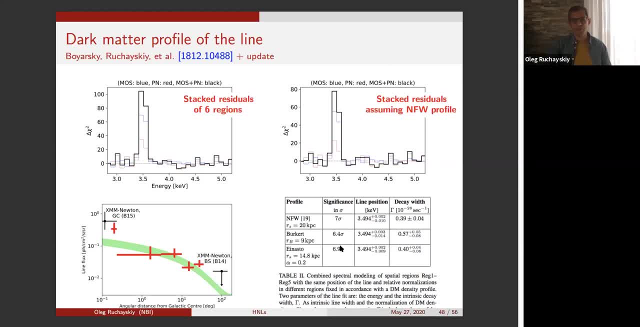 Yes, I do. I see the line there at seven sigma, from six to seven sigma, no matter which profile I choose. actually, I mean the significance varies, but not much because all the profiles should roughly agree with each other in the region of degrees. 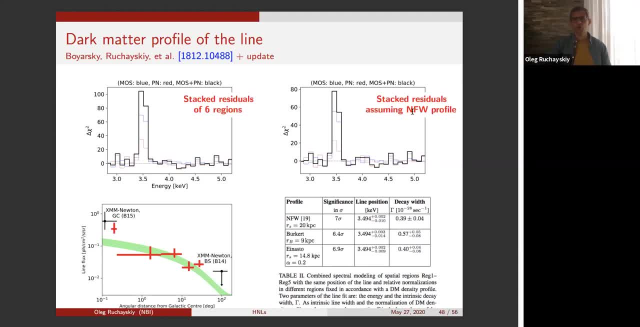 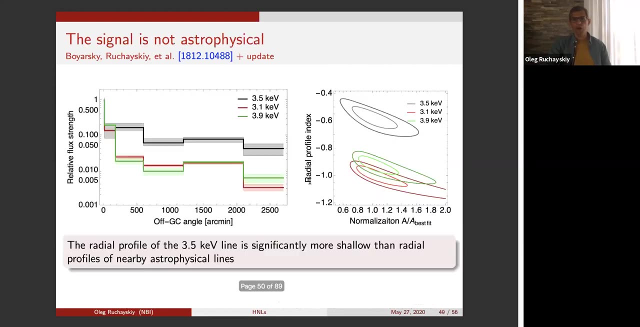 And again residuals, density profiles- again huge slack Around nine standard deviations. Of course it's less when you interpret it as two-dimensional, parametric fit, etc. Now is it compatible with astrophysical lines? There are other lines, astrophysical. 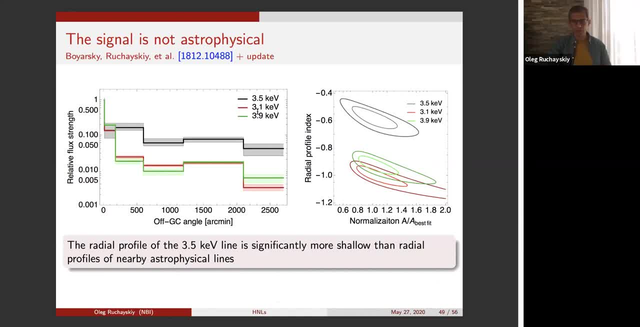 lines like argon or calcium emission lines nearby. They behave with off-centers of six regions. They fall off like that. This is a logarithmic scale. This is my line And if you compare the radial profile, slope your astrophysical 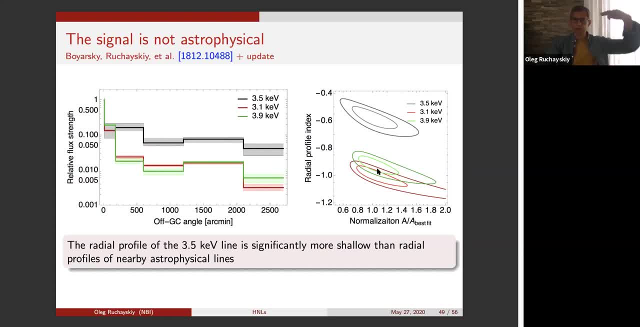 lines have the same roughly Radial profile, decay is off-center distance And your 3.5 kV lines is completely separate, much more sharp And again, this does not prove anything right, But this serves as the another consistency check that we see. 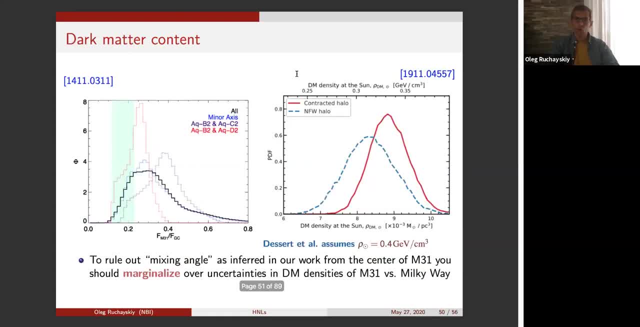 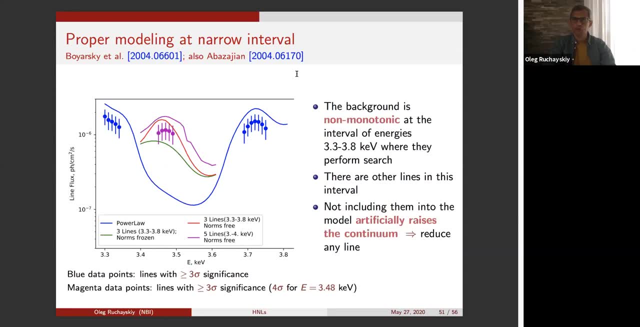 something and the something doesn't behave like astrophysics. Now, what went wrong between us and Desert Etal? We don't know, because it's difficult to reproduce their procedures. There are some details that are not there, But we tried to do. 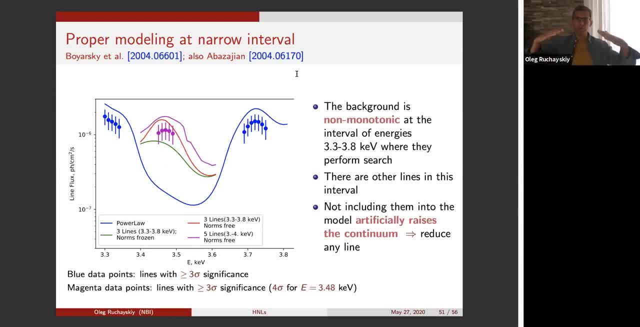 what they do and essentially they tried to fit a very complicated background model on a narrow energy interval And in this way you can compensate the presence of the line by under-subtracting the ground in one place and over-subtracting it in another place. 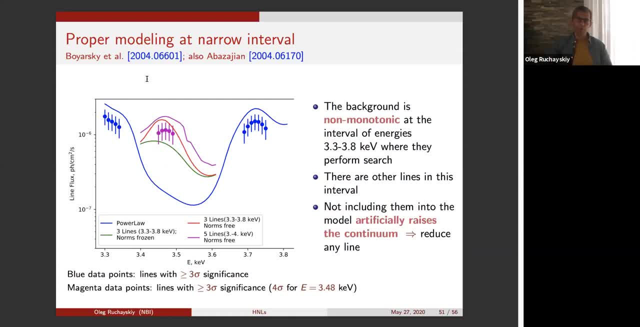 And we tried to repeat their exercise when the paper appeared. We also kept up with the jump, trying to do it independently of us, And this is more or less the bound which they get very similar when we reproduce it. But this is because the model lines 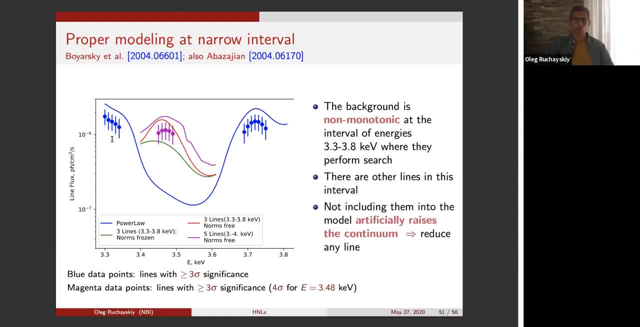 sitting here. these are 3-sigma residuals and that model also lines sitting whose tails enter the region. This is some technicalities for those who are interested and can speak more. So, to make a long story short, we believe that if you do conservative bound. 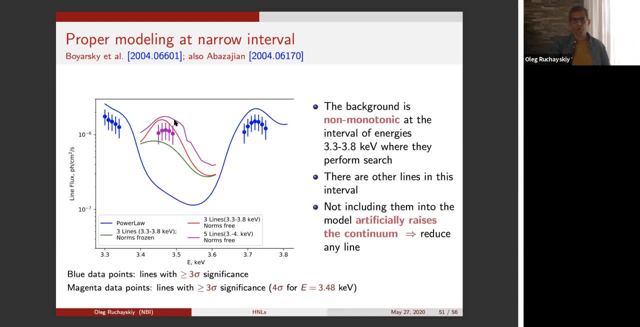 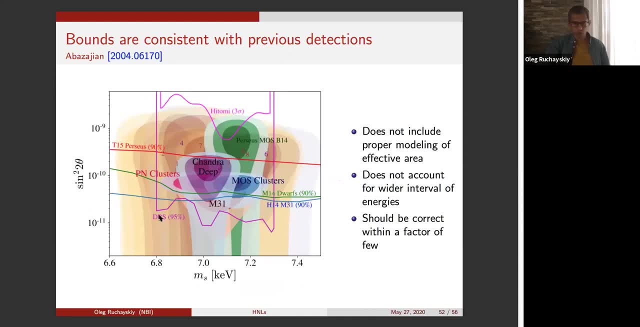 in a method similar to theirs, you will get about the order of magnitude weaker exclusions, And that's what Kev also concludes, who puts this desertile bounds onto their, onto his plot. Yeah, it's in some tension, but again. 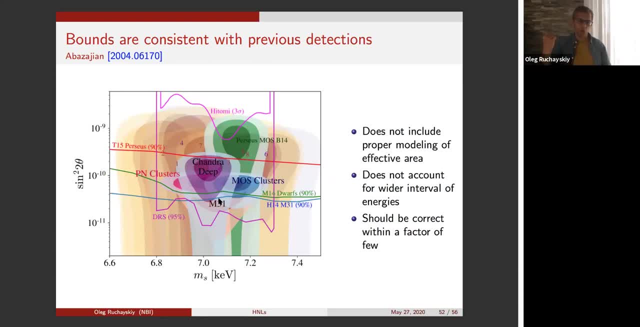 it will take a factor of few, having to do with the fact that you need somehow to account for the correct documentary abundance and so on. So, regardless of what you read about recent stats, 3.5 KV line- I believe that this line is there. 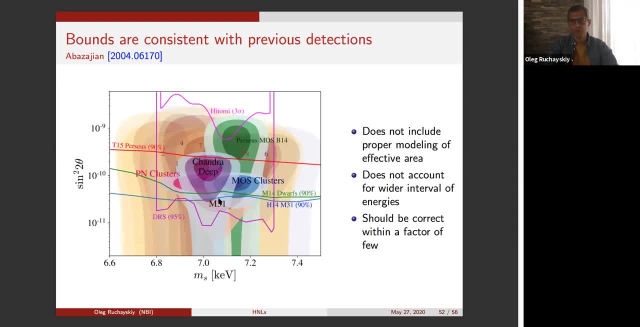 I see a strong line. I see this line behaving as document density profile predicts. Of course, it's always challenging to explain why other people got different results and that may indicate some flow in our analysis, but we don't understand where it is. 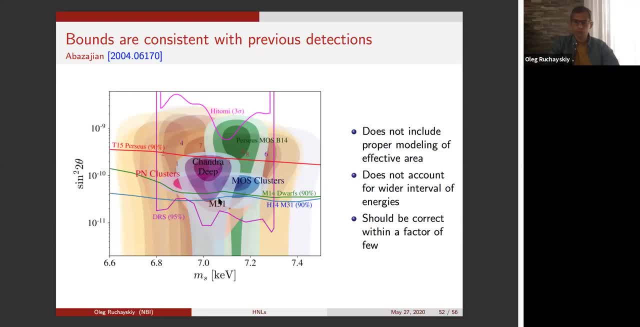 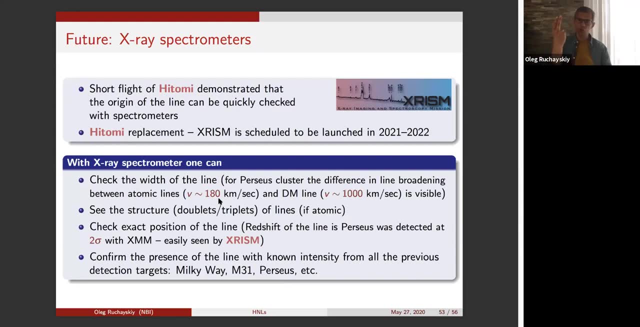 and maybe also flow in their analysis. So that's the status for now And of course, only the future will tell. At some moment, the satellites which can resolve this line and not mix it with nearby astrophysical lines will fly. 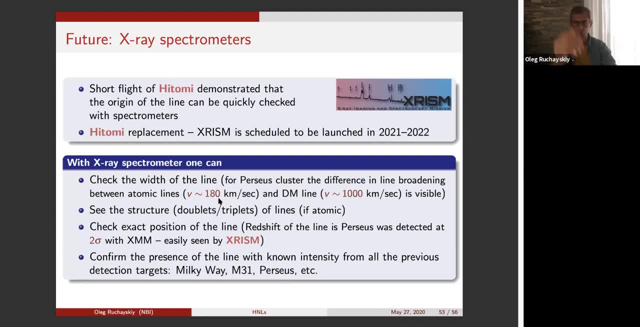 like this poor Hitomi, which will be replaced in 2021-2022.. And then we will finally know the truth. And if it is a documental line, then the cosmology of the 2020s will be completely different, because we will start to do. 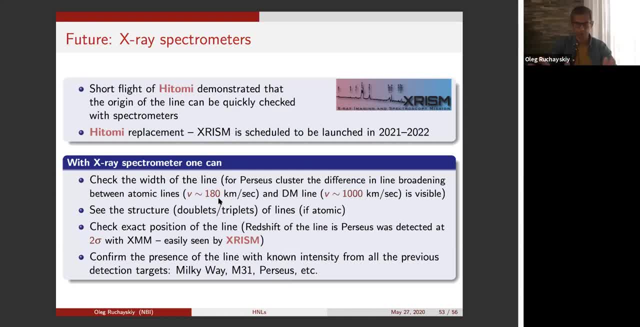 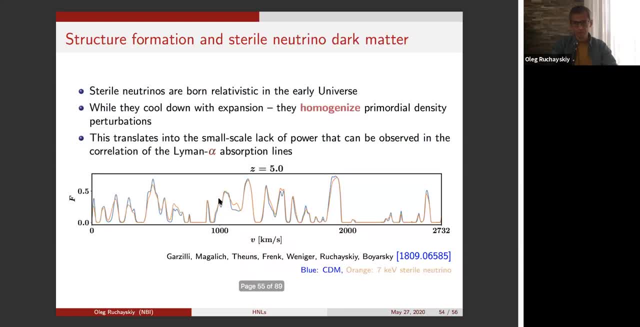 the documental astronomy, and that's where the tomography will be very exciting. I will need to finish in a couple of minutes, so one last thing, Because your documental particles are light, they are relativistic. in the early universe, They move around. 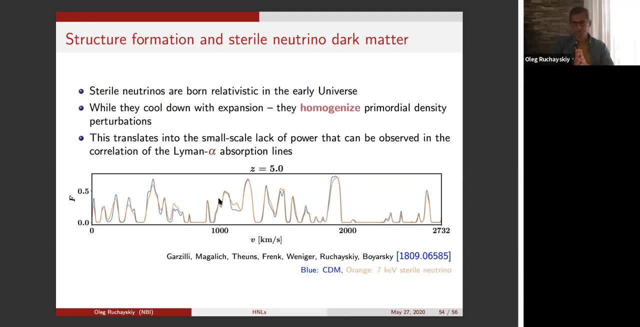 and they smooth the primordial in homogeneity, And so at small scales you should see the less structures in sterile neutrino documentary universe than in the core documentary universe, Which means that in the Lyman-Alpha forest your absorption spectra has less features. 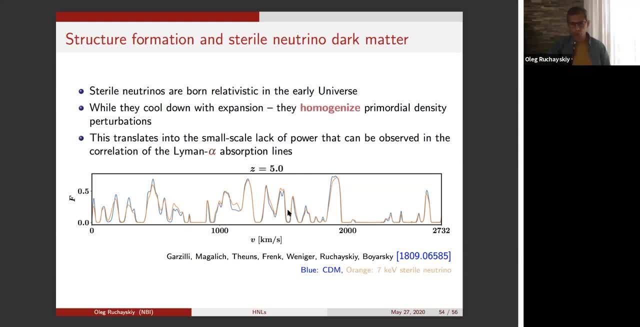 It's a small difference, like between the orange and blue, So blue have slightly more features than orange. You can understand that orange is a light smoothing of blue on this plot, But this difference is small And if you look at the modern data of Lyman-Alpha forest, 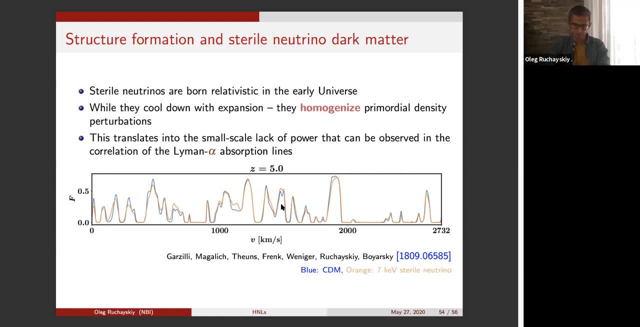 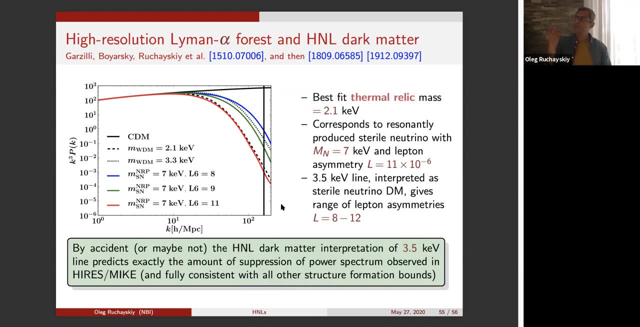 and I can speak more about this in the question section. then you see that actually- and this is completely by accident, because there is no a priori reason why the 3.5 kV line should have a correct clustering property. that's independent. 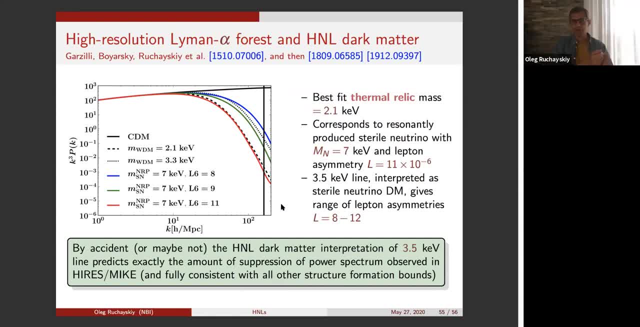 Only within the sterile neutrino documentary model. these things are related. It turns out that the same sterile neutrino documentary model, which feeds 3.5 kV signal, also is the best fit for the Lyman-Alpha forest data. It may be accidental. there are things to. 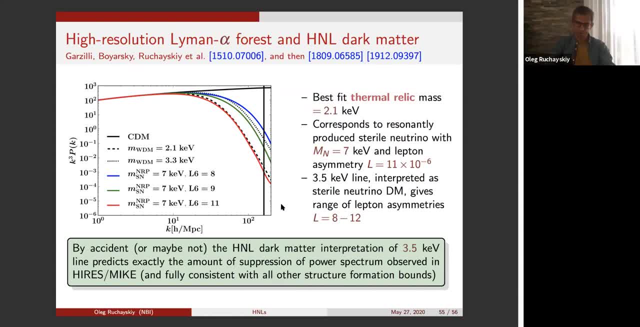 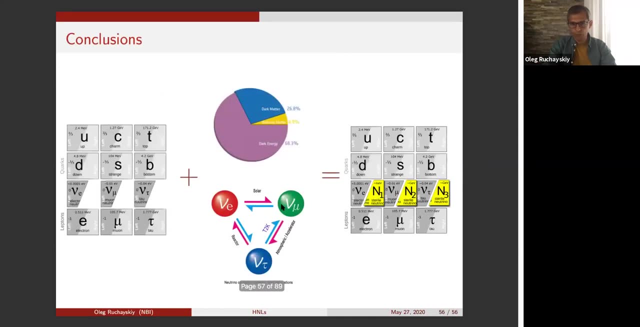 discuss here, but of course it keeps your spirits up. Okay, we started five minutes after the hour so I should finish, probably. So I promised for you to build a unified model of particle physics and cosmology, And more or less. 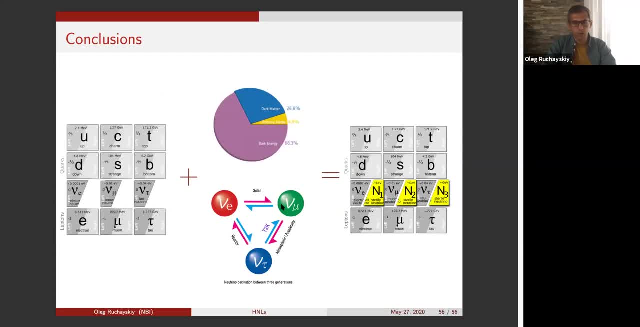 in my view this is the model, Standard model, plus three right-handed neutrinos. It can incorporate for you neutrino oscillations, duck matter, origin of baryonic matter. It can be testable at cosmic frontiers, at particle physics frontiers. 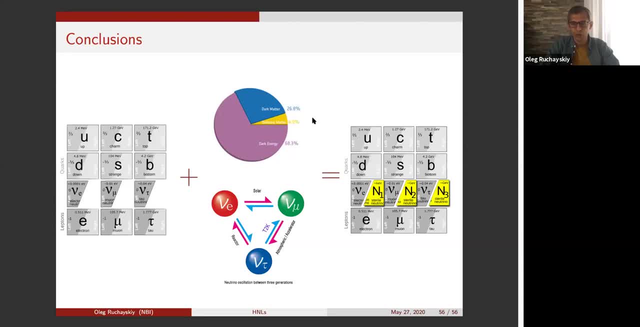 That's why I like it and work on it. So thank you for your attention. Well, thank you for the presentation. It's a lot of information, interesting and mind-boggling. So, anyway, this is the time we. 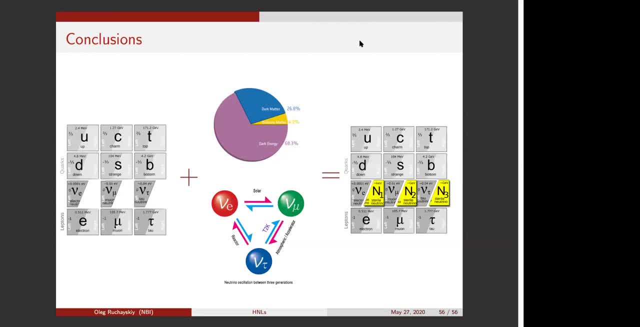 could go to questions. So if anybody in the audience has questions, please raise your hand in the participant section or let me know in the chat While people are thinking about their questions. I was actually wondering myself about one thing concerning the SHIP experiment. 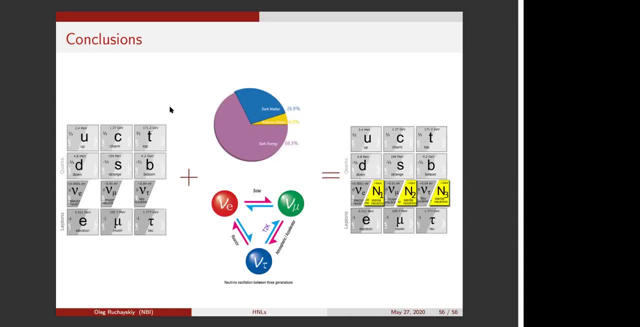 So what is the current status of that, if it's in the progress of being built, or what's happening? Well, as you understood, SHIP, if built, would be an experiment built in CERN, It would be experiments sitting on the 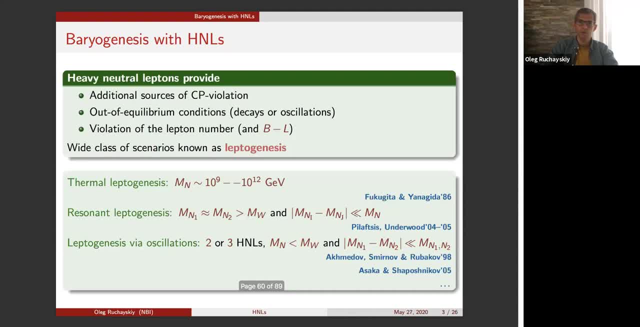 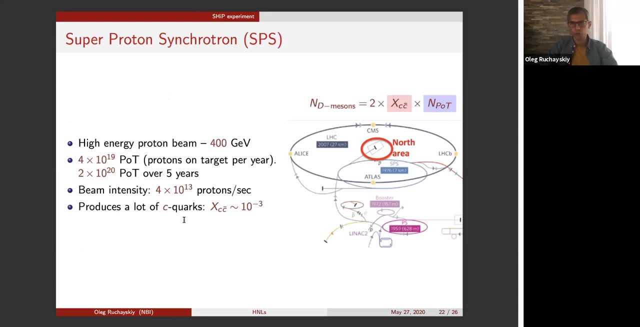 Yeah, so there is a in terms. there is a super proton, one of the previous generations experiments, and it accelerates proton to 400 GeV before they are injected to the LHC ring, And most of these protons are not used by the LHC. 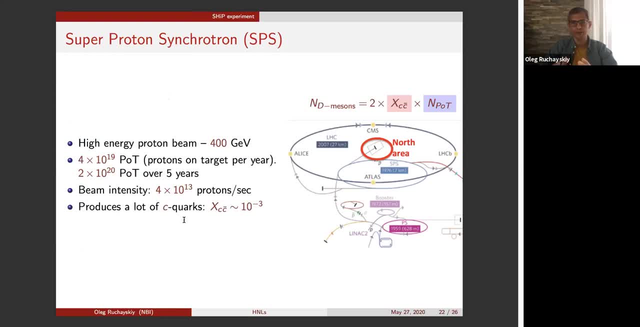 However, the intensity- not their energy, but their intensity- is enormous. It's highest intensity, highest energy intensity beam in the world, And so such an experiment would need to be built in CERN, and this experiment needs to be included into the European. 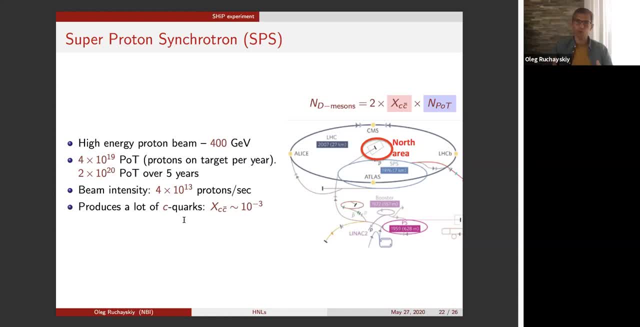 particle physics strategy update, which is going on right now. It has not been done yet, And if the strategy update will say that, okay, such experiments should be built, then CERN management will let us to go forward. So there are certain stages. 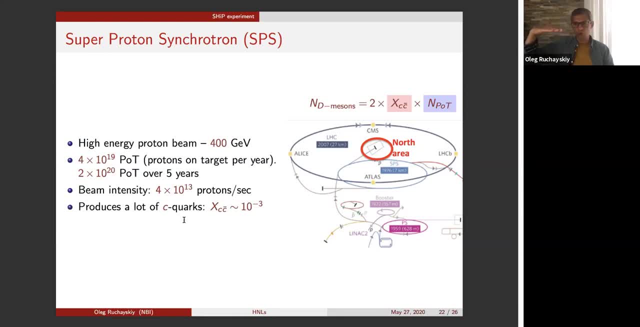 of preparing the experiment. We have completed all the stages which we can do now and we are waiting for the CERN management to give or not to give us approval to move on to the next stage to them, to the so-called TDR Technical Design Report. 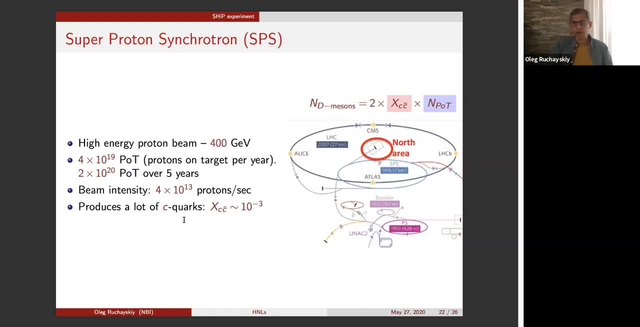 stage, In which case, if this happens around 2026, the experiment could start. So we think, if approved- but of course experiment of such level is not approved by CERN at all- It should be approved by a larger scientific community. 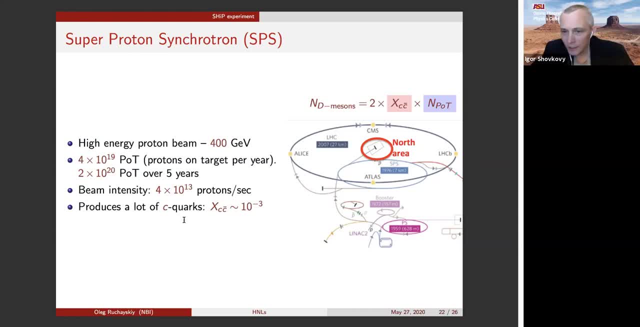 Awesome. Okay, Any other questions from the audience? I don't want to hijack this all by myself, Although I do have plenty of questions that I could ask if needed. I don't see any raised hands. Either, everybody is still sleepy Already. 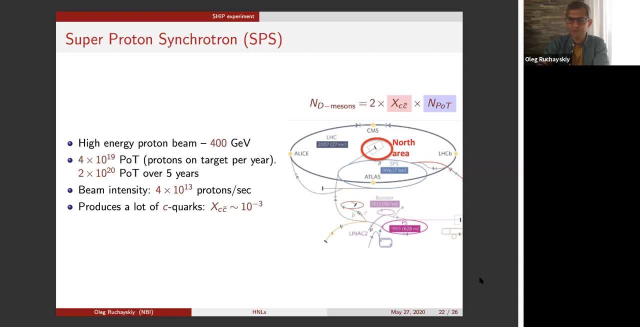 sleepy. Okay, Go ahead, Tanmay, Tanmay, go ahead. You have to unmute yourself. Hi, Oleg, Nice talk. Thanks, I might have missed it because I was having some internet problems. Could you say something about? 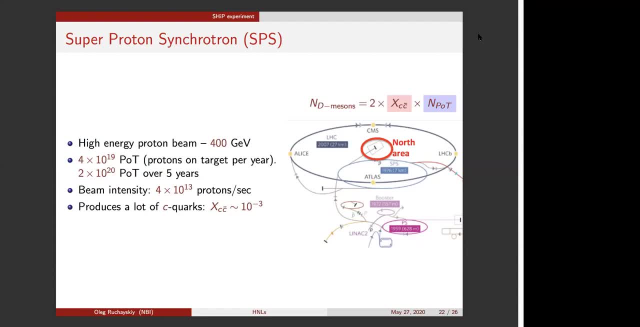 leptogenesis that you're doing. Yes, So there are these kind of HNLs. They are light. Therefore they cannot produce lepton asymmetries in the usual way by just Cp-violating decays as heavy HNLs. 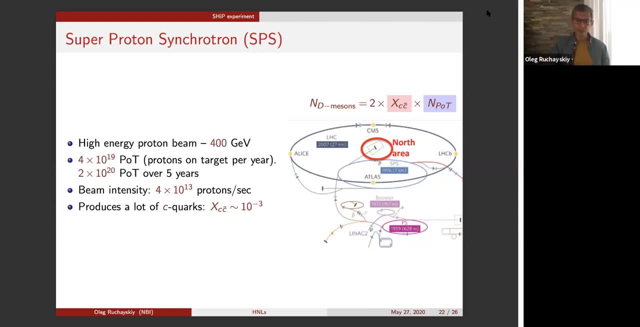 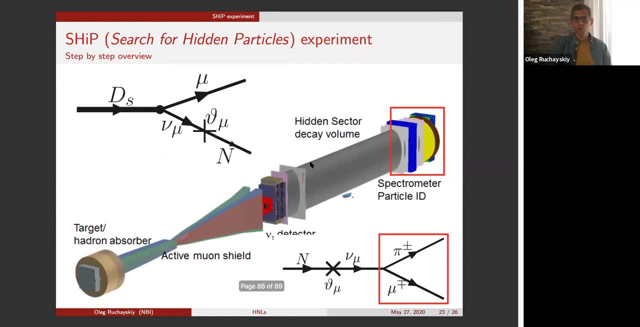 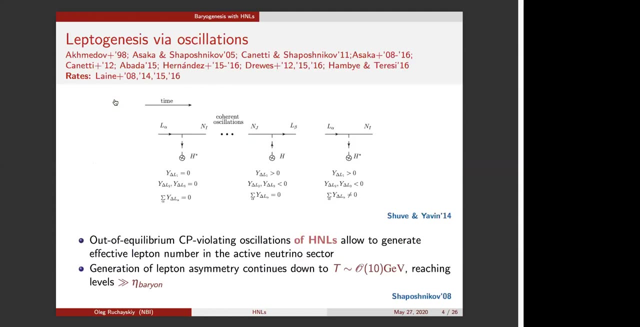 could do. Your Yukavas are too small. What they do? they do so-called retogenesis through oscillations, which works in the following way. Let me have a slide here. So you produce an HNL, you produce a lepton, it produces. 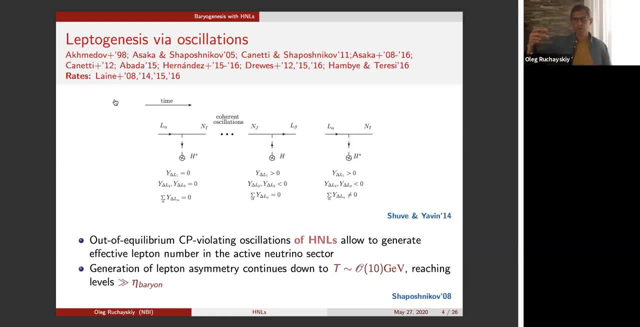 an HNL. HNL flies and oscillates and can produce another lepton. In this way, you violate lepton number, lepton flavor number, but don't violate the total lepton number, However, because your oscillations are actually Cp-violating. 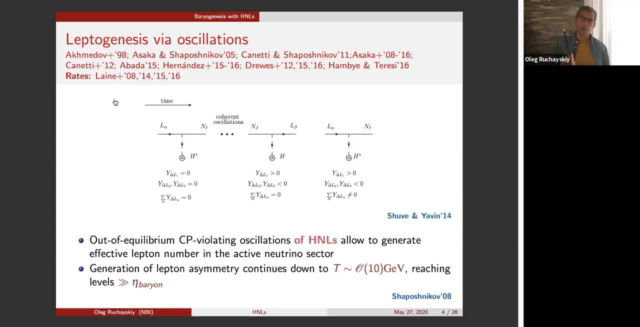 they can be Cp-violating. That's a requirement for this numism model to be a retogenesis model. In this case you can also produce total lepton number. So you produce a particle, you oscillate, produce another particle. 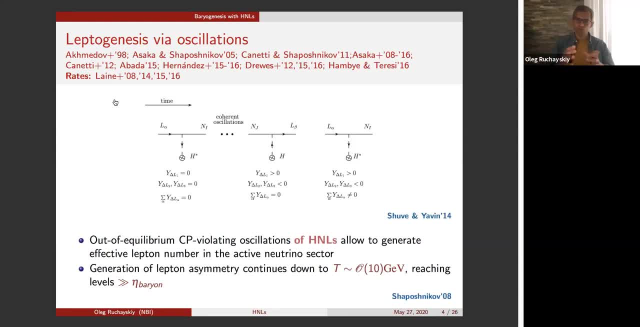 Which is actually an antiparticle. In this way you violate the lepton number and you generate it. It builds up Svalerons, convert into the baryonic symmetry usual story And in this way you can produce a baryonic symmetry of the universe. 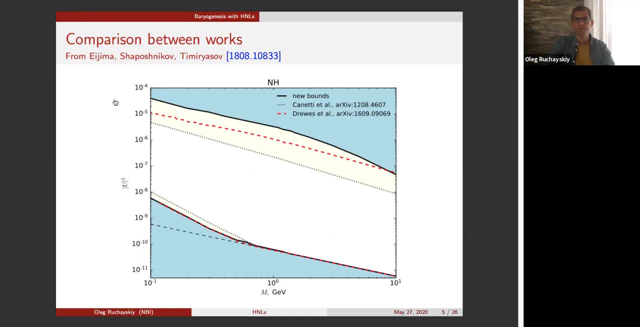 in a very wide range of mixing angles. If your coupling constant is too high, like here, then you enter equilibrium before the Svalerons freeze out and you give back all the baryonic symmetry you produced. If your coupling constant is too small. 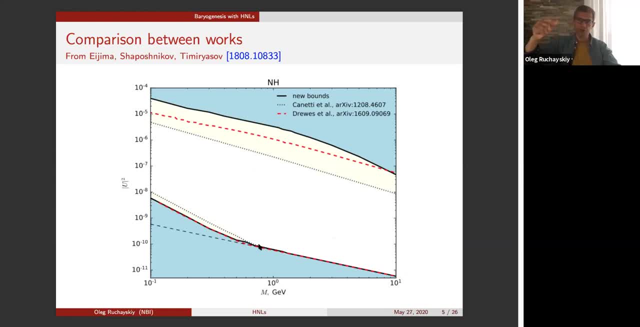 I mean you're still proportional to the Yukawa's, although with some enhancement from the resonant oscillations. then you just don't produce enough. But there is a several orders of magnitude wide region where you can produce enough. baryonic symmetry of the universe. 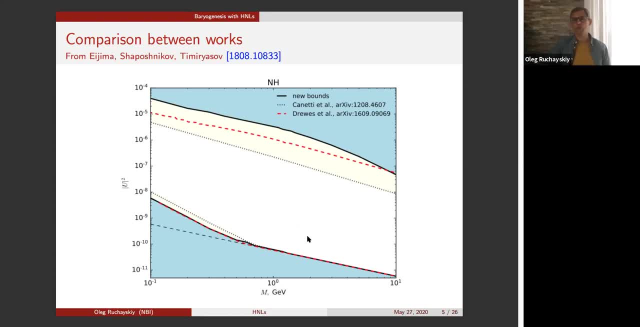 given some other parameters which are not constrained by experiments or by neutrino data. Alright, thank you. Okay, Any other questions? Okay, I don't see any other new hands. So well, for the sake of it, since nobody's interested. 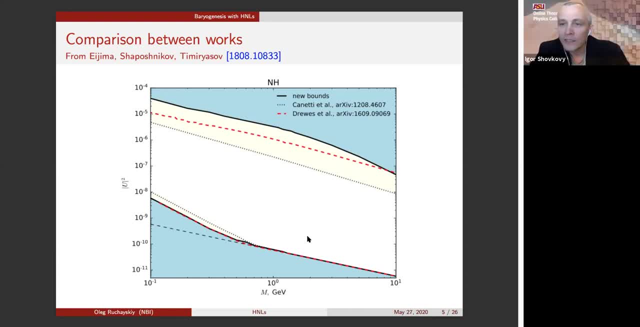 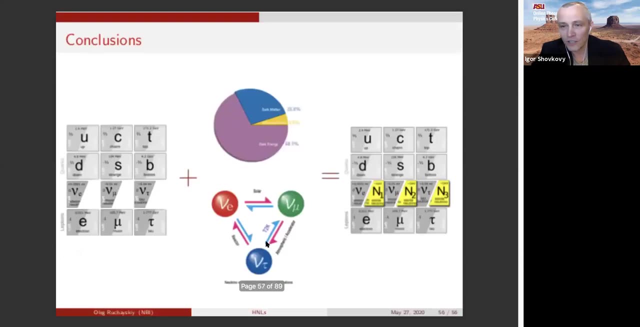 I am In these models with the sterile neutrinos. well, this is like one of the models that is to replace the previously thought supersymmetric models to work and they apparently there is no trace of them, So sort of it's a two-sided question. Is there any? 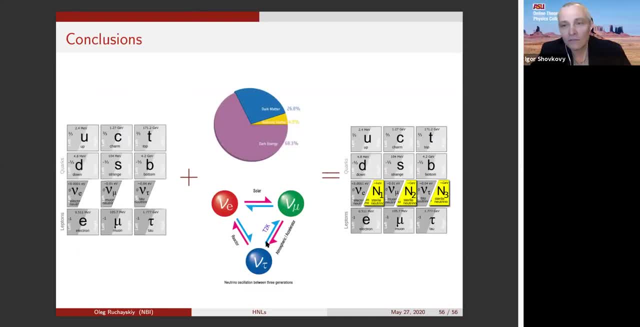 connection to the potential supersymmetry? And, of course, if not, then the next natural question is: is there some sort of natural unification? like the supersymmetry was praised for the ability to unify couplings, to unify everything, and maybe 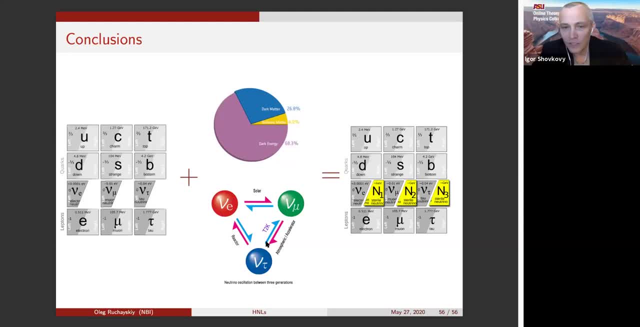 reduce or remove the hierarchy problem. Is there something like that with this sterile neutrinos? Okay, So several things here. First, in this model, the top is the heaviest particle, and then Higgs and then everything else. H and L are lighter than W. 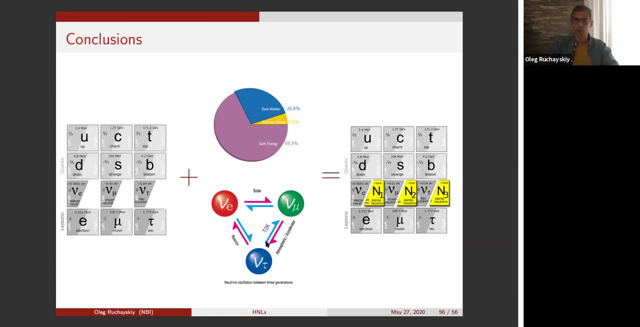 So in this model there is no Higgs hierarchy problem because there are no heavy particles in the loop which give quantum corrections to the Higgs. So it's essentially your effective potential, is the effective potential of the standard model which people have computed. 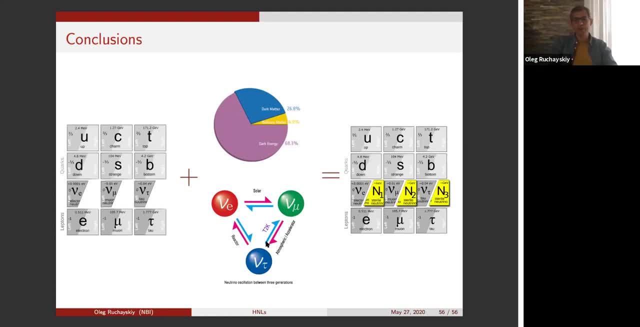 and know how it runs, Or says there is no hierarchy problem here. The question you may ask here is the question like: why is gravity 10 to the 19 JV Planck scale and you see the scale of 100 JV, but that's a different story. 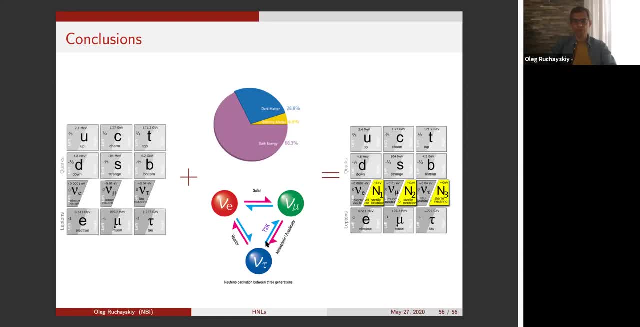 There are some answers to this question outside the scope of this talk. Now, supersymmetry I mean of course you can supersymmetry on MSM, but there is no reason for that. It doesn't do you any good and 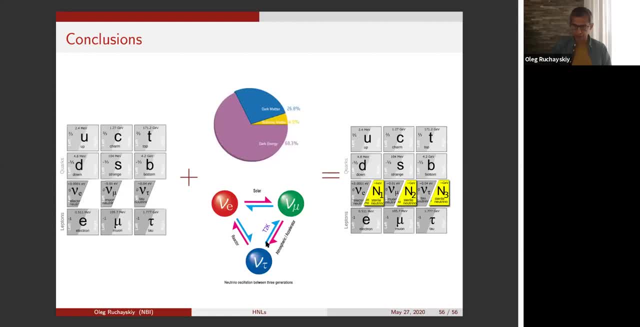 as you probably know, when you deal with supersymmetry, yes, it buys you something, but it also needs to be very careful, because a generic supersymmetric model would be ruled out by observations many, many long time ago. right, You need very specific coordinates of the 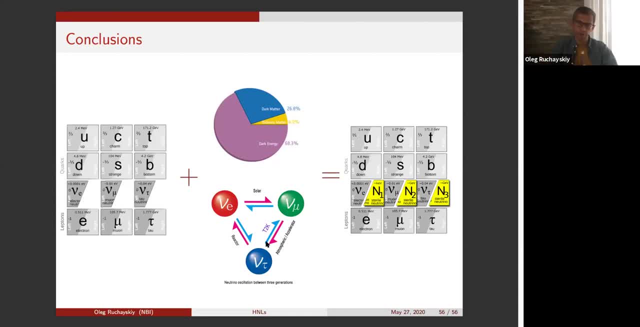 big parameter space of supersymmetric models to be consistent with the data flavor and so on. So here again, it doesn't give you any benefits because only some problems are solved, but it gives you troubles. I mean, of course, nature may be. 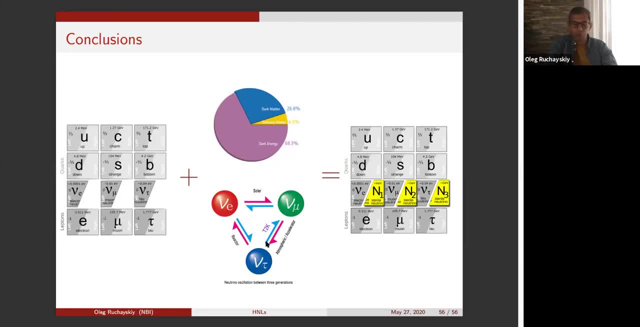 very ironic sarcastic here- ironic I don't know. but Well, I'm not to protect the supersymmetric model. I sort of like that was one of the driving forces for a while and I'm just trying to see what's replacing it. 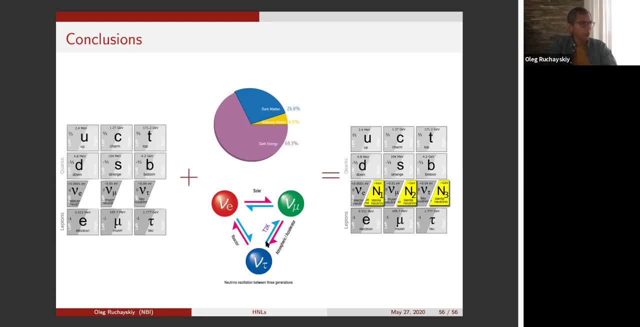 So for the ground unification, no, the coupling constant here run exactly as in the standard model, so they don't meet. Then the question is: what is UV completion of the CO? and it takes a little bit to decide this field. 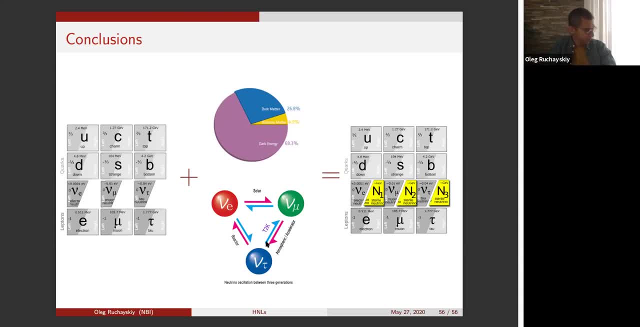 of kind of phenomenological physics in which I was sitting so far. In principle, you can organize ground unification in standard model-like theories if you allow yourself certain high-dimensional operators which are Planck-suppressed. Interesting thing, that Planck-suppressed, high-dimensional 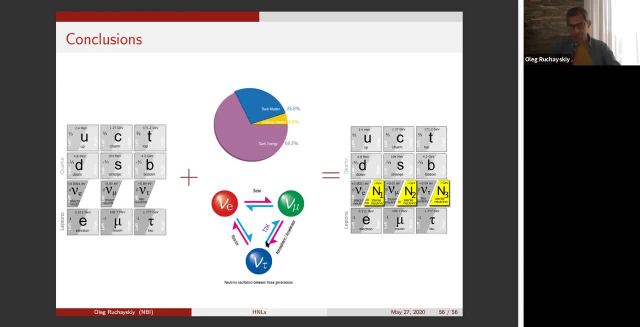 operators can organize for you the ground unification. And then the question is: why do you believe that Planck-suppressed is okay and not Planck-suppressed? I mean, we enter into the very kind of speculative realm and we can talk.